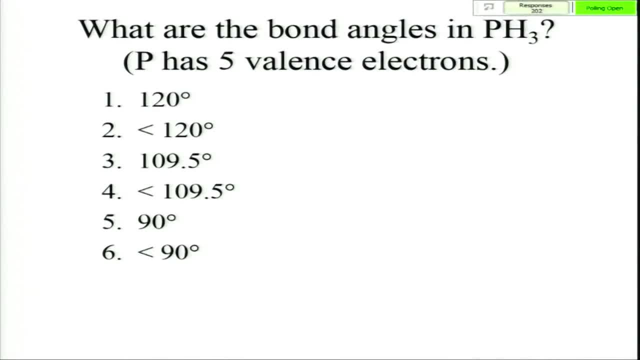 If you haven't clicked in yet, please pay attention to the clicker question and I'll give you a little bit more time to click in And I'll give you a 10-second warning. All right, let's just go ahead and take 10 more seconds. 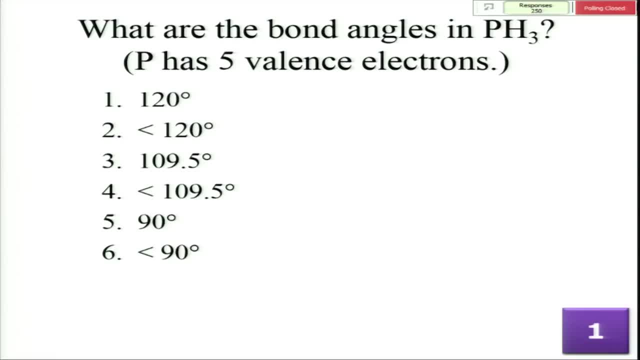 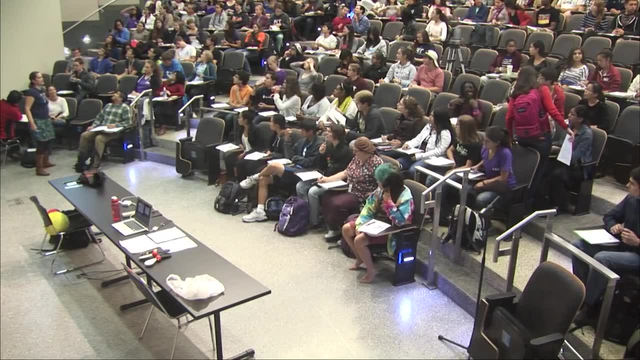 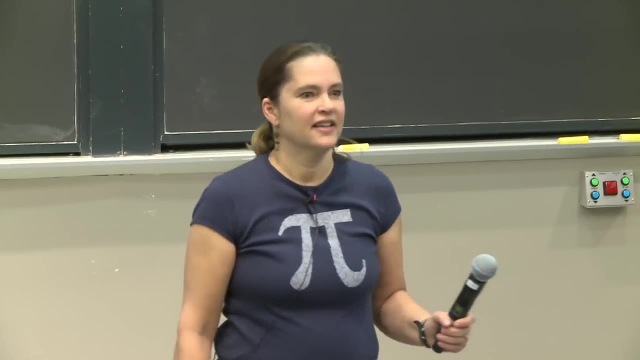 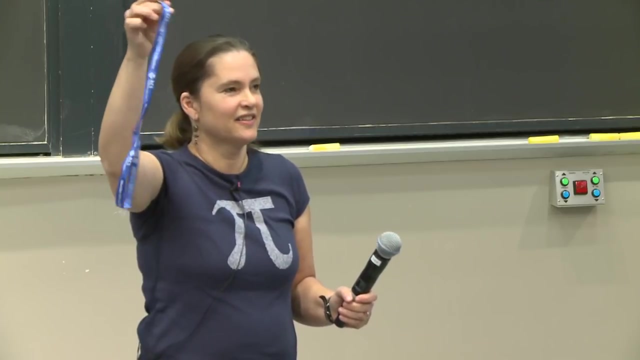 All right. does someone want to say how they got this one right? Anyone willing to say how they got it right? We have a American Chemical Society- whatever these are called- that hang around your neck and clip things to them. Yes, 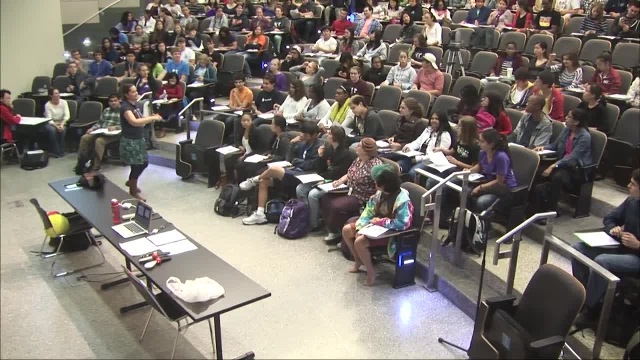 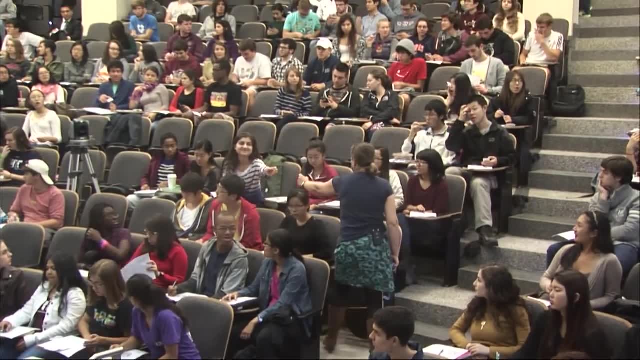 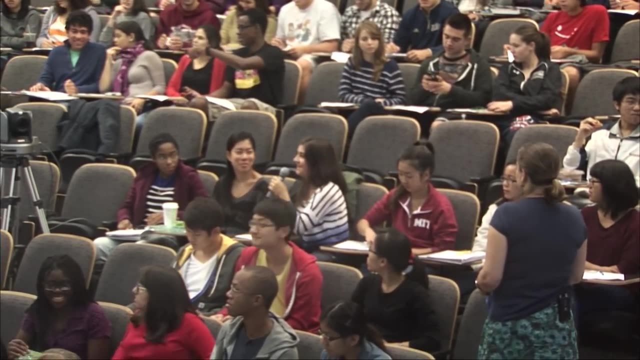 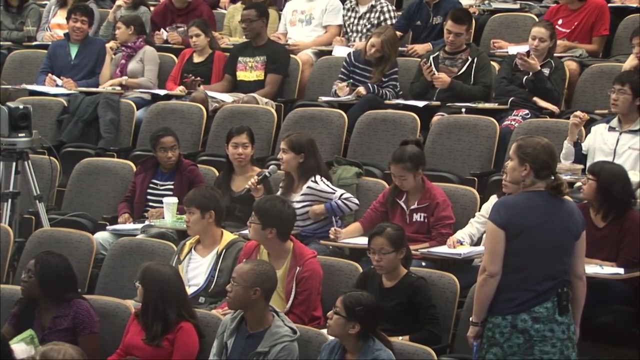 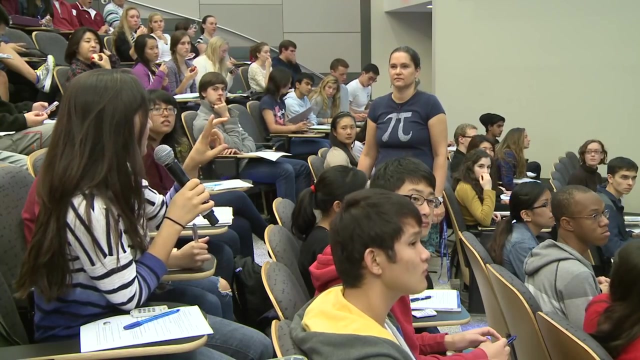 There's the word No. Oh, there we go. OK, so this molecule is, the phosphorus has five valence electrons and then each hydrogen has three, So it's for a total of eight. So it has three bonding And then one lone pair, which makes it a tetrahedral. 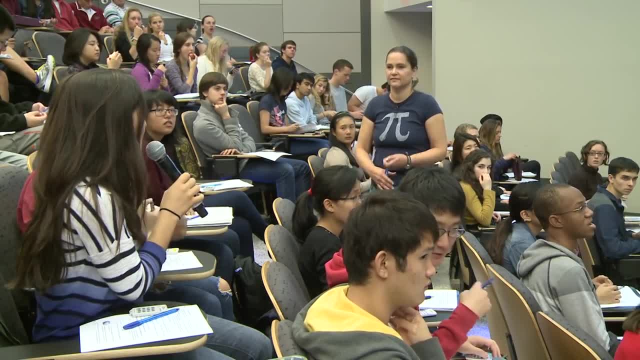 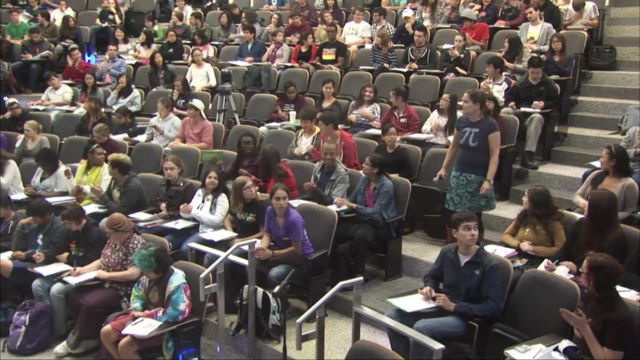 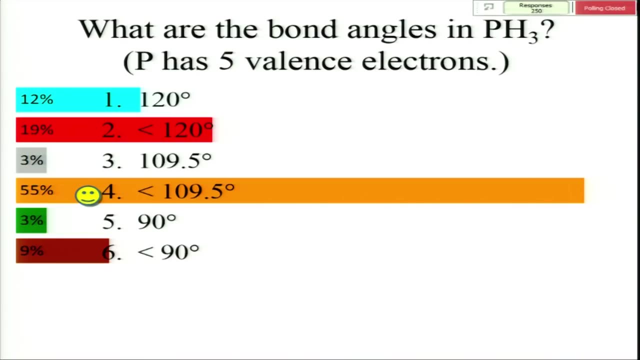 but then the lone pair pushed the other bond, so it's less than 109.5 degrees. Excellent, Yeah, So I see that some people just decided that there were three things bound to it, and so then they decided either 120 or less than 120.. 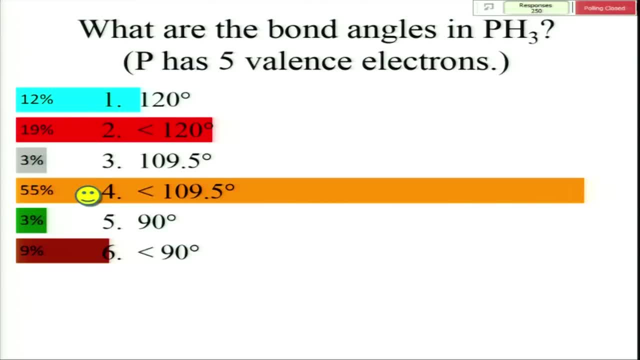 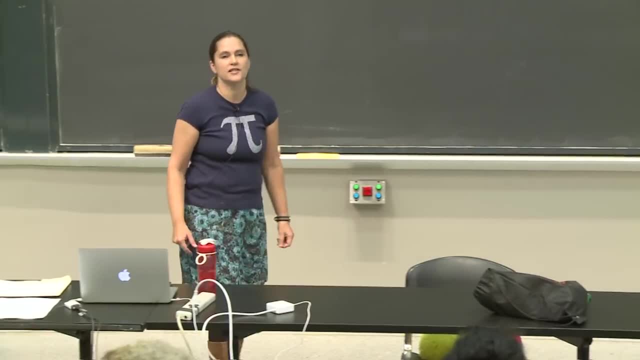 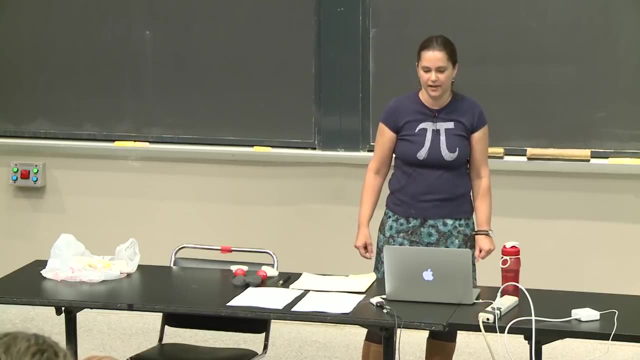 But you really need to do the Lewis structure and see and see how many lone pairs there are first. So once you do the Lewis structure, then you figure out the parent geometry, SN4 system or tetrahedral system. All right, so more practice on these coming up. 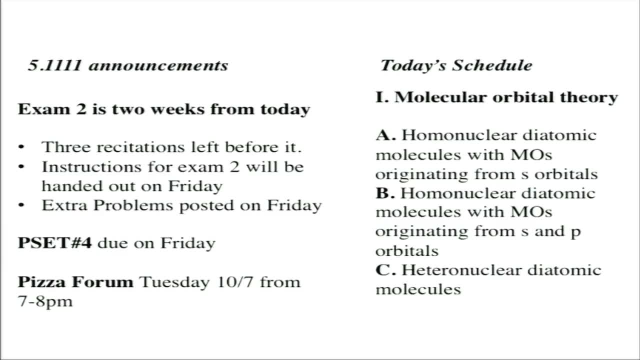 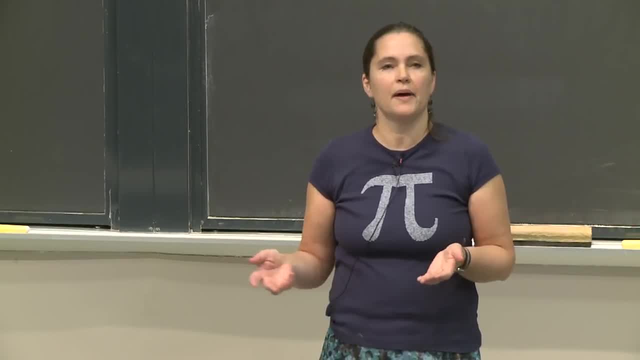 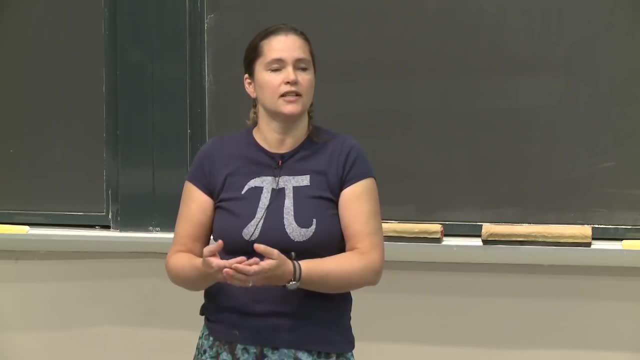 All right. so we're continuing on now with molecular orbital theory And we started the course talking about atomic structure and then we talked about atomic orbitals or wave functions, And then we moved on to bonding- that atoms can come together and bond and talked. 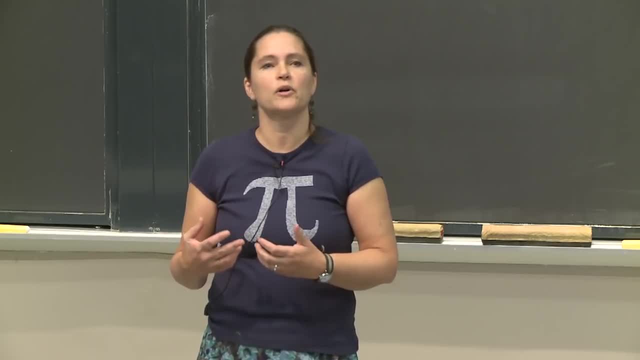 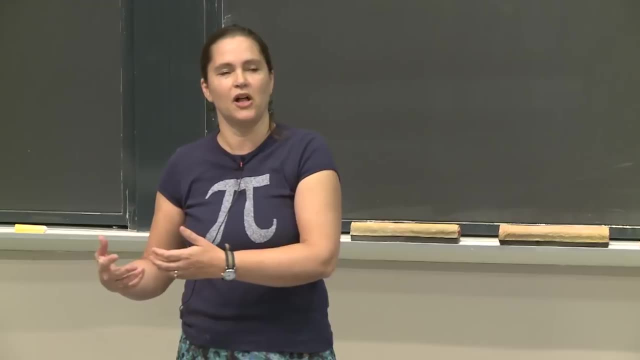 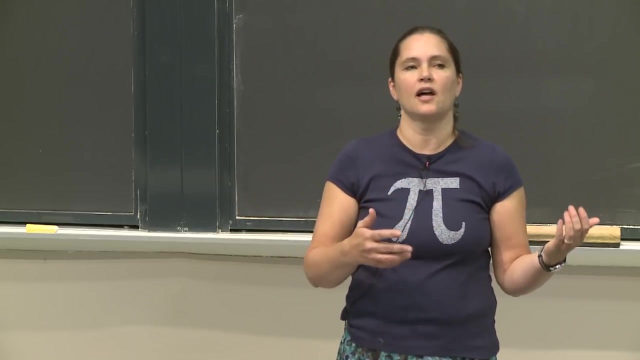 about the structure of molecules, And now we're going to molecular orbitals, And then we'll also talk more about the structure of molecules based on those molecular orbitals on Wednesday. So we're really coming all the way around. We're using a lot of the ideas that you've seen before. 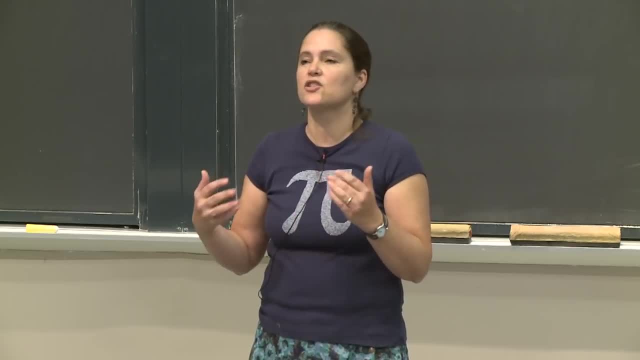 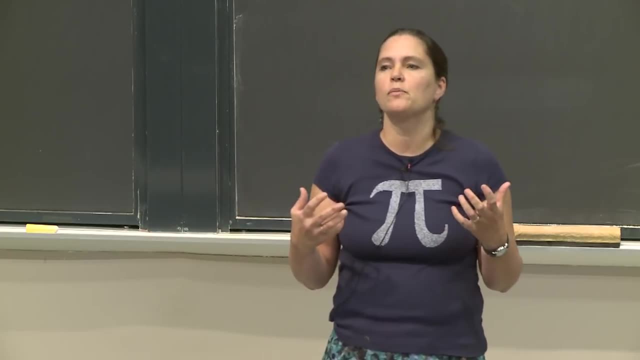 but now we're applying them to molecules And then to me this is really an exciting part. I love getting to know you. I love getting up to the molecules and talking about structures of molecules and how orbitals really play a role in those properties. 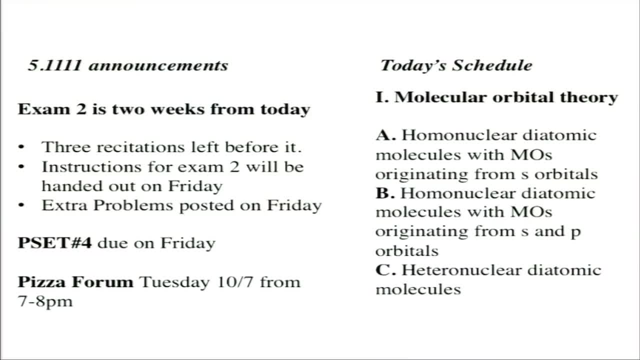 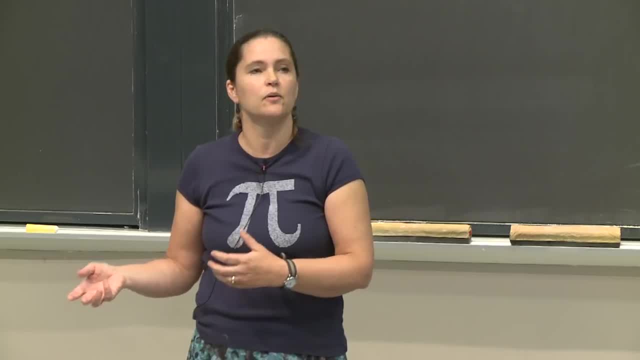 that molecules have. And then to me, the really exciting I like- reactions. So after we finish with the structures, we're going to talk more about how molecules react, And so on Friday we're going to be starting that- reactions of molecules and getting into thermodynamics. 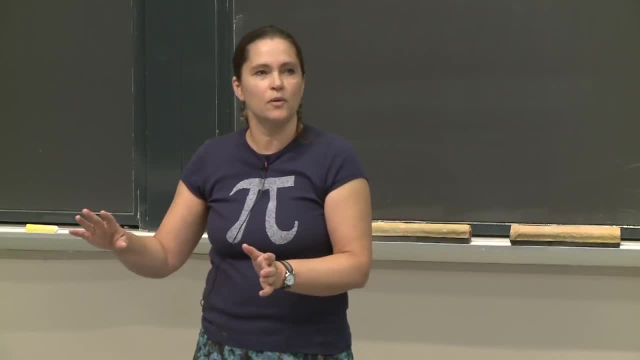 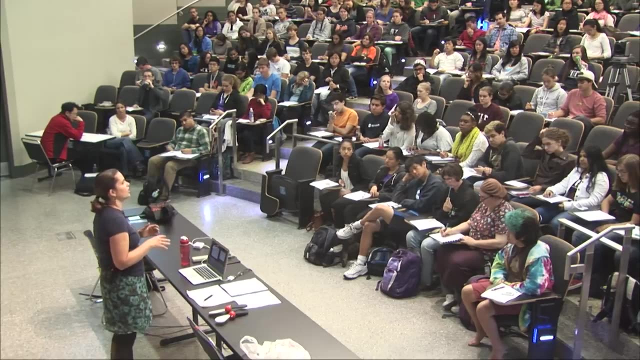 So we're sort of winding our way away from orbitals for a while. We will come back to d orbitals. We're going to talk a little bit more about that around Thanksgiving time, but we'll have a long time before that where we're talking about reactions. 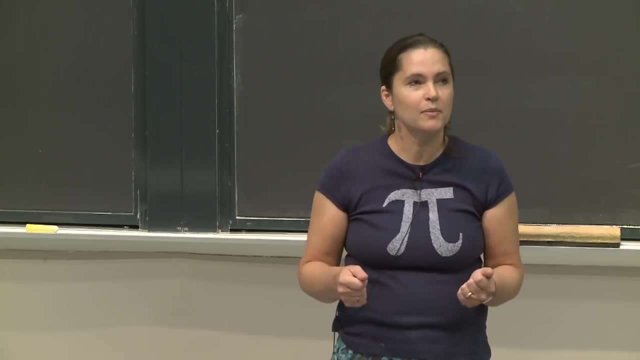 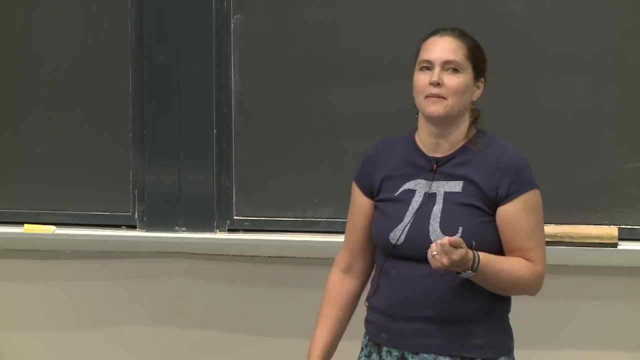 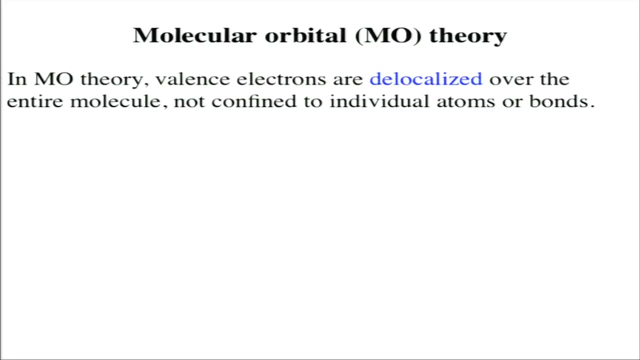 So we're about to kind of do a transition in the type of material, But before we do that, more orbitals. But these are super cool because these are molecular orbitals. So we're going to talk today about MO theory, MO for molecular orbitals. 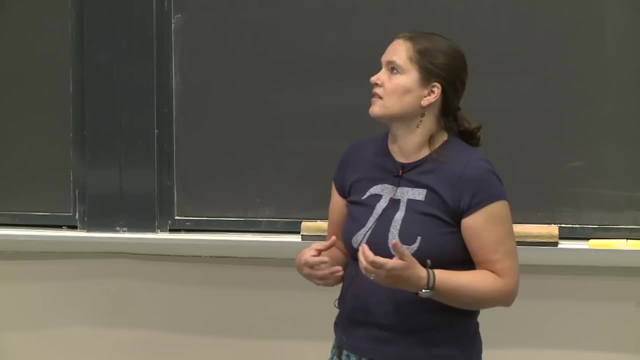 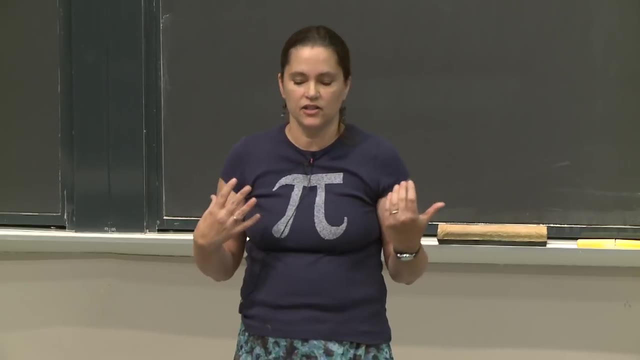 So molecular orbital theory presents the idea that these valence orbitals are going to react. These valence electrons are really going to be delocalized around these molecules and not just sitting on individual atoms. So to think about this electron delocalization, 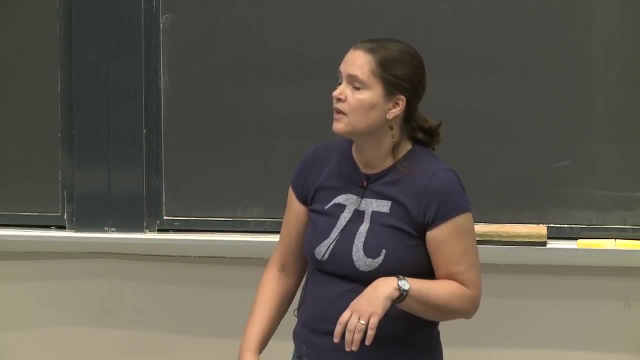 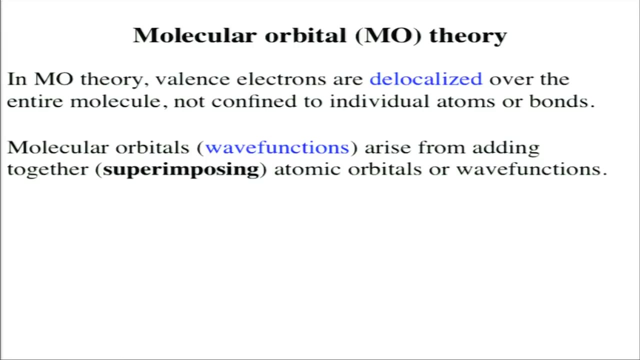 we need to think about molecular orbitals. Molecular orbitals, as we've learned another word for orbital- is also wave functions. Wave functions are orbitals. Orbitals are wave functions. You need to consider the wave-like properties of electrons to think about where. 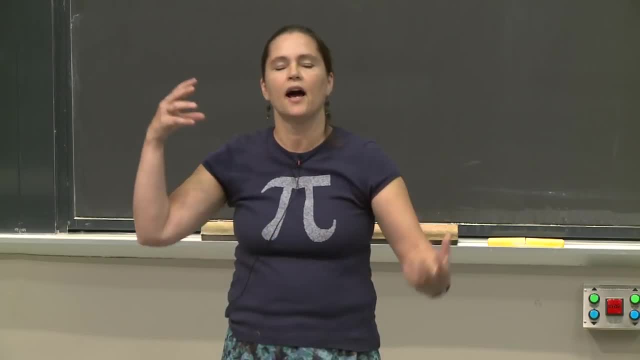 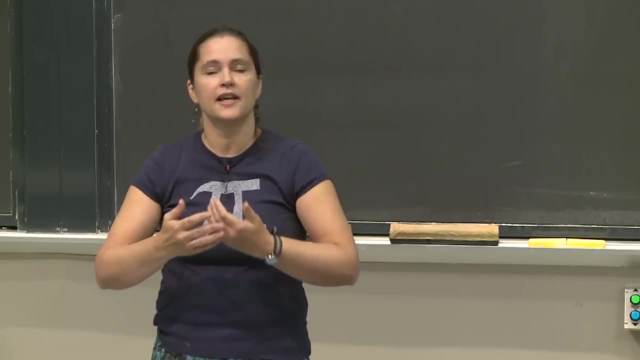 the electrons are going to be? What is their probability density? How are they going to be arranged with respect to the nucleus? And so we take atomic orbitals and we bring them together. As atoms come together to form bonds, atomic orbitals come together to form molecular orbitals. 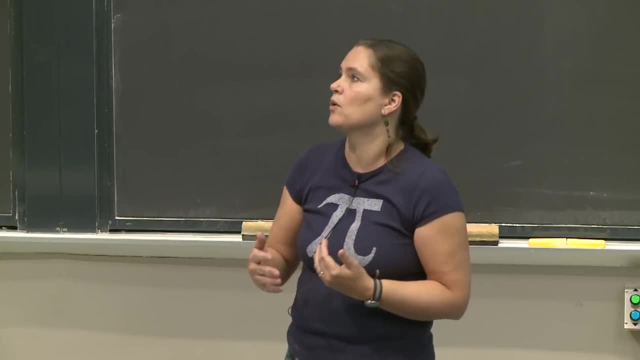 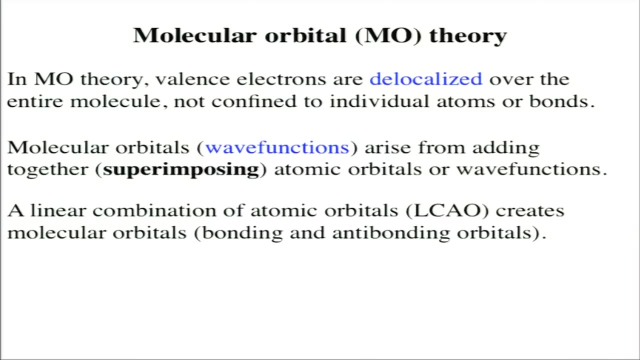 So we're going to be adding superimposing atomic orbitals to form these molecular orbitals, And this is called a linear combination of atomic orbitals or LCAL, And so we're going to bring those atomic orbitals together and create molecular orbitals. 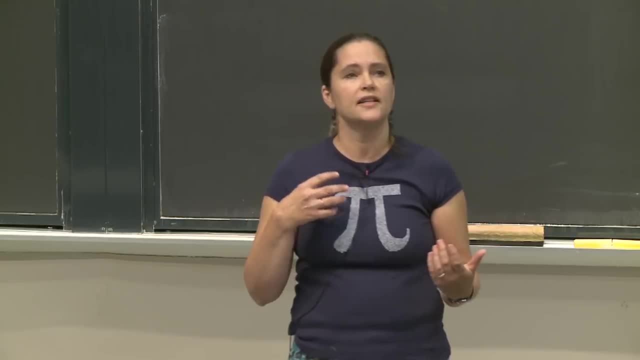 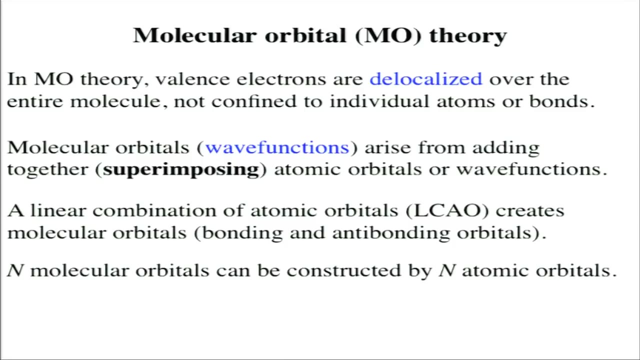 And we're going to create two types of molecular orbitals. We're going to create bonding and antibonding, And some basic math principles apply here, And that is that you can create n molecular orbitals from n atomic orbitals. So that's really the basis of molecular orbitals. 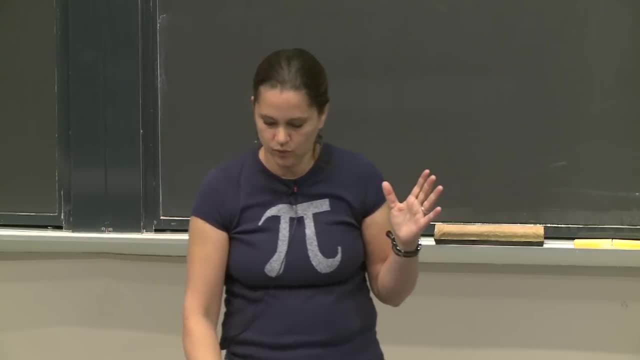 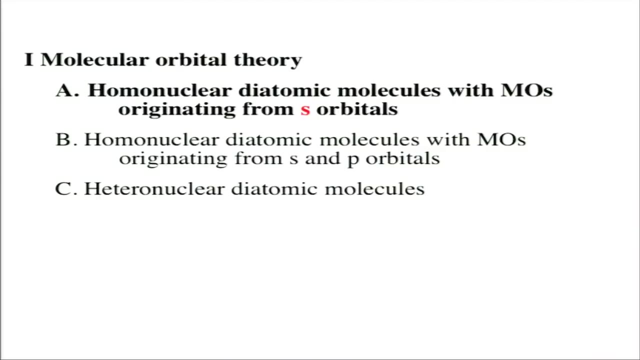 And then we're going to go back to our orbital theory, And now let's apply it to our friends the s orbitals. All right, So we're going to think about really simple molecules, bringing together two atoms that are identical with each other. 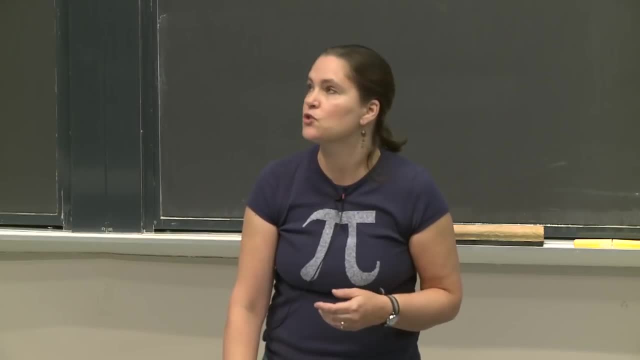 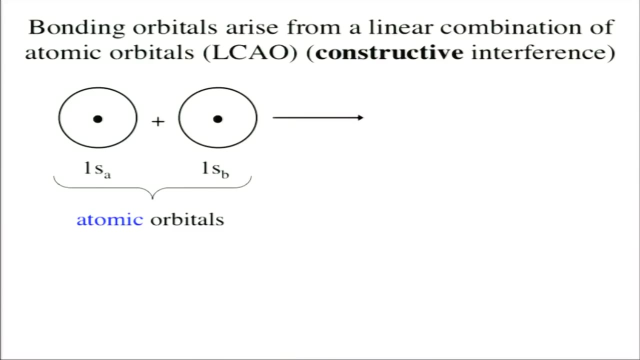 and what happens to their s orbitals when this happens. So first we'll talk about bonding orbitals. So bonding orbitals again arise from this linear combination of atomic orbitals, the LCAO, And bonding orbital. it's going to arise. 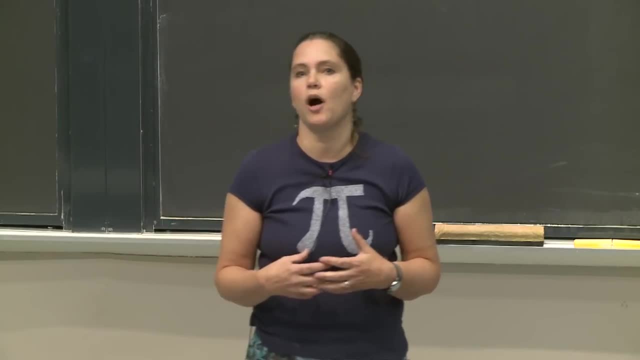 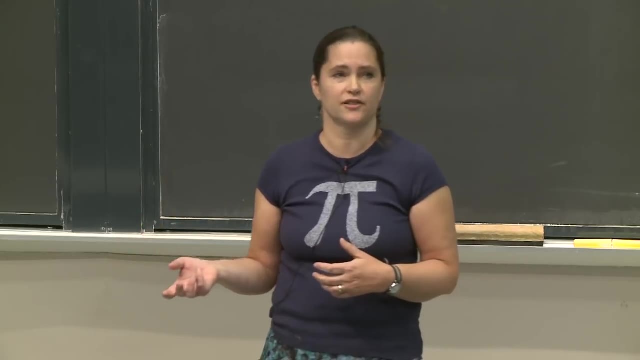 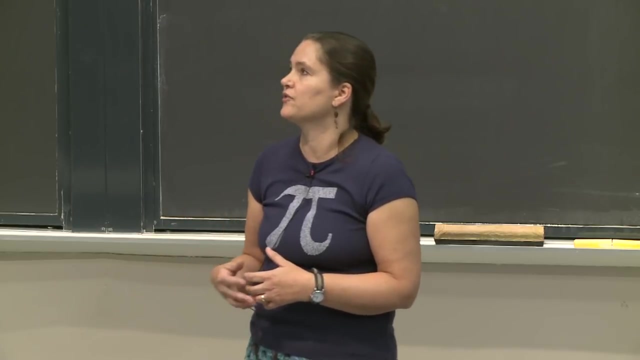 from constructive interference. So we talked before about the properties of waves, And one of the great properties of waves is that they can constructively interfere or destructively interfere, And orbitals are wave functions, so they can constructively interfere and destructively interfere. 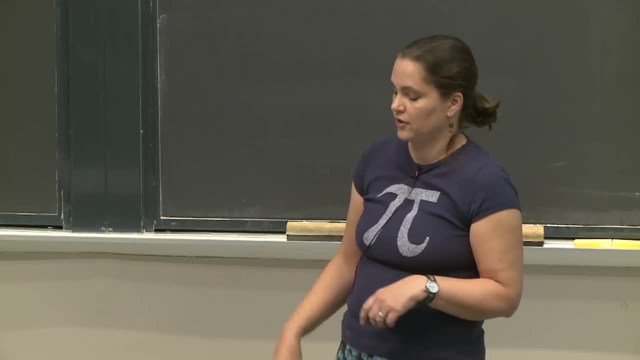 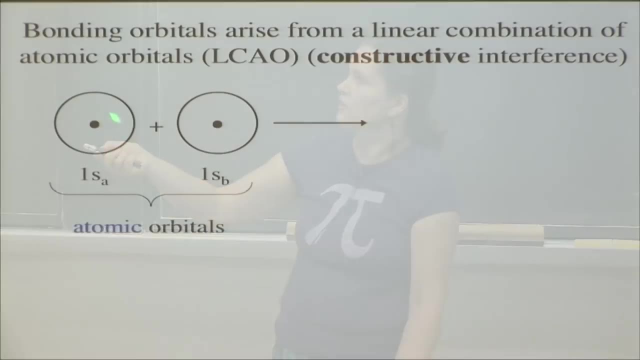 Bonding orbitals are generated by the constructive interference. So let's look at two atomic orbitals, And so here we have an orbital, The nucleus. It's in the middle, It's a little dot, It's a nucleus, And these two atomic orbitals are going to come together. 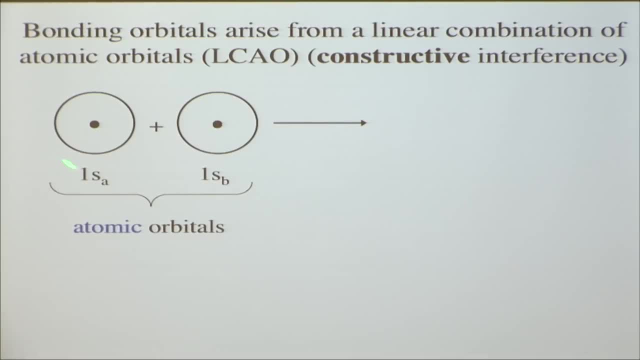 There's going to be a bonding event And so we have a 1s orbital from atom A and a 1s orbital from atom B And they're going to come together And they're going to form a molecular orbital, an AB molecular orbital. 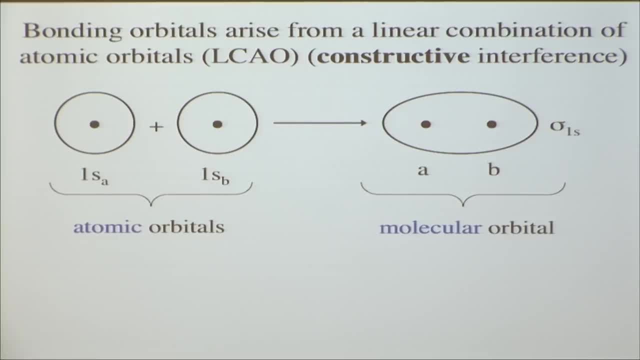 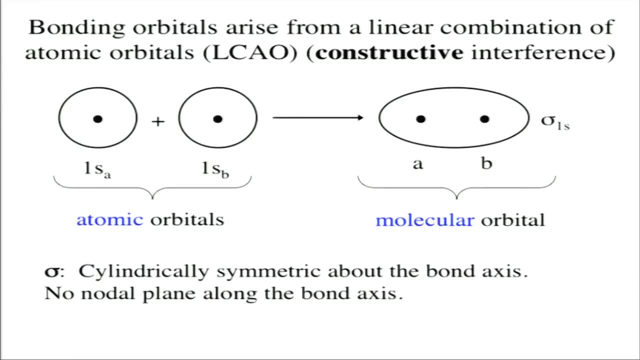 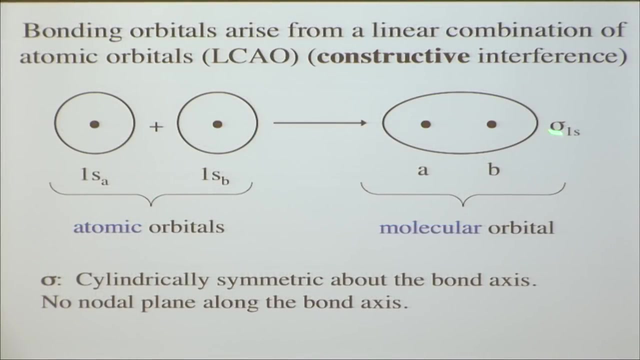 And this is called sigma 1s. So a sigma orbital is symmetric. It's symmetric around the bond axis. So the bond axis here would be just a vertical a line between these two nuclei here, And so this molecular orbital is symmetric around that bond axis. 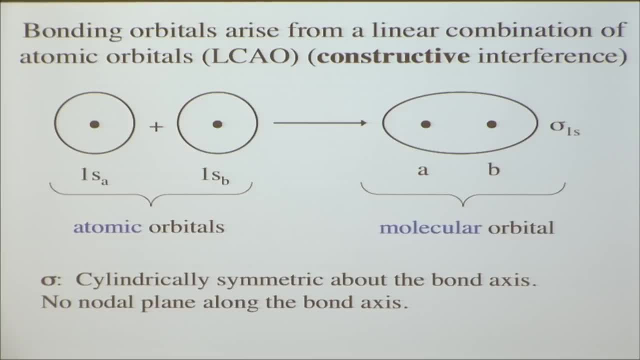 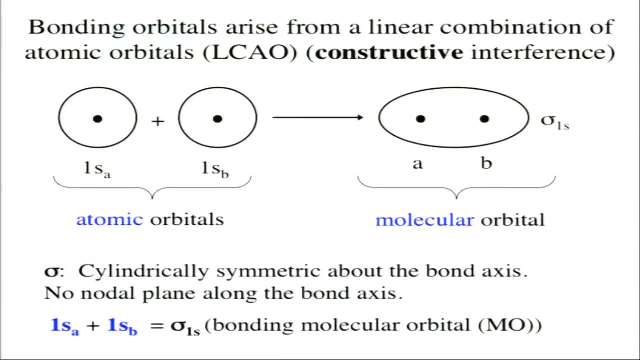 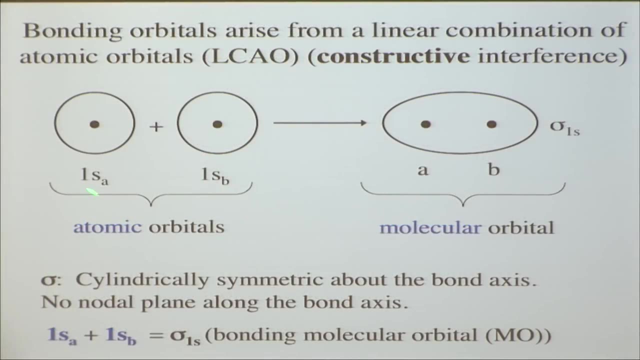 There are no nodal planes for something that is symmetric. There are no nodal planes for our s orbitals, And so there's none for the molecular orbital either, And we can also write this as 1sa plus 1sb, So the atomic orbital from 1sa, the atomic orbital 1sb. 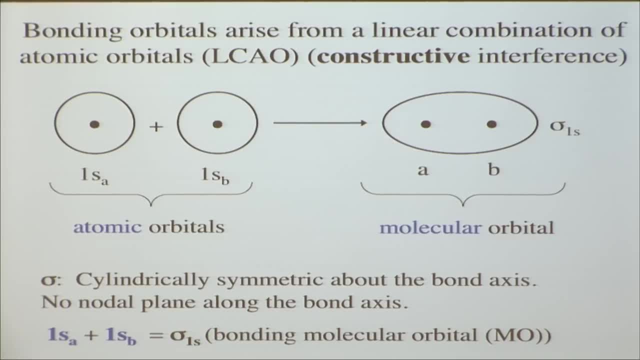 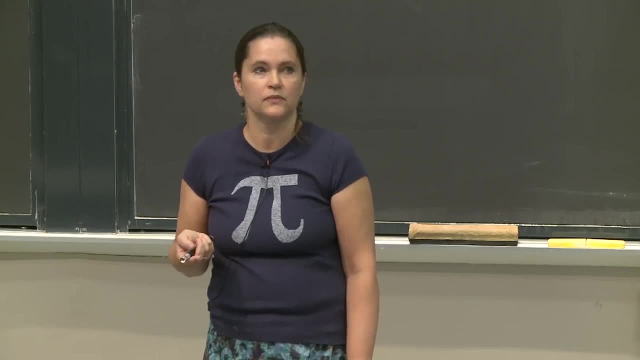 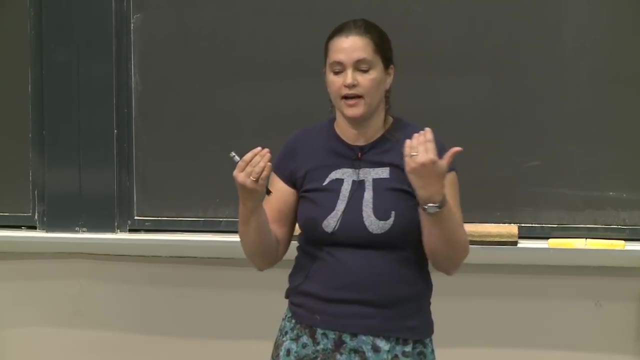 coming together to form sigma orbital 1s. That is a bonding orbital because it's constructive interference. It's a bonding MO or molecular orbital. So now let's consider the wave-like properties And think about these atomic orbitals coming together and what is happening. 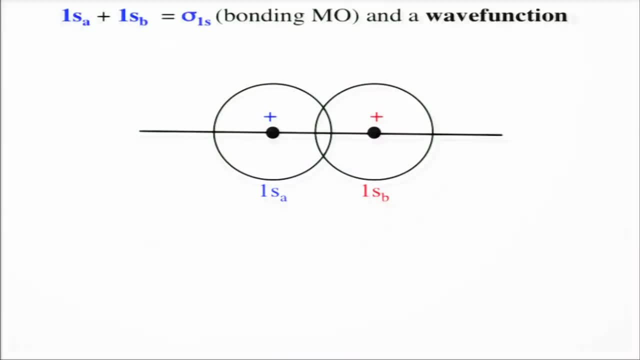 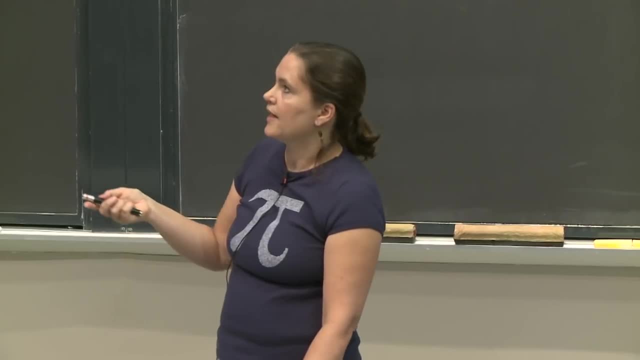 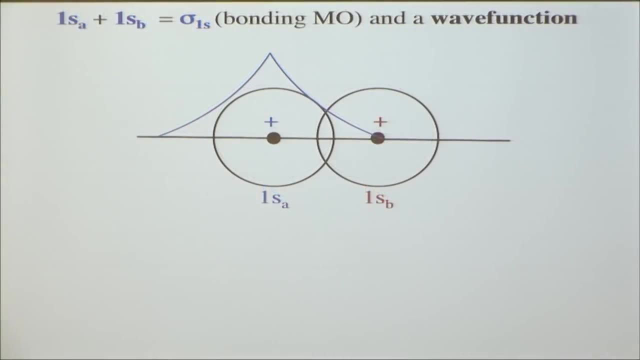 So here we have the same equation. up here We're bringing together 1sa and 1sb, But now let's think about this as a wave function. So there is an amplitude associated with the wave function for 1sa And there is an amplitude associated with the wave. 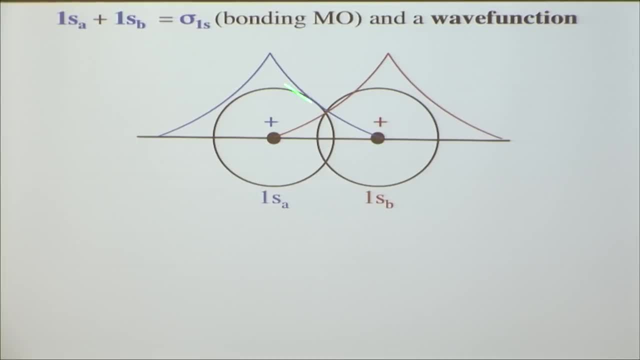 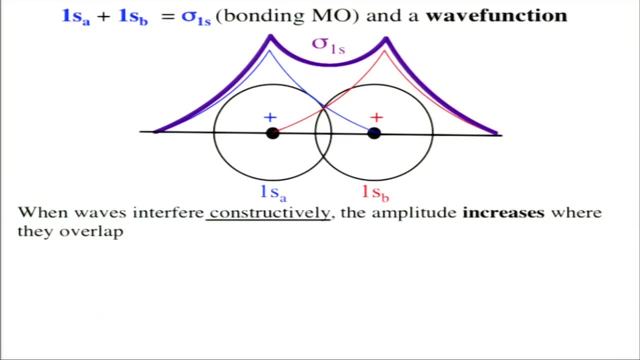 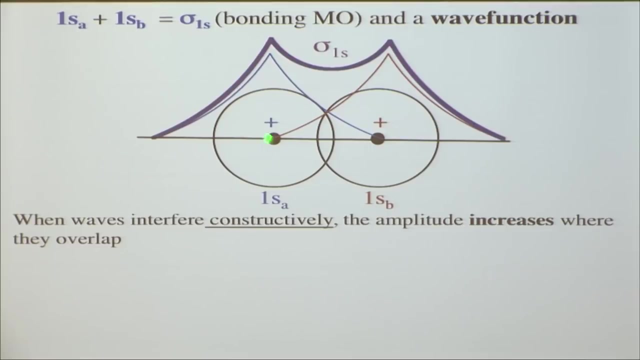 function for 1sb, These wave functions come together- Here's one nuclei, Here's the other nuclei- And for a bonding orbital it'll be constructive interference, And so the amplitude where these atomic wave functions overlap will be increased. when you have constructive interference, 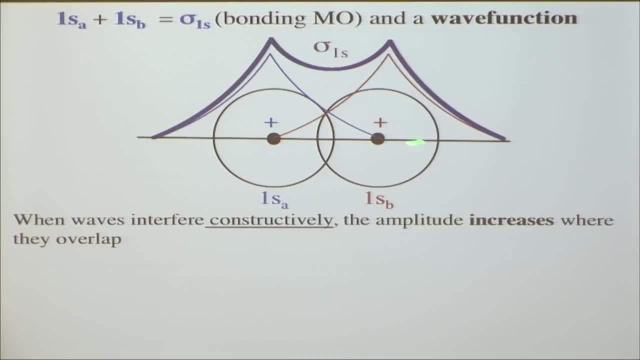 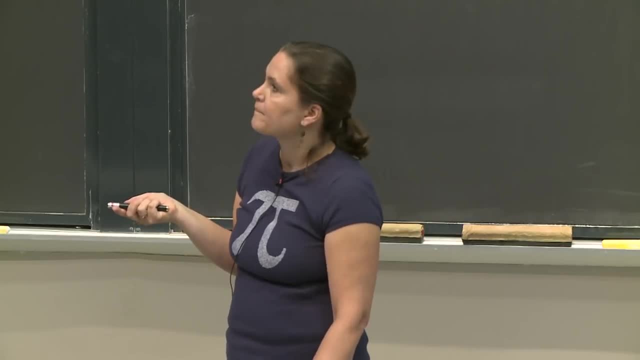 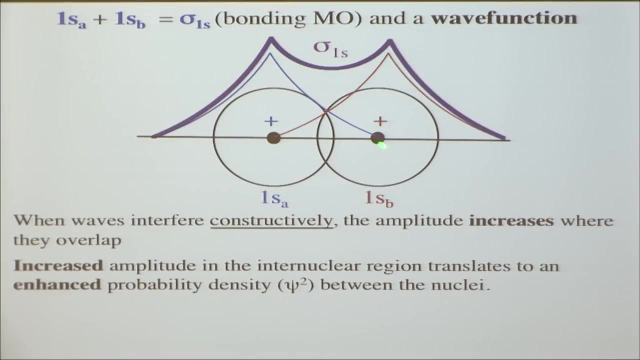 So our sigma 1s now has increased amplitude between these two nuclei due to that constructive interference. So an increased amplitude between these two nuclei, which again, this is the bonding axis- Here's one nuclei, Here's another- So an increased amplitude here corresponds. 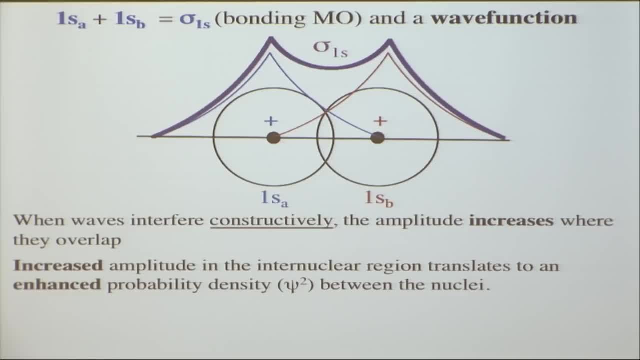 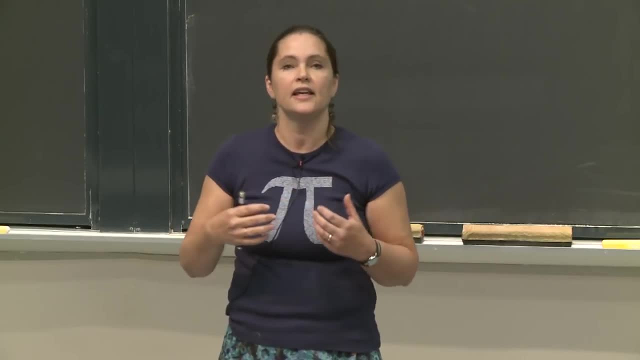 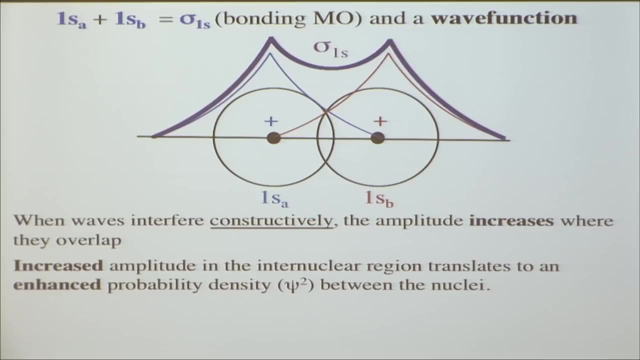 to an increased or enhanced probability density. Remember our wave function, squared is probability density. It suggests the likelihood of finding an electron in a certain region of volume and if it's enhanced by this constructive interference. So if that density, probability density, is enhanced, you have a greater chance. 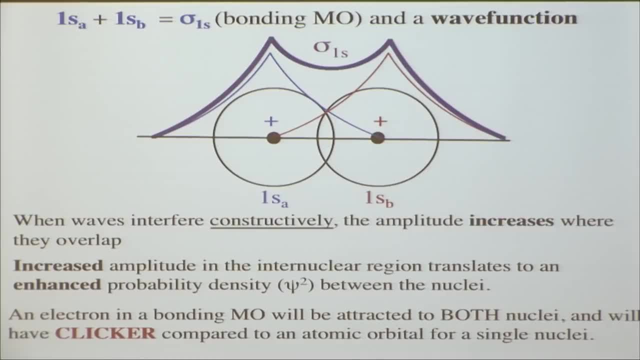 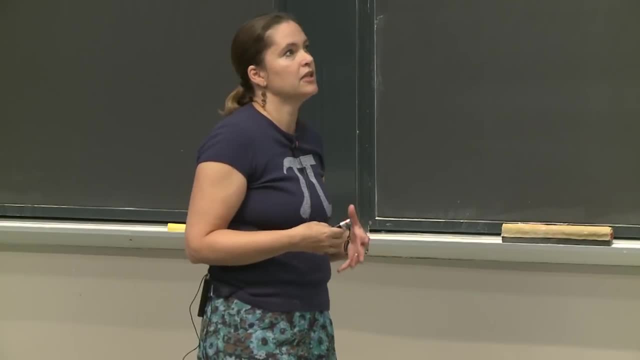 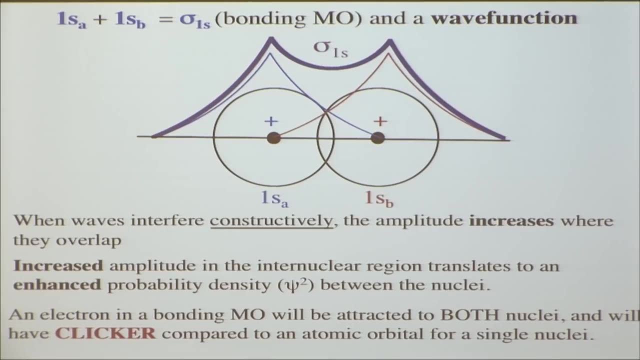 of finding an electron between these two nuclei, which will be attracted by both nuclei. So now, why don't you tell me what you think is going to happen to an electron that is in this region of constructive interference, this increased area of probability, density? 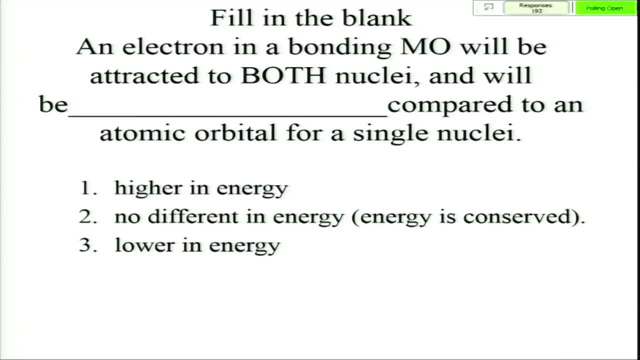 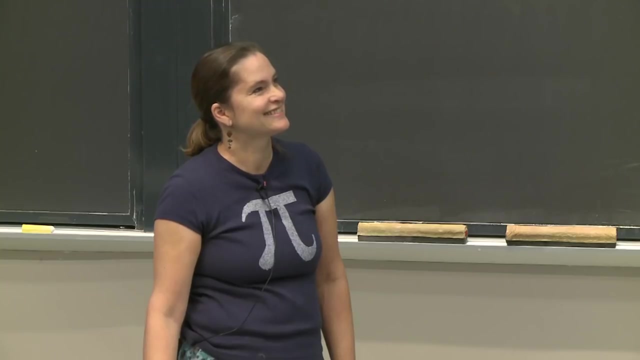 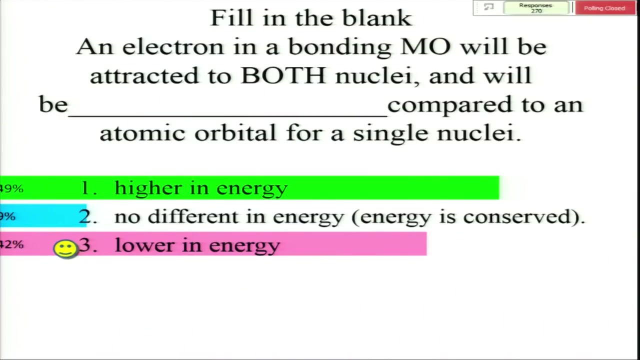 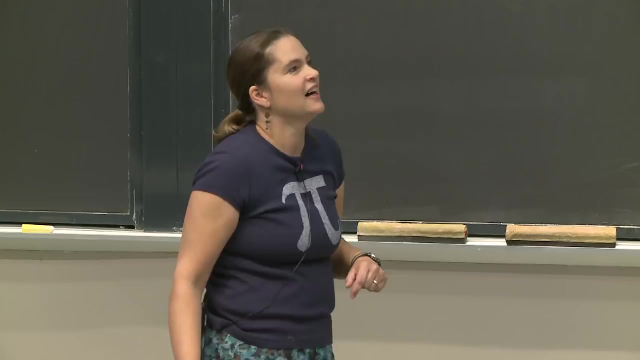 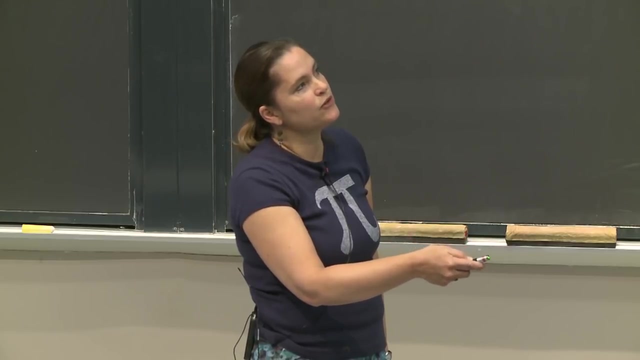 OK, 10 more seconds Interesting, OK, So we should have probably not put up the answer there and re-poll. So yes, so here, if we have an electron that's attracted to both nuclei, then we want to think about whether that's. 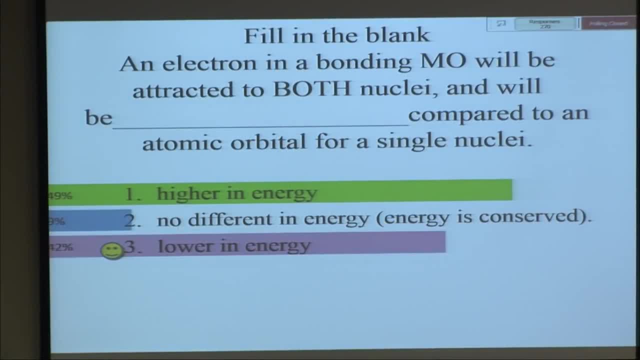 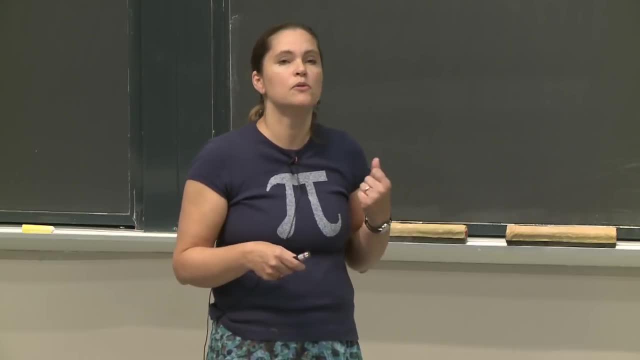 going to be lower or higher in energy than something in an atomic orbital. So if it's attracted to both, it's going to be more stably bound to those. It'll be harder to remove that electron, which means that it's lower down in energy. 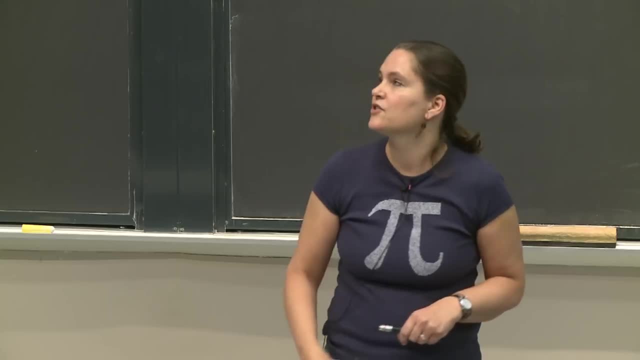 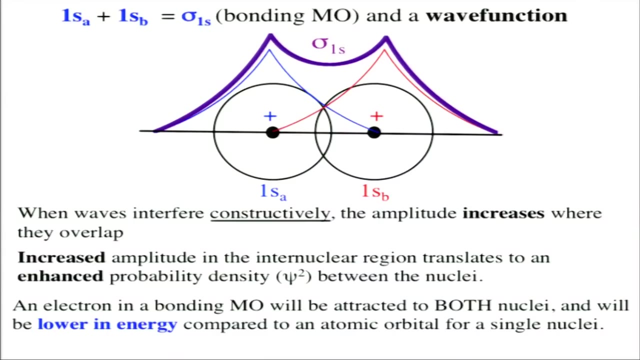 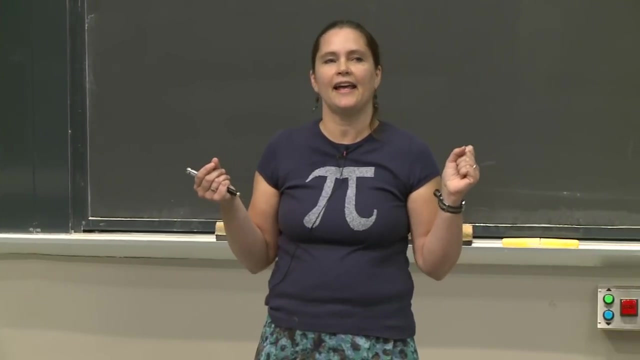 And so we should look at that and we're going to. So the answer is it should be lower in energy, more stable, harder to remove that electron. It's in a sweet spot, It has two positively charged nuclei and it's kind of hanging out right in the middle. 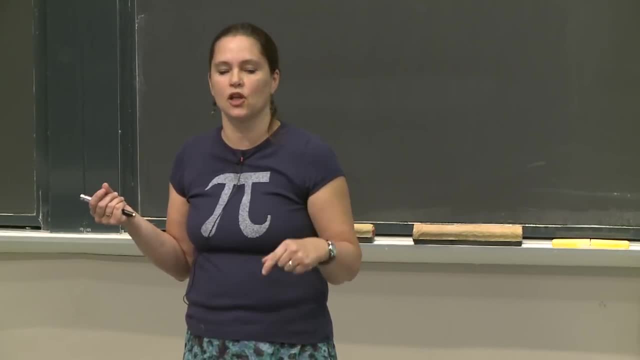 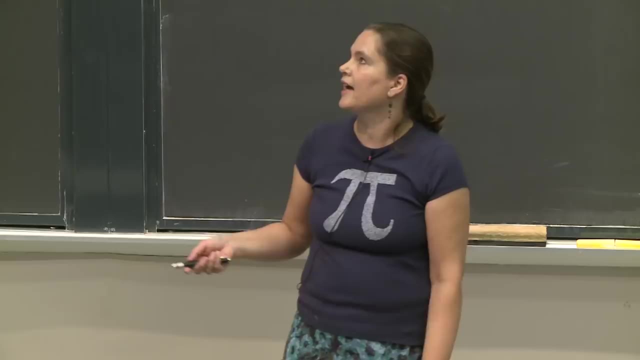 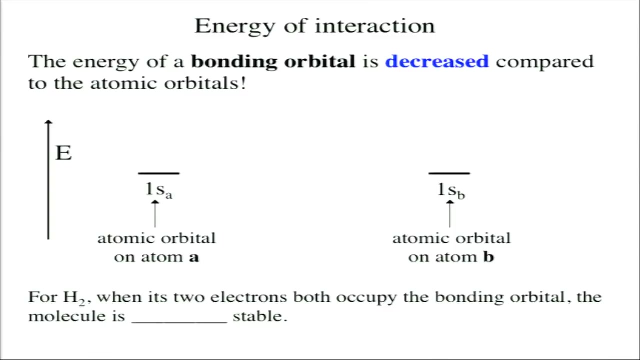 It's very happy. It's going to be more stable and that means lower in energy. All right, so let's take a look at that. So the electron is lower in energy and the bonding orbital energy is also going to be decreased compared to the atomic orbitals. 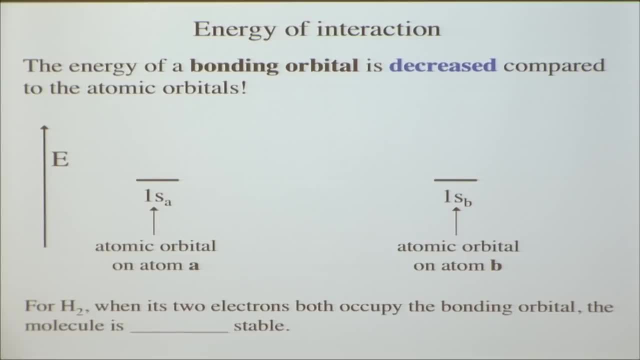 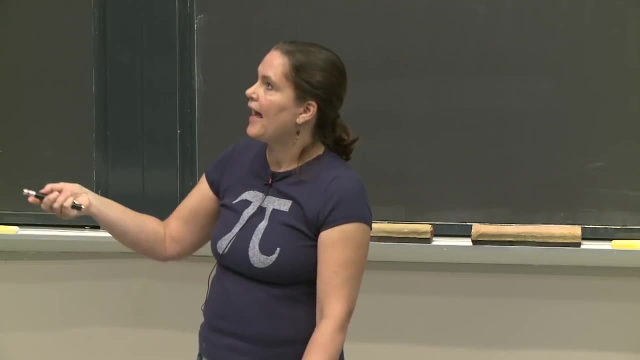 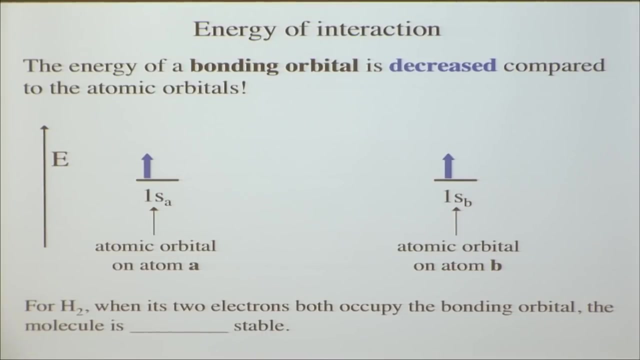 and that has to be true if that's where the electron is. So let's look at the atomic orbital from a and the atomic orbital from b, And now I'm going to put the bonding orbital at a lower energy level. First I was going to put the electrons on. 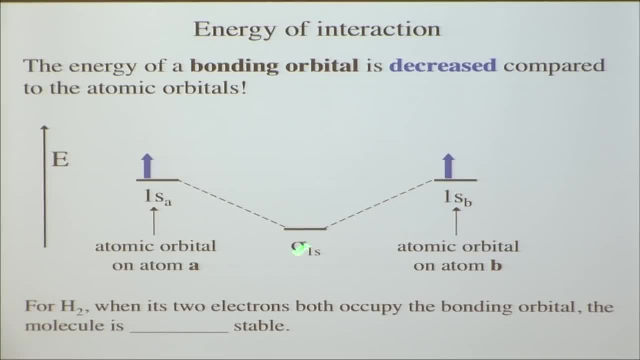 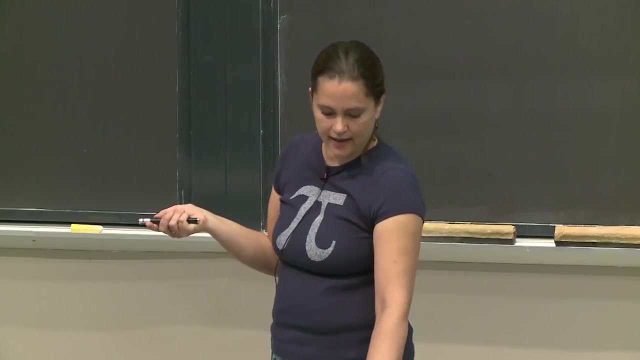 and now I'm going to put the orbital at a lower energy. So remember, this is increasing energy here. So the atomic orbitals would be up here, whereas the molecular orbital is down here. Molecular bonding orbital will be lower in energy And now we'll put our electrons there. 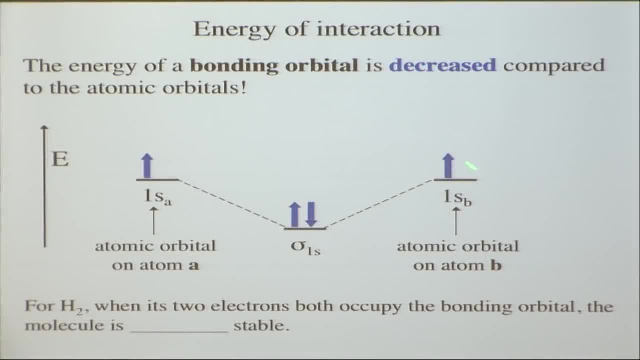 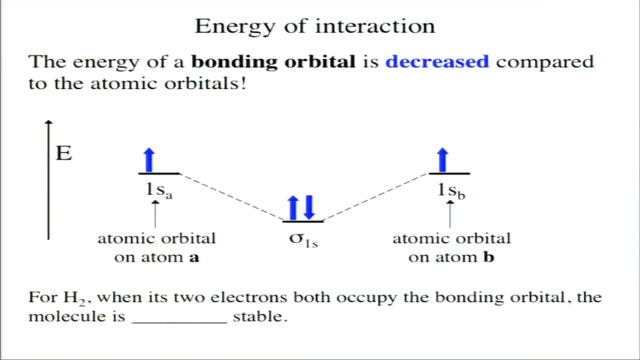 So we have one electron up here and one here, And so when they come together we're going to have two electrons in this molecular orbital. So when you have these two electrons and they both occupy the bonding orbital- and this is the case for H2, each H atom 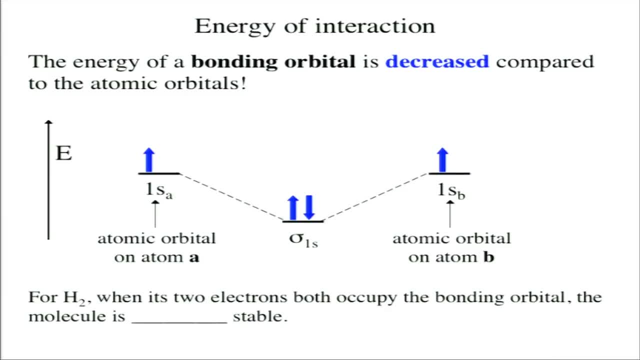 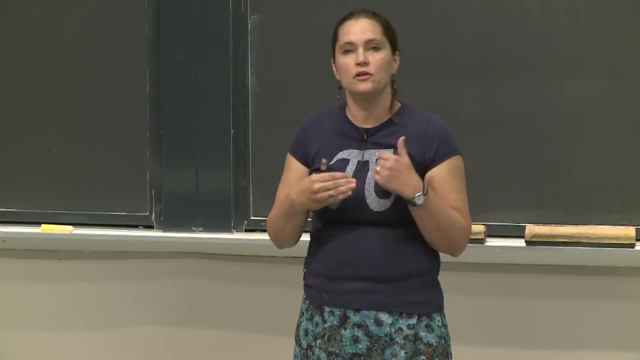 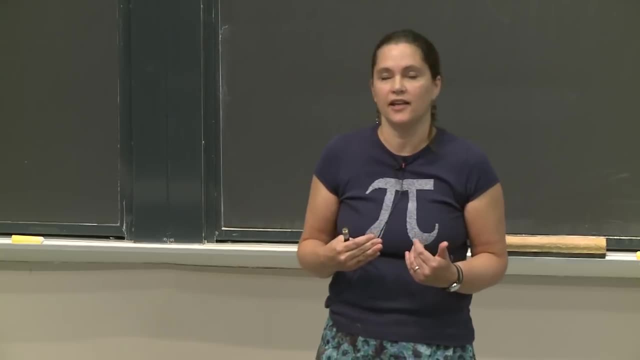 is bringing one electron. H2 has these two electrons and that's going to make H2 more stable And we saw that before that you have to dissociate the H2 bond, You have to add energy into the system. H2 is more stable than free H plus H. 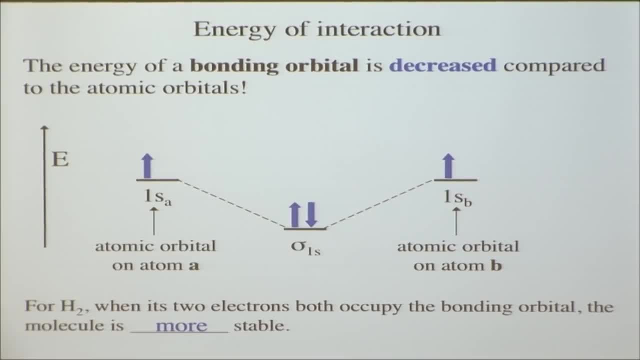 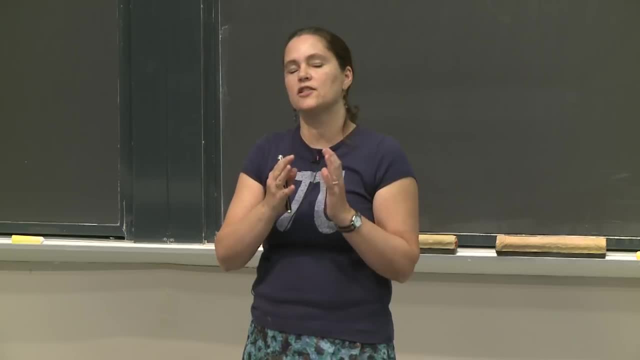 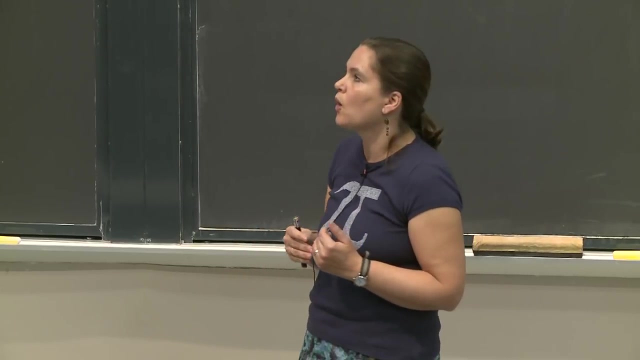 So when you bring atomic orbitals together and you have constructive interference, an increased probability of electrons between those two nuclei, that's a sweet spot. Those electrons are going to be very happy there and that will result in a more stable, lower energy structure. 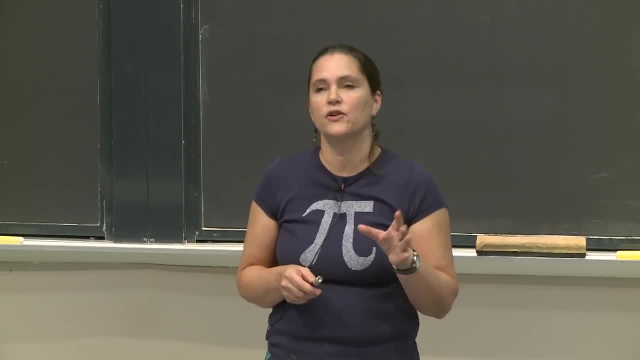 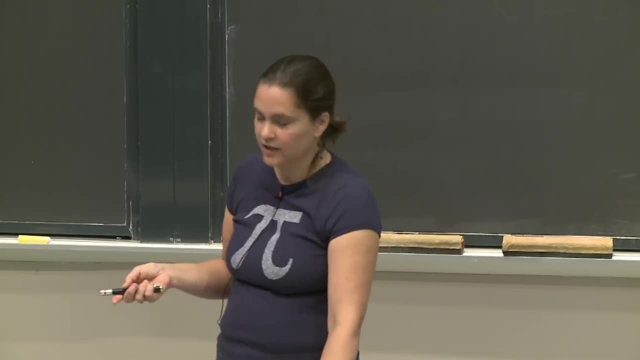 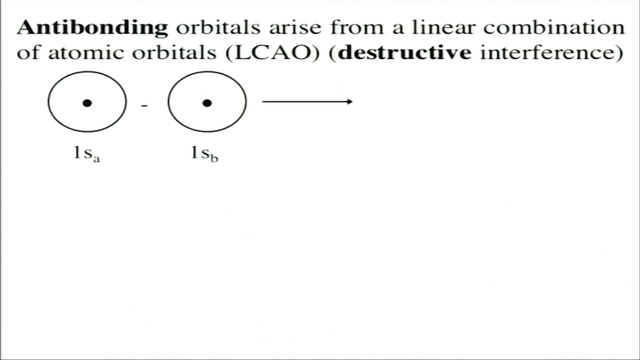 That's bonding. But whenever there is a positive event like this, there's always a negative event, because that's just how life works. So we have bonding orbitals, but we also have antibonding orbitals. So antibonding orbitals arise from the linear combination. 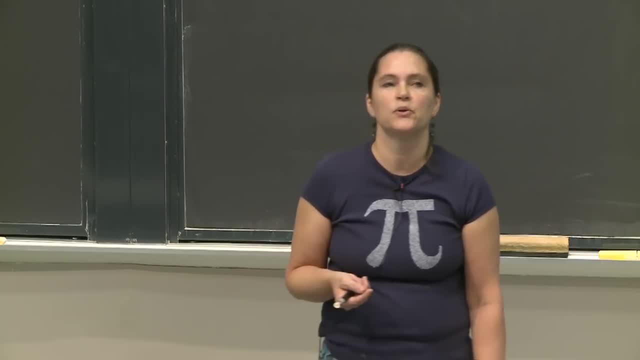 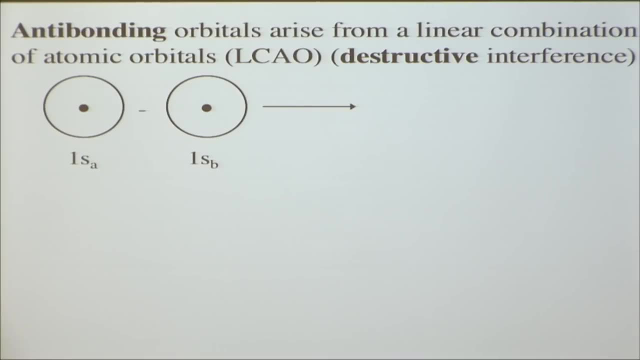 of atomic orbitals, LCAO, through destructive interference. So here these are going to be destructive, These are going to be destructively interfering And that will generate a molecular orbital that is an antibonding orbital. So here are little nuclei again. 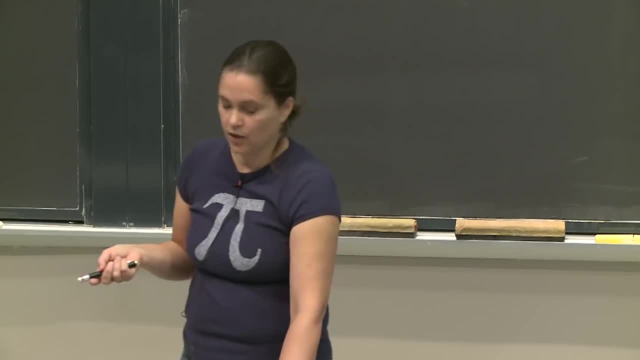 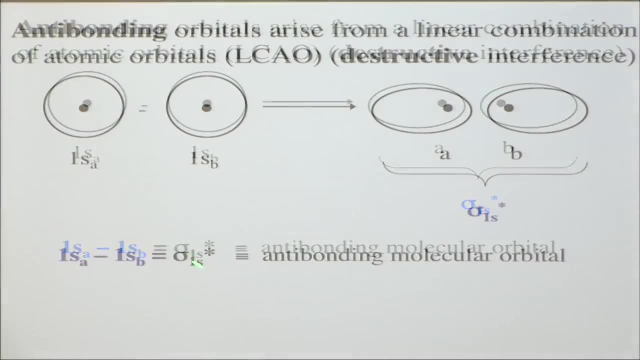 And this antibonding orbital is called sigma 1s star. So we can write an equation for this as 1sa minus 1sb equals sigma 1s star. That is an antibonding molecular orbital. And let's just think about how this kind of shape 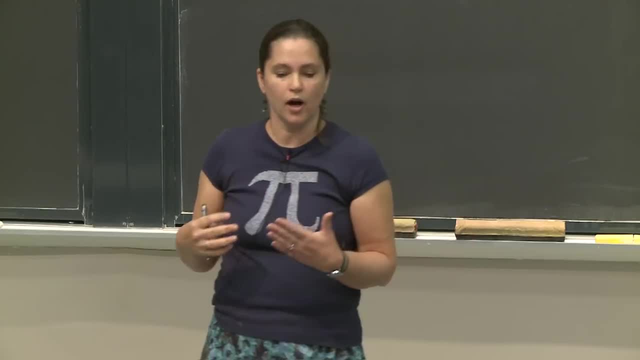 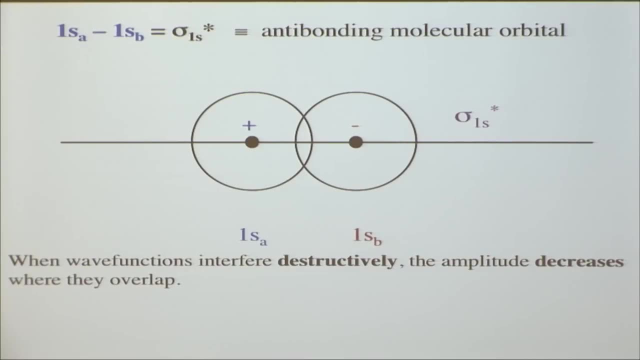 arises, considering the wave-like properties of these atomic orbitals. So I'm going to now move this equation up to the top, And now I have my 1sa here, my 1sb here, And now it's destructive interference. So we have opposite phase of the wave functions. 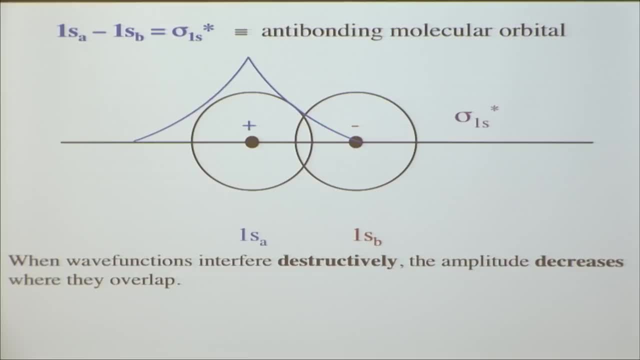 And when we'll put up? We'll put up a wave function there. Now the next one has the opposite phase, So they're going to destructively interfere. There is overlap over here, But when you have destructive interference then the amplitude is going to decrease. 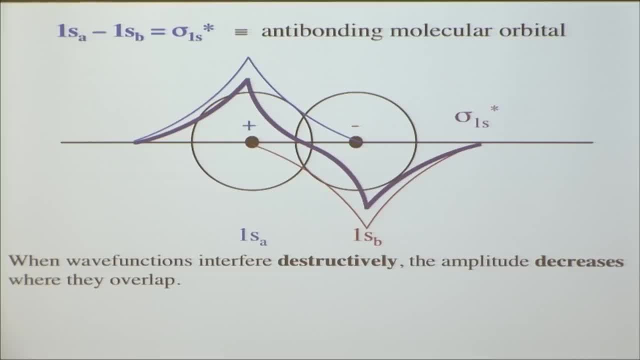 So now, when we consider this destructive interference between these two orbitals, you see that you have what arises between them. Instead of enhanced probability of finding an electron, you actually get a node. So you have decreased amplitude, translates to decreased probability density between these two nuclei. 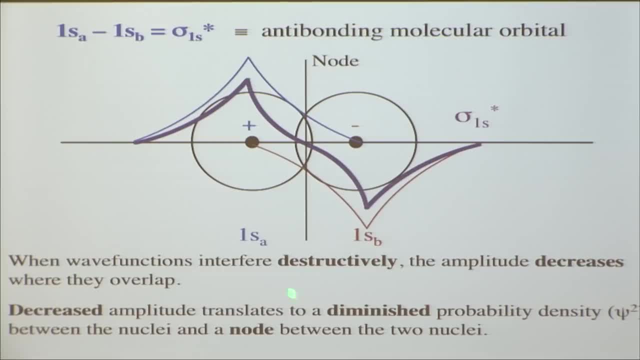 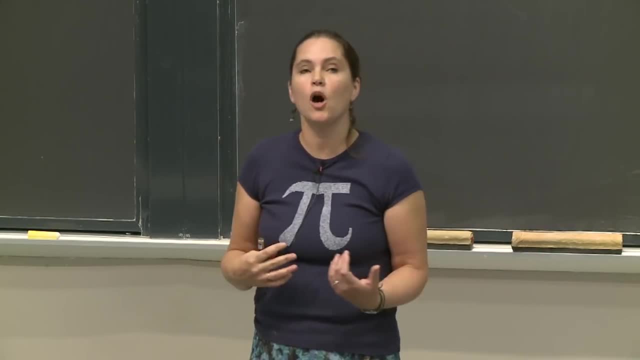 one here, one here, And that results in a node between the two nuclei. So in the antibonding orbital there's a much lower probability that it will be in this sweet spot between these two nuclei. So that's what we're going to do. 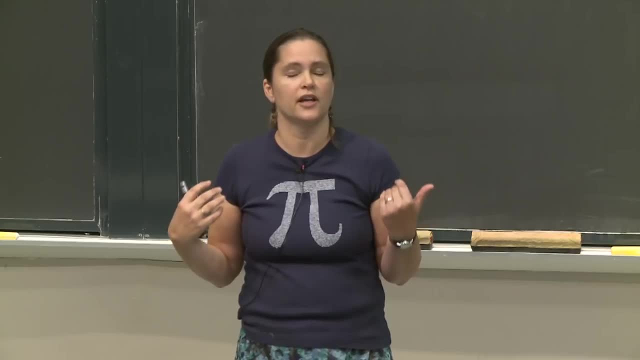 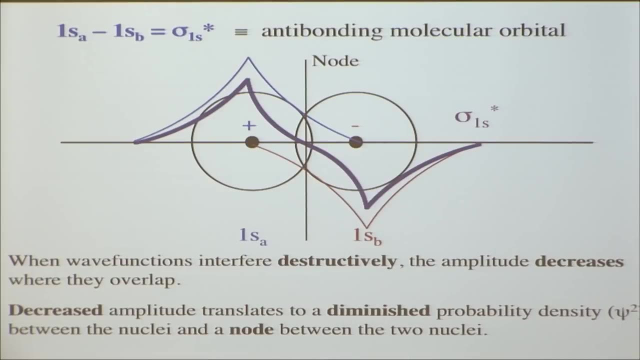 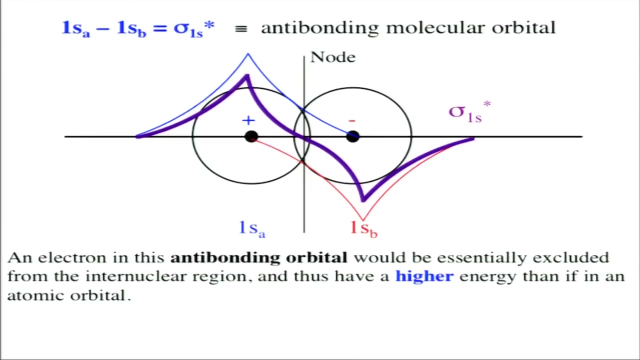 It's going to be in the sweet spot between the two nuclei that have this nice positive charge for its little negative charge. So there's pretty much no shot at being in that nice sweet spot, And so what that ends up meaning is that an electron in an antibonding orbital 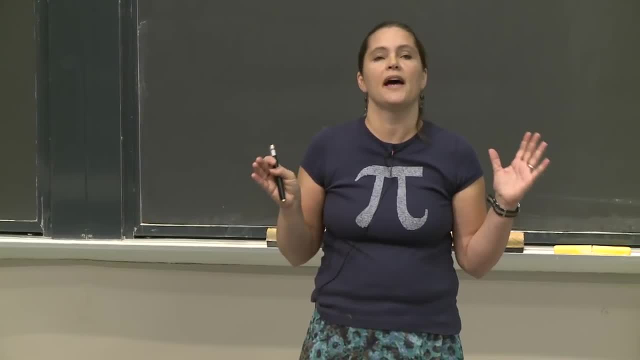 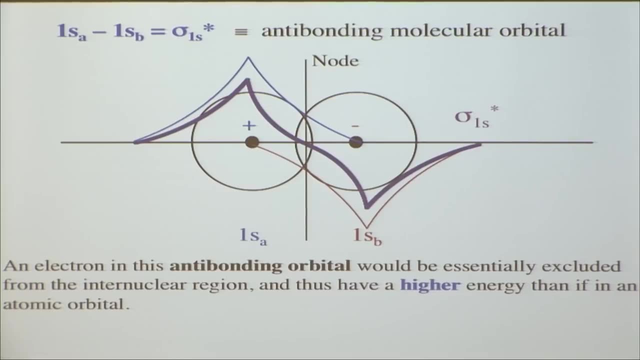 is pretty much excluded from that internuclear region, that region between those two nuclei, And that results in a molecular orbital that has higher energy than the atomic orbital. There's just no chance of being in that wonderful spot. It's really very sad for the poor electron that. 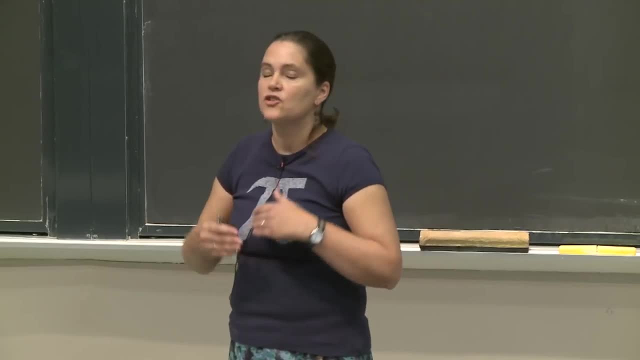 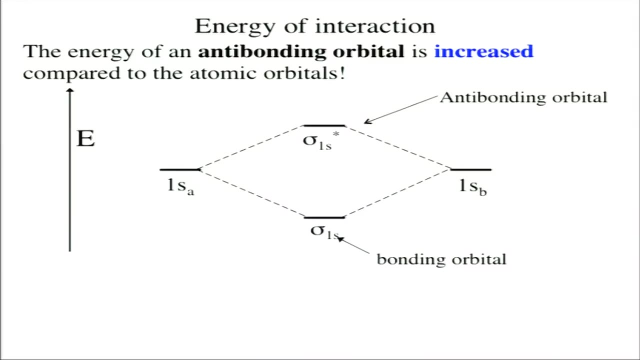 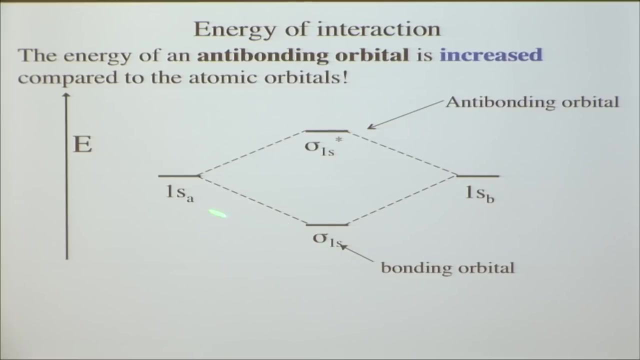 has to occupy an antibonding orbital. So now let's put this on our energy scale. So we'll go back to our energy scale. And we saw before that when we had 1sa and 1sb and you had a sigma 1s, a bonding orbital, 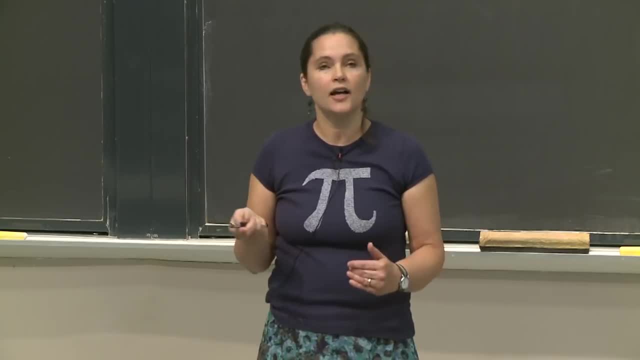 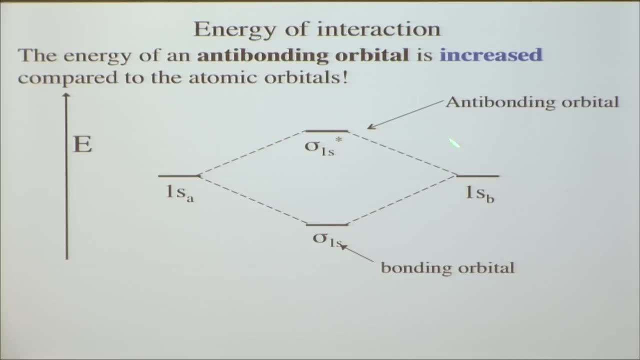 that was lower in energy. Electrons that occupy it are more stable compared to their positions in the atomic orbital. But we also now have an antibonding orbital from destructive interference between the wave functions of the atomic orbitals, And that's higher in energy. 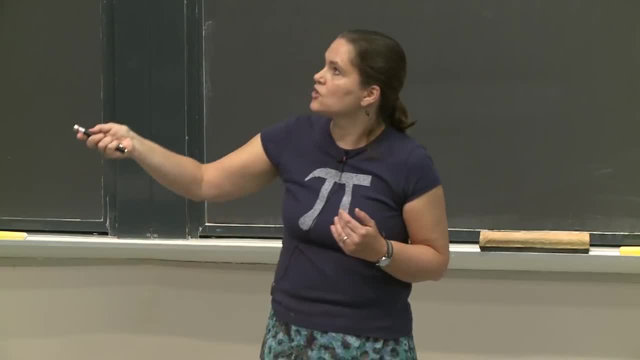 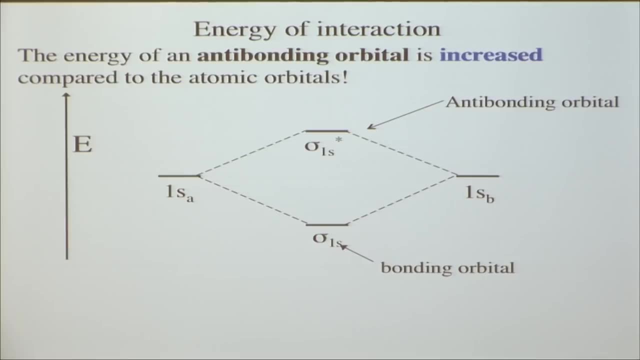 And so that's up here. So this is what our diagram is going to look like. that brings two atomic orbitals together to create two molecular orbitals. So The antibonding orbital up here is raised in energy by the same amount that the bonding energy is lowered. 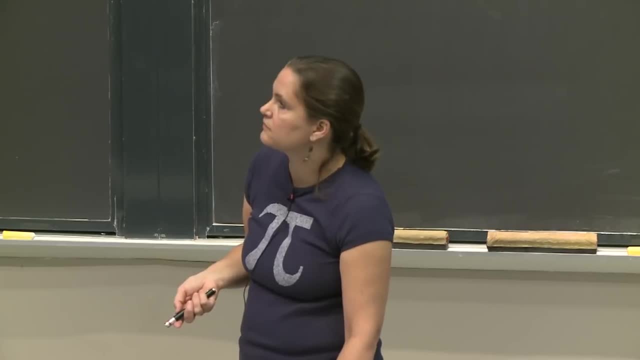 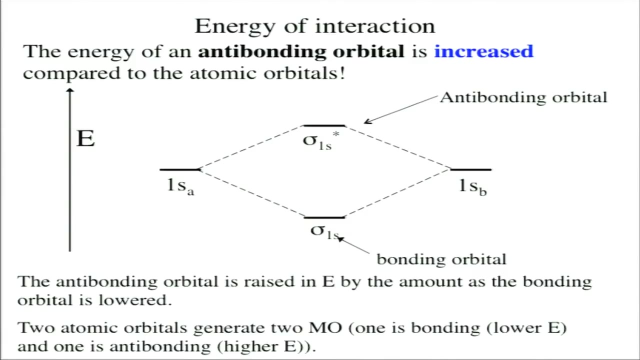 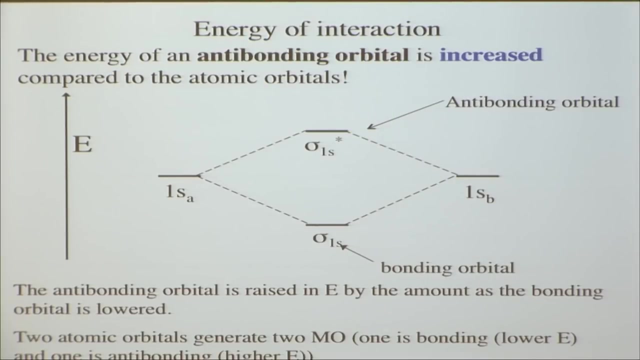 And so that gives rise to this diagram. And importantly, as I mentioned, we have n atomic orbitals forming n molecular orbitals. So if we have two atomic orbitals, we generate two molecular orbitals. One is bonding lower in energy. 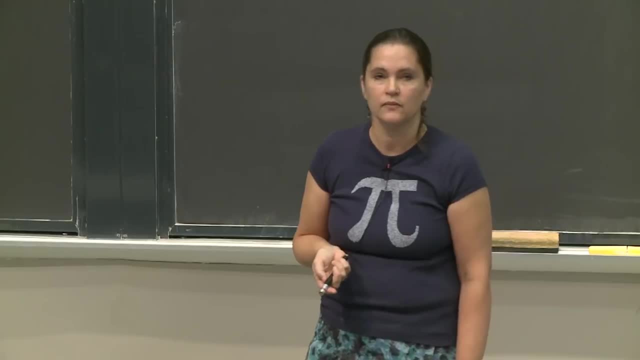 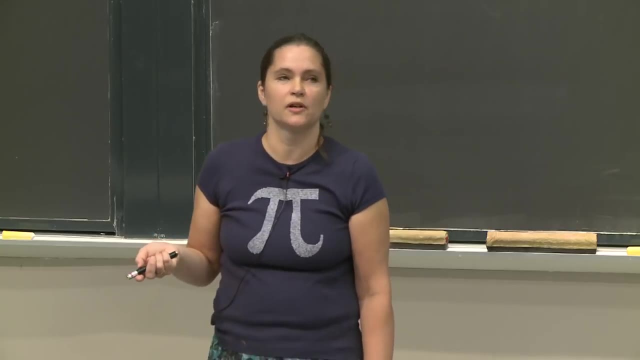 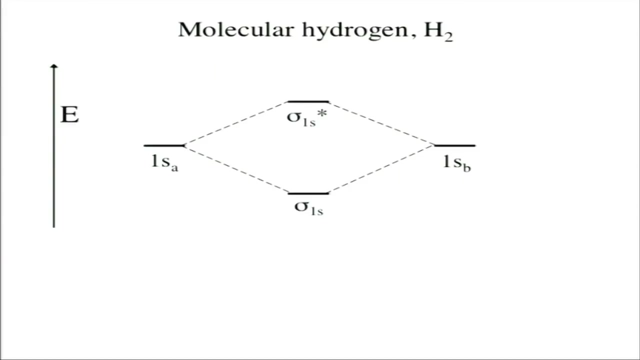 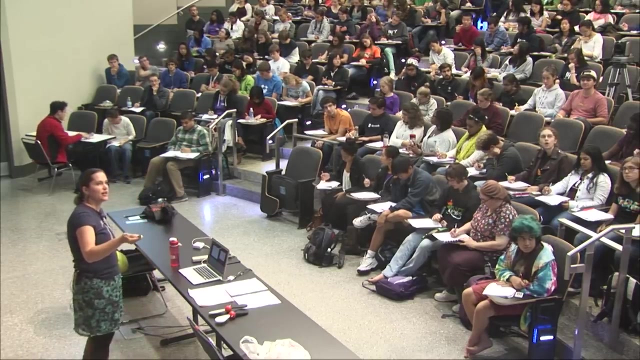 And one is antibonding, higher in energy. All right, So let's take a look at some examples. So always start with hydrogen. So hydrogen has how many electrons? One hydrogen Hydrogen atom One, So we have two hydrogen atoms. 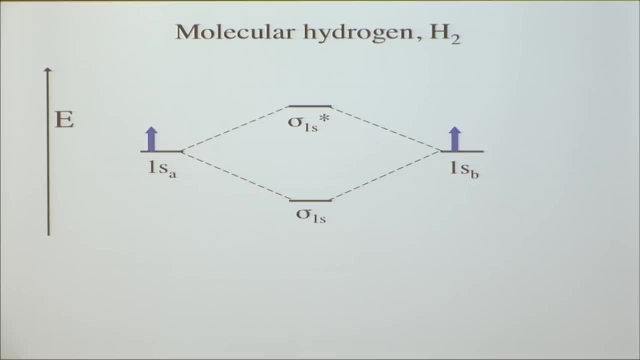 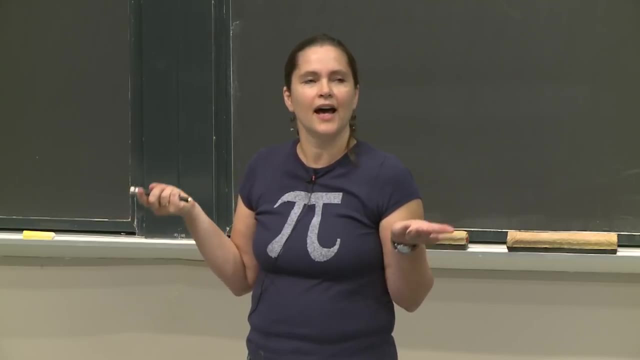 And so we have two 1s orbitals, 1sa, 1sb. And now we're going to. where do we want to put our electrons In the highest energy possible, lower energy, where do we want to put them? 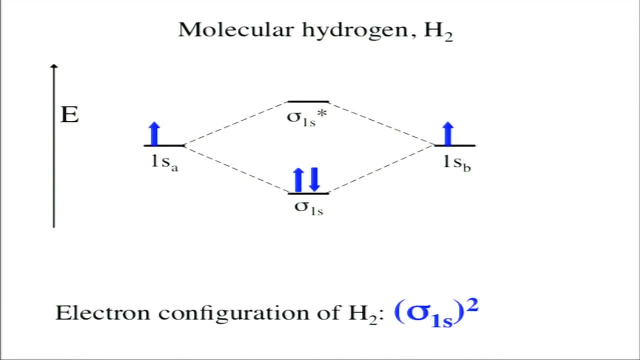 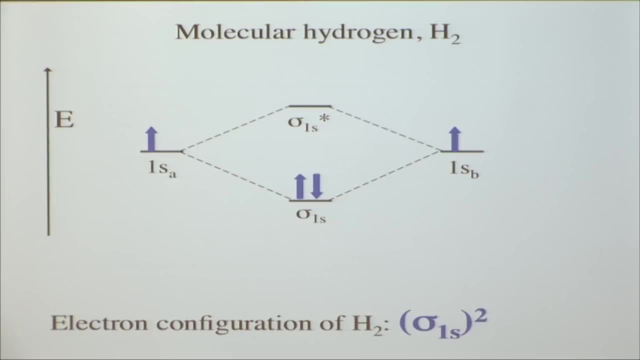 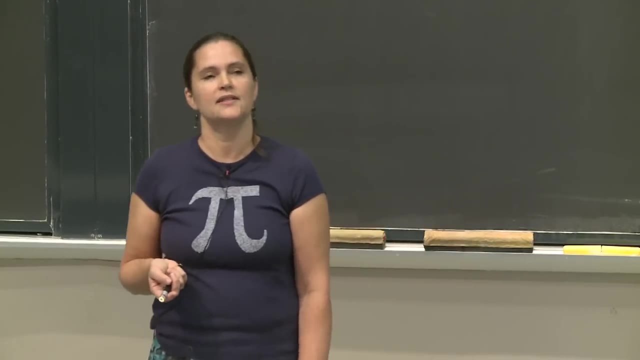 Always start with lower energy. So we're going to put them down here, And so this is now the MO diagram for H2.. And we can write the electron configuration for the MO diagram, which, you'll note, is a different electron configuration than you're going to see. 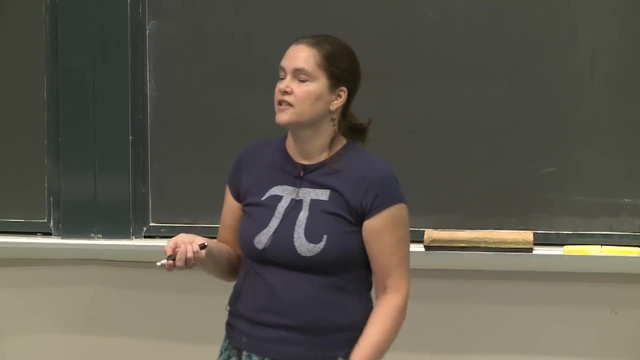 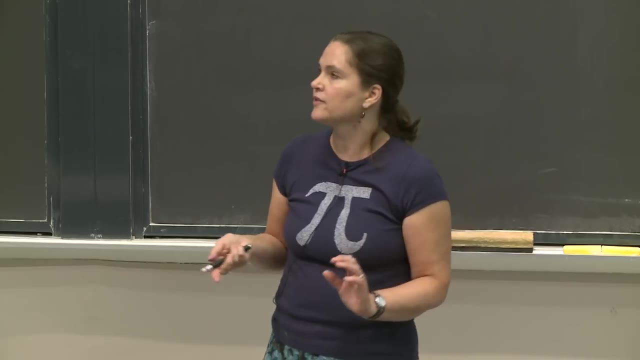 So we're going to write the electron configuration than you were writing when you were looking at the periodic table, because now we're not writing it in terms of 1s2, 2s2.. We're writing it in terms of molecular orbitals. 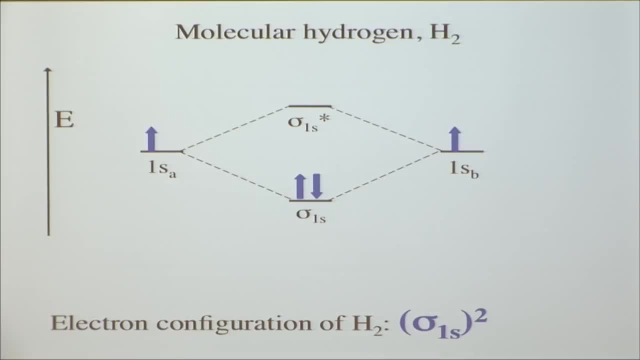 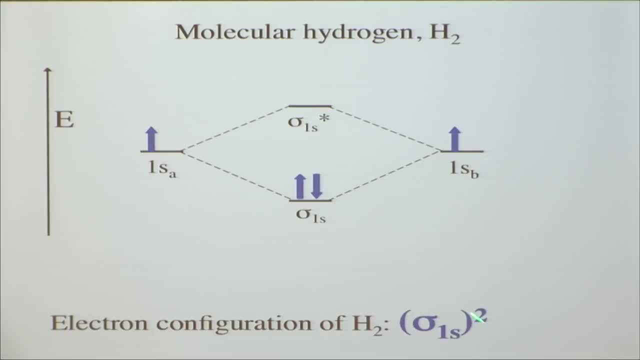 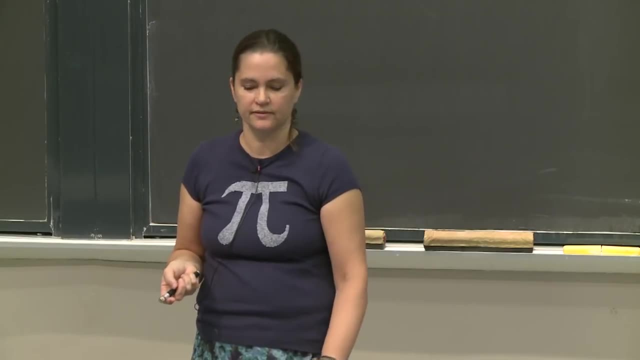 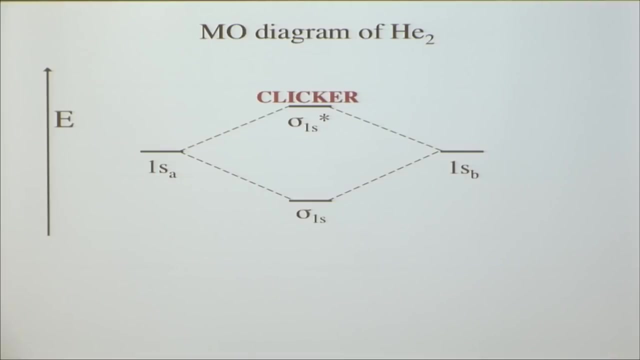 So the answer to this would be sigma 1s2.. There are two electrons in the molecular orbital sigma 1s. Good, So that means that you can do the same thing for dihelium, And that's a clicker question. 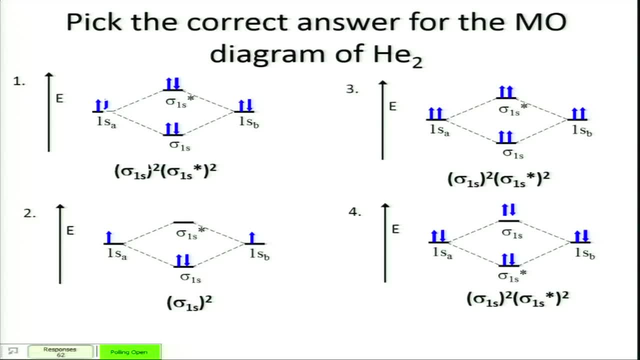 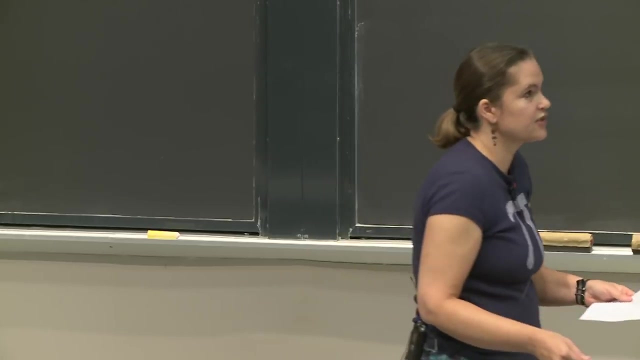 So let's just take 10 more seconds. OK, you can put up Yep, All right. So does someone want to tell me that is correct? What's number 2?? What's number 2 for Hydrogen? For hydrogen. 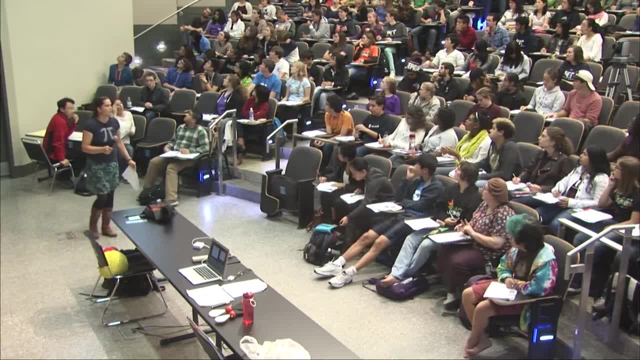 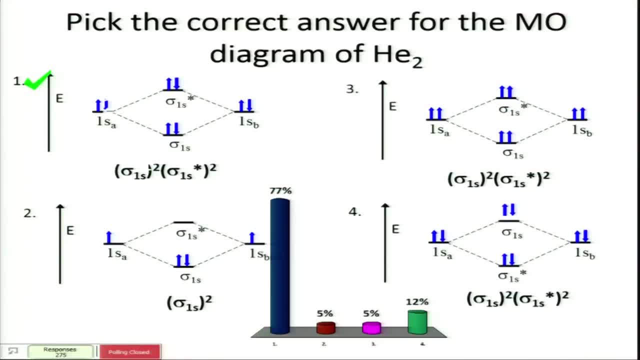 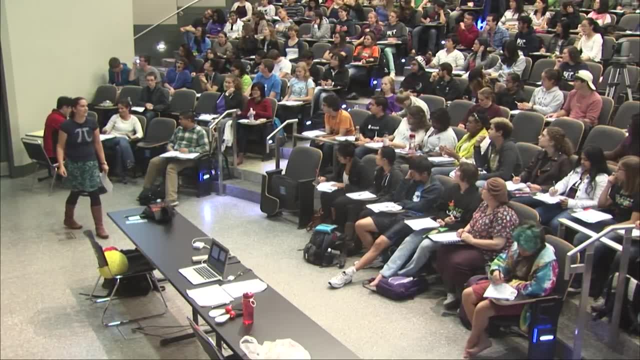 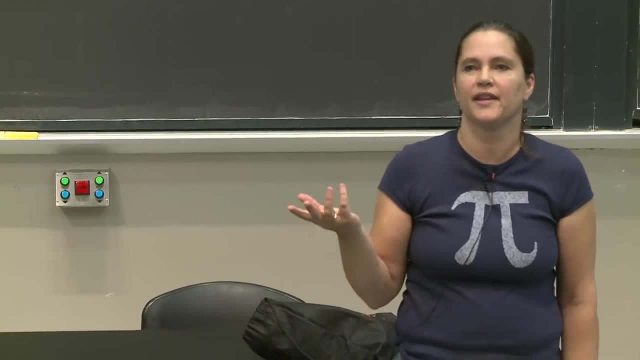 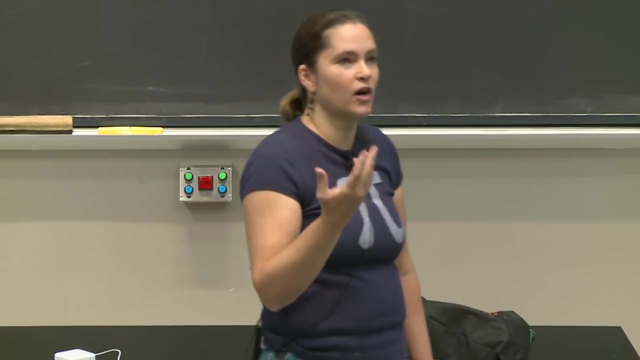 number three: What was wrong there? Okay, everyone's doing really well. yeah, So we had all of the electrons were parallel in there, And what does that violate? What would be true in that case? Yep, And so they'd have the same four principal quantum numbers. This is not allowed. 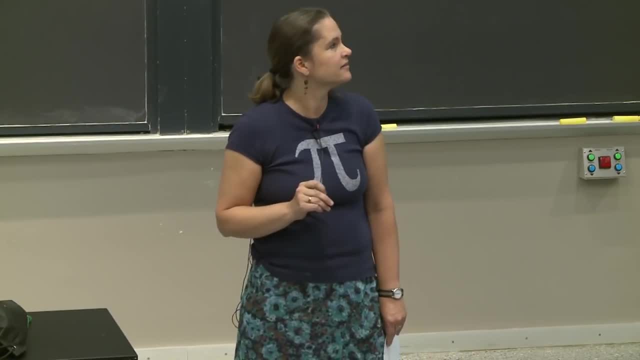 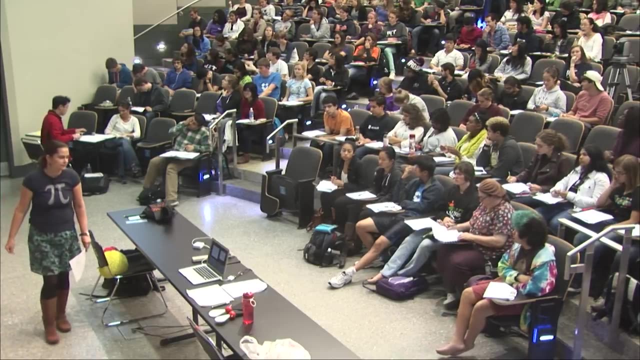 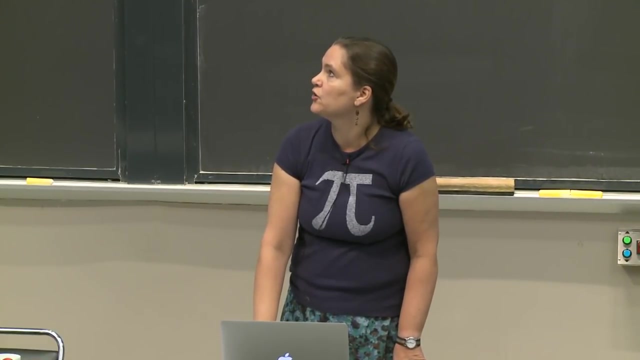 So that one's not good. And what's wrong with four? Yeah, star was on the bottom, So they were flipped around. Antibonding was lower in energy- Great Okay, so we'll just put those in over here. And so we had two electrons. Helium brings two. 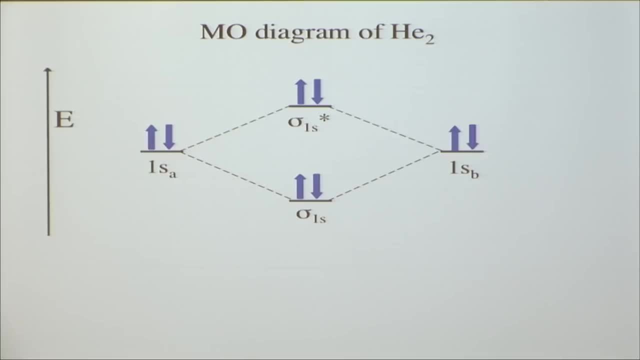 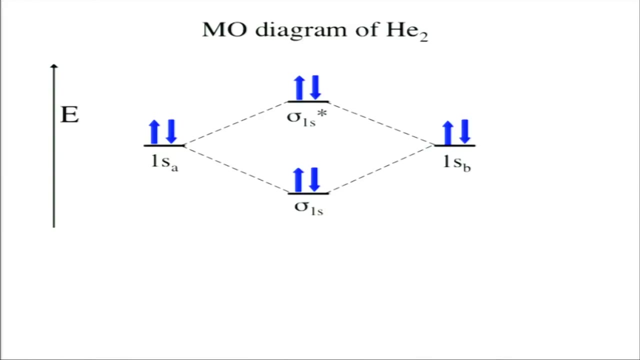 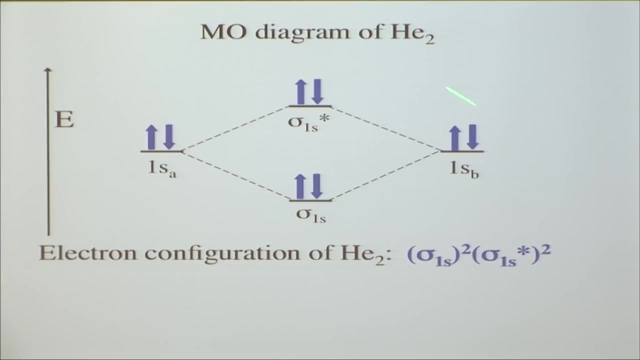 So two went into the bonding and two went into the antibonding with opposite spins And we had: We have the bonding, lower energy, antibonding, higher energy, All right, so then we can put in the electron configuration here And we have sigma 1s2,, sigma 1s, star 2.. So that's the electron. 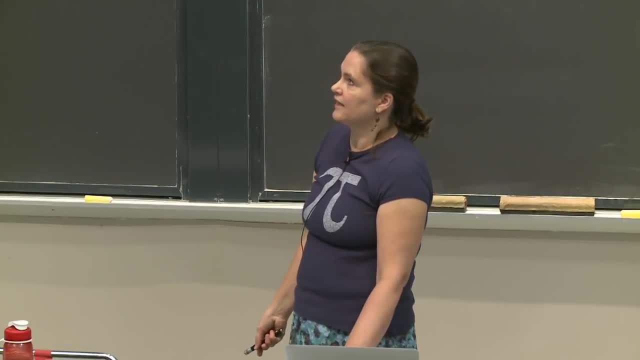 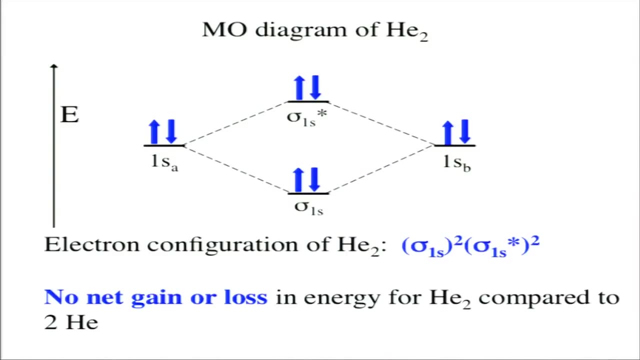 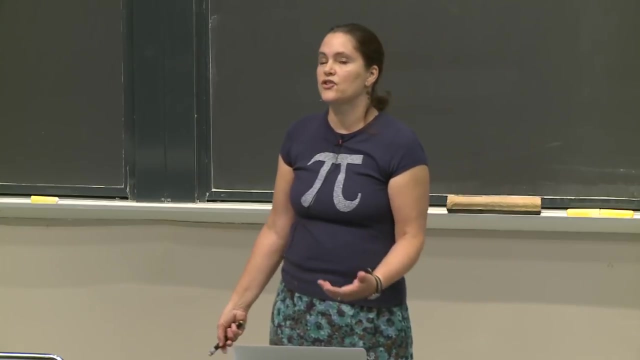 configuration Now. interestingly, you see you have two at lower energy and two at higher energy, So there's no net loss or gain in energy. Well, I think, because you've got a lot of helium, you know there's no net loss or gain in energy. 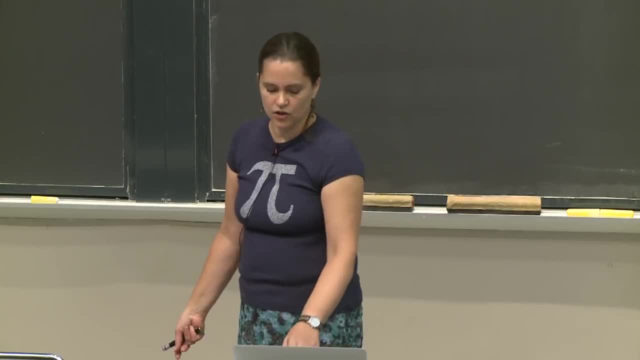 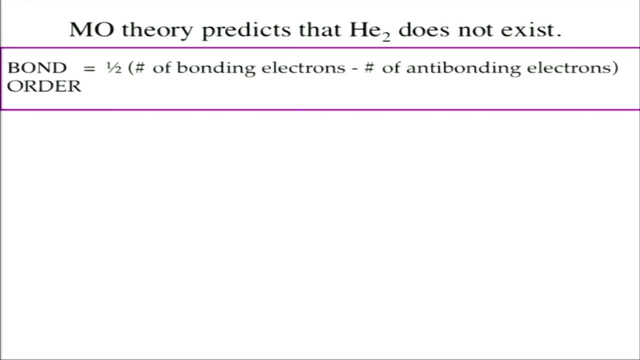 What is the equilibrium? Yes, so the equilibrium can be compared to just one. As a matter of fact, the equilibrium can be compared to just one, And so we can look at the number of electrons. so the equilibrium can be compared to just one. 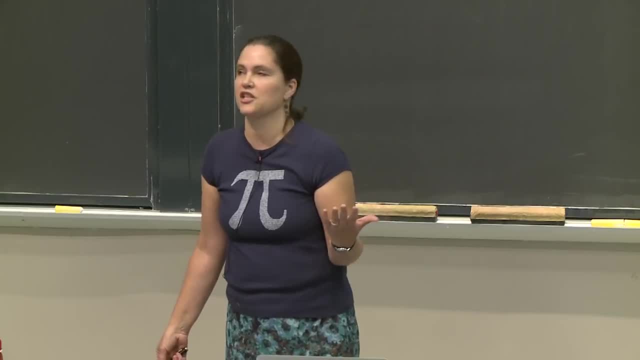 and the number of electrons can be compared to just one, but the equilibrium can be compared to just one. So if we were to just put one element here, I would say, oh, I don't have a really good idea of which one. 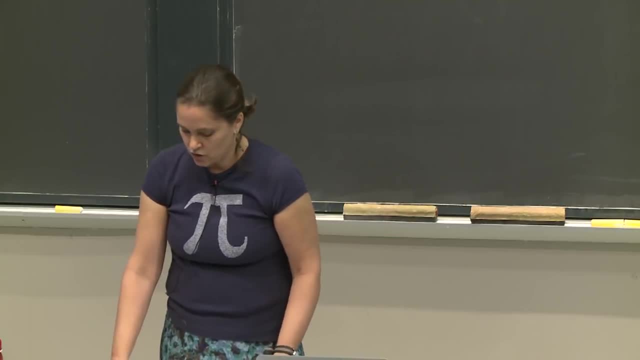 Well, we'll have to go over them now and see where that goes. So we can just go over them to go over to the future. But it's a little bit difficult. So we have a question here. We've got two. Let me just go over them. 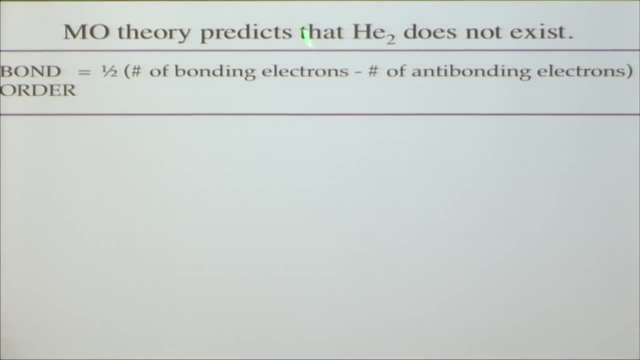 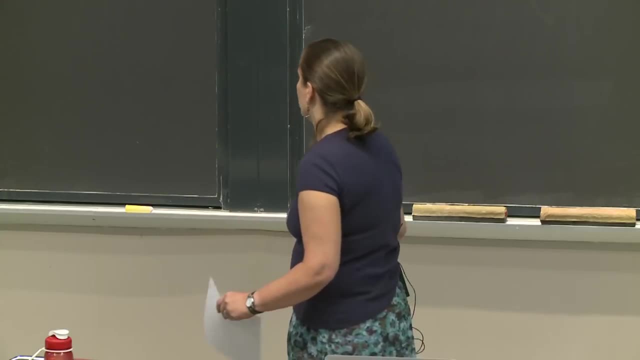 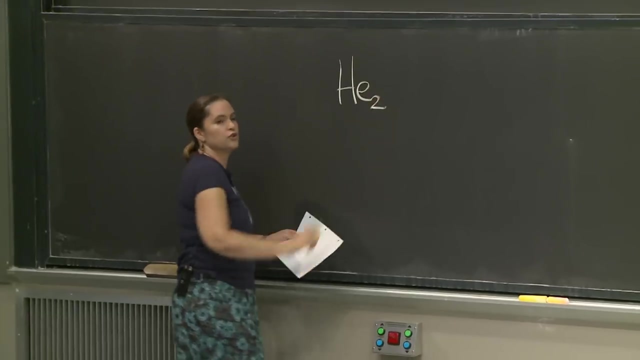 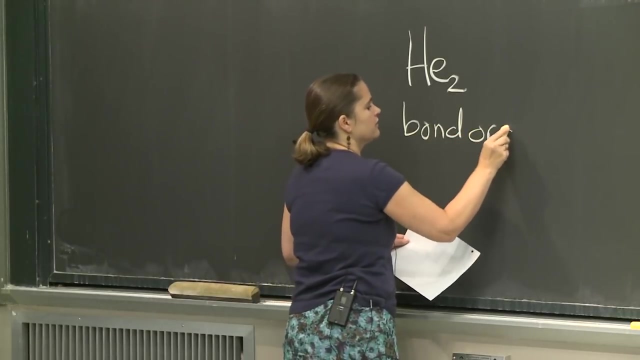 is half of the number of bonding electrons minus the number of anti-bonding electrons. So let's just write out what the bond order for helium would be. So helium 2, our di-helium molecule, So we have bond order equals half. 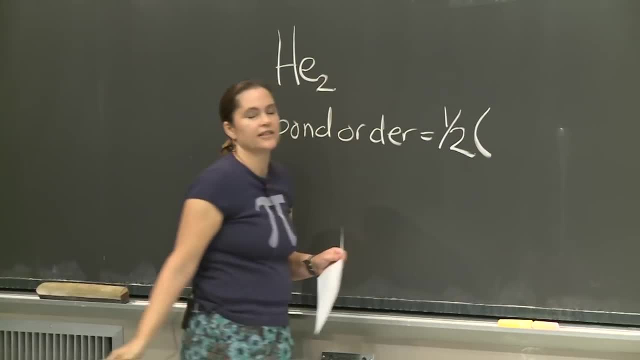 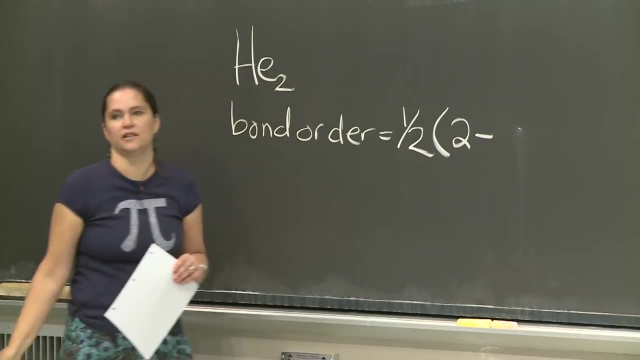 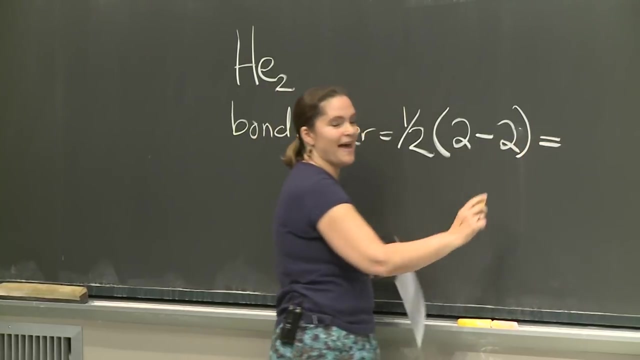 There's always a half And now the number of bonding electrons. So how many bonding electrons do we have for helium 2.? How many anti-bonding electrons do we have for di-helium 2.? And can someone do this math for me? 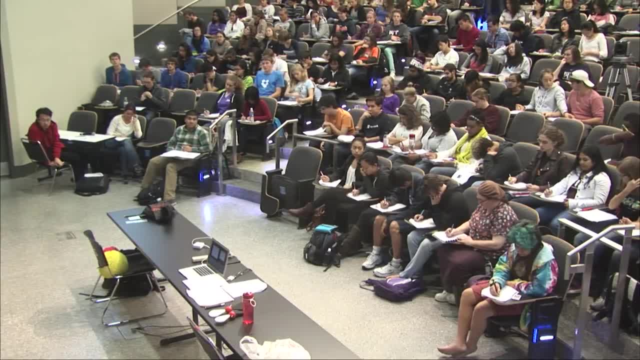 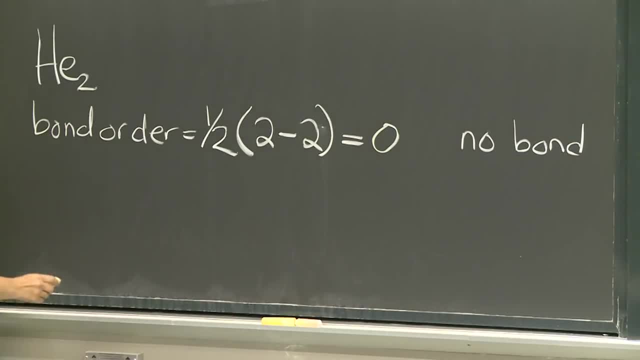 0. So that would suggest a bond order of 0, which means no bond. And let's just compare that to hydrogen H2, which should have a bond order equal to a half. It's always a half In the hydrogen. how many bonding electrons did we have? 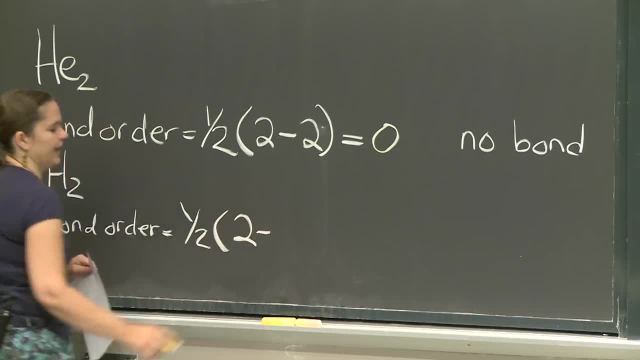 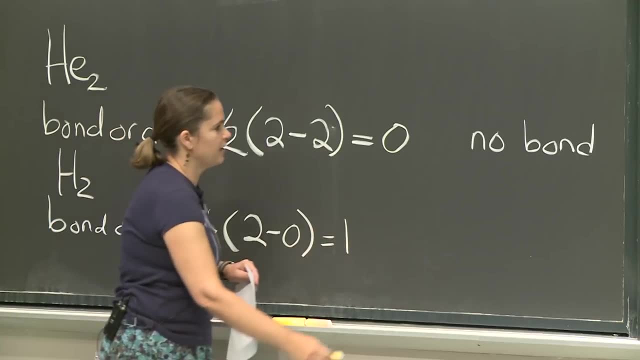 We had 2.. How many anti-bonding electrons did we have 0.. And the math Bond order is 1.. So that means one bond or a single bond: 1. 1. 1. 1.. 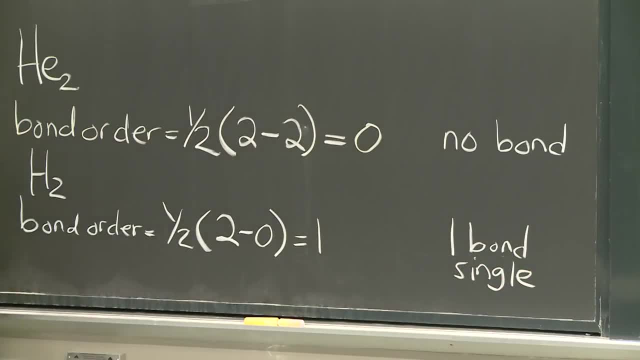 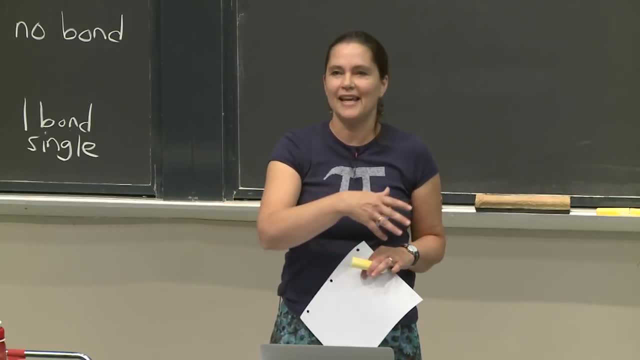 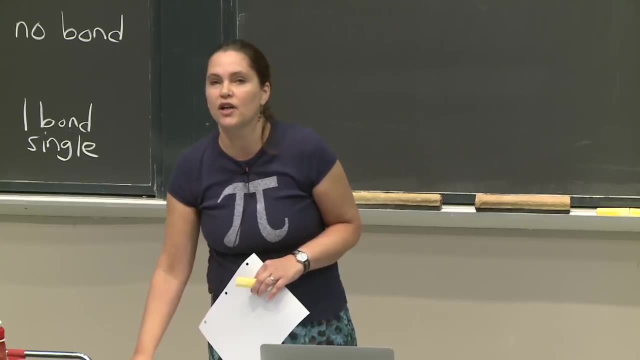 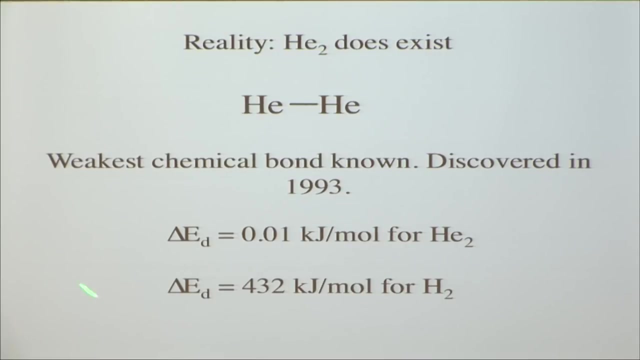 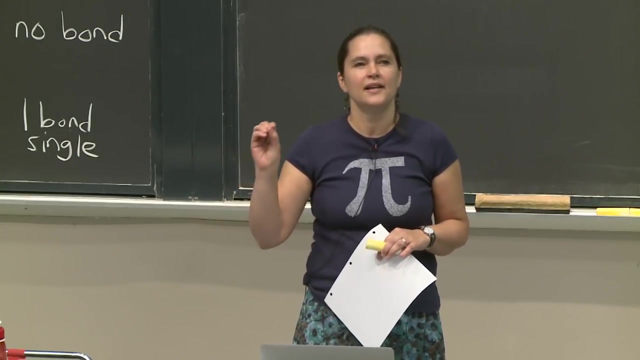 mostly talking about discoveries that were made in the 1800s. it took a long time before someone could prove that dihelium existed, And if we look at the bond association energy for H2, 0.01, and compare that to H2, 432,, dihelium really doesn't exist very much Zero. 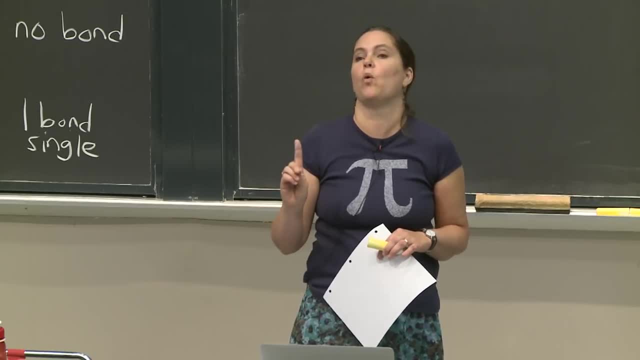 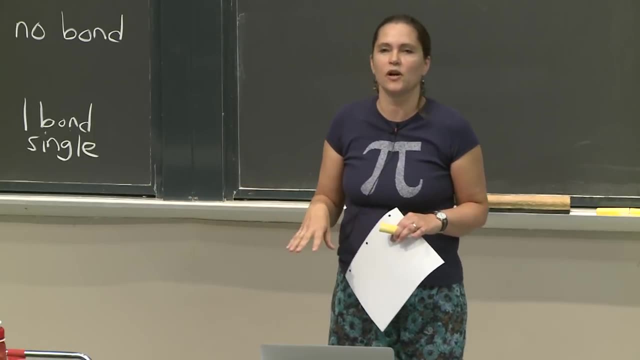 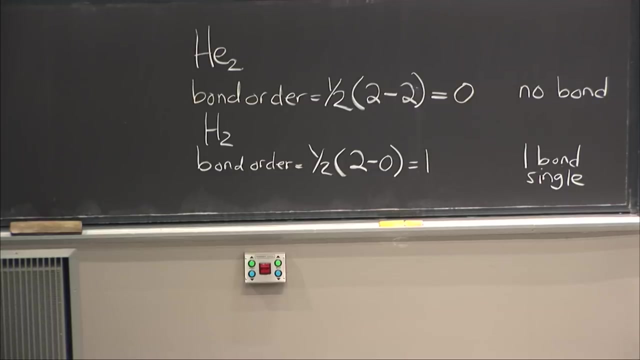 is a much better approximation of its bond than one would be. It really is not a very good molecule, So I would call this a win for molecular orbital theory. It correctly predicts that H2 is not going to be a very good molecule or helium 2 is not going to. 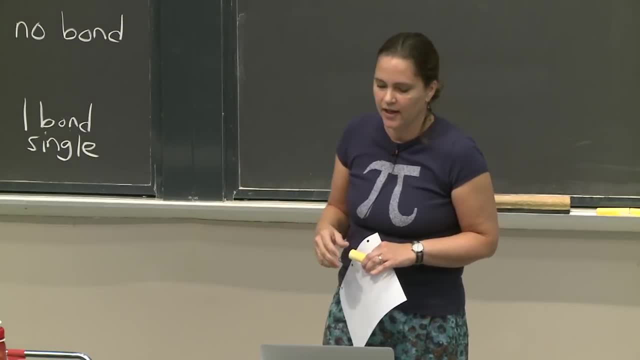 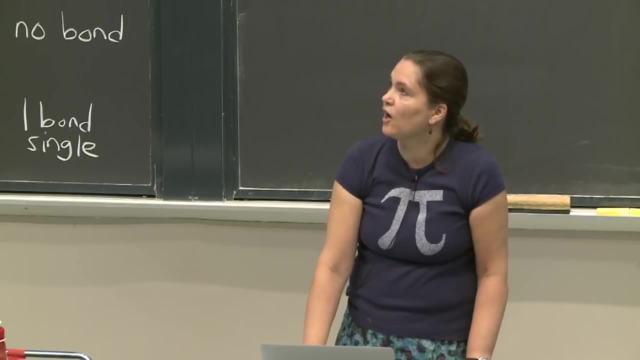 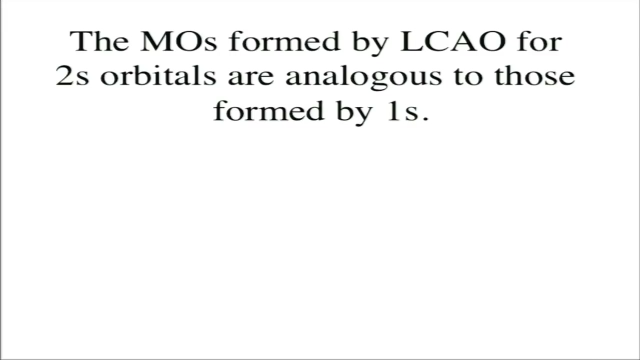 be a very good molecule, but H2 will be a good molecule and that works All right. so now let's consider 2s. So 2s orbitals are analogous to 1s, except that you have to remember that they're bigger. 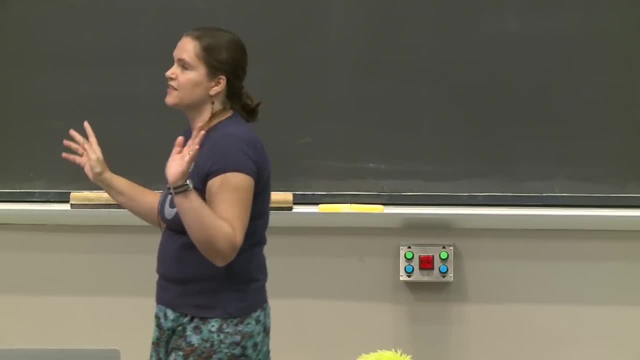 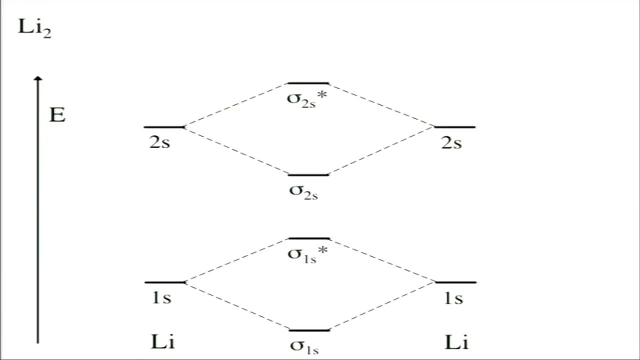 So we have our 1s and our 2s, But for the purposes of this it doesn't really matter. So let's look at a diagram now that has 1s and 2s. So we have lithium. So how many electrons? 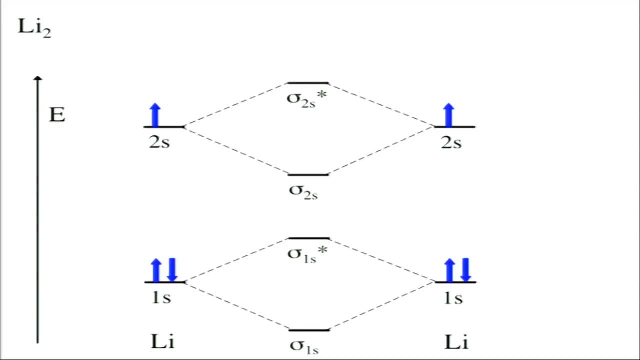 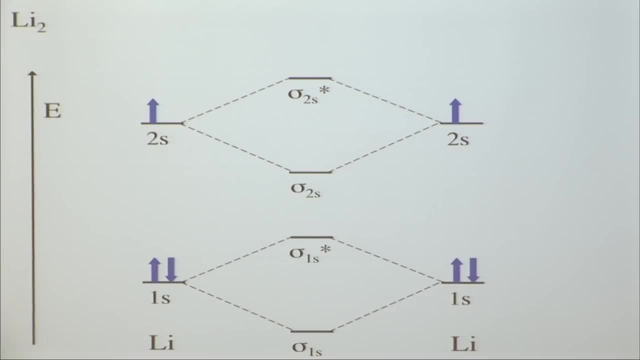 does lithium have? Yep, So we'll put on lithium, dilithium, We'll put on lithiums. It has two in 1s and one in 2s, And so we have one lithium here and one lithium over here And our 1s orbitals. 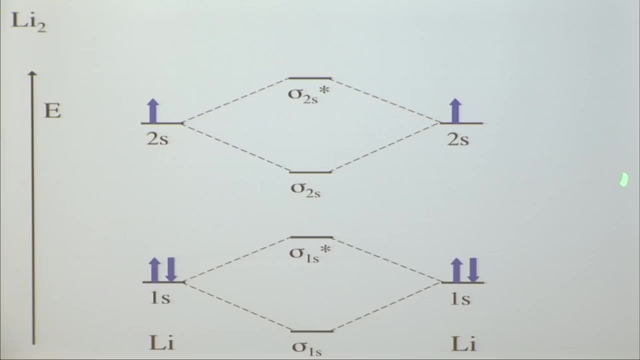 are going to be lower in energy, So they're down here. Our 2s orbitals are higher in energy, So that goes for both the atomic and the molecular orbitals that are generated. So bringing together 1s with 1s, we get sigma 1s and also sigma star 1s, And so we can start putting our electrons. 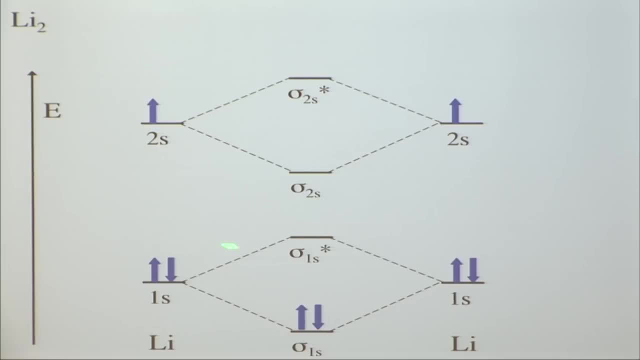 in. We're going to start with the lowest energy and move up. So we have four electrons that we need to put in. So we fill up everything here And now we go up to our 2s, The 2s orbitals. 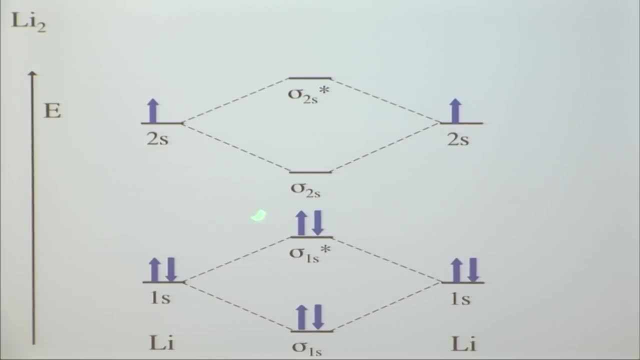 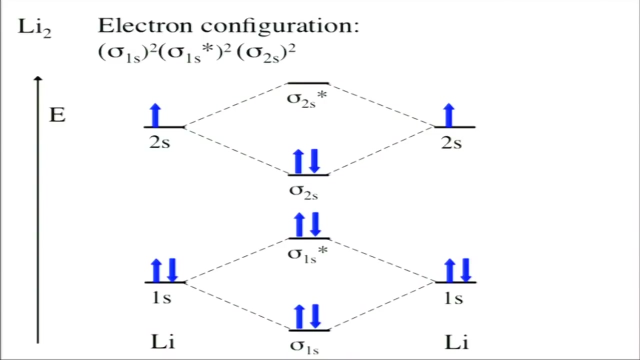 will generate sigma 2s and sigma 2s star. We have two electrons so they both can go down here. So here is what our MO diagram looks like. We can write out the electron configuration again based on this diagram. So we have two electrons in sigma 1s, So we have a 2 there. 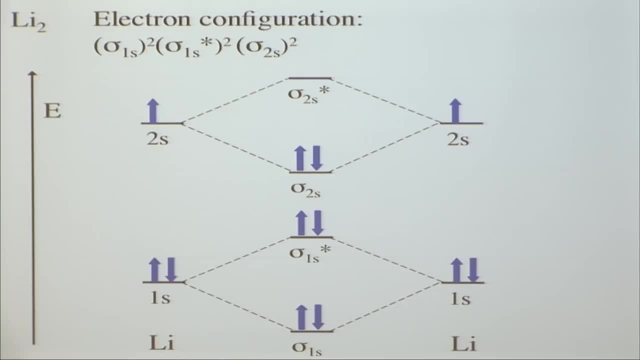 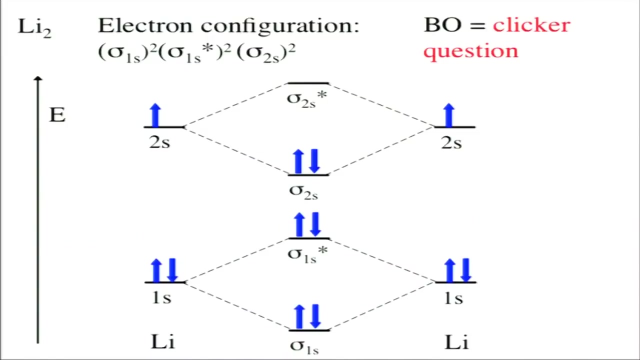 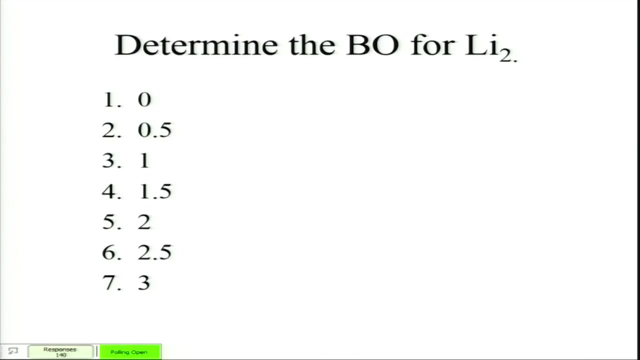 We have two electrons in sigma 1s star, our antibonding orbital, And we have two electrons in sigma 2s, And now we can calculate the bond order, which is another clicker question. OK, just 10 more seconds. 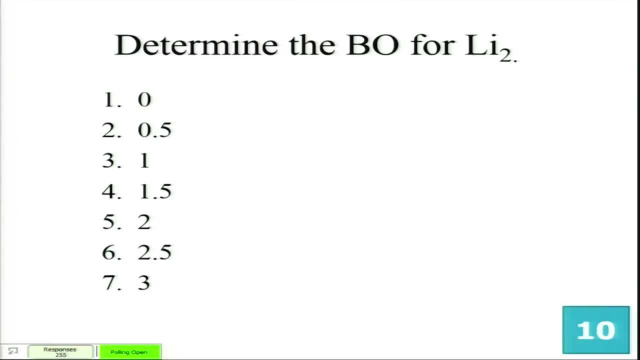 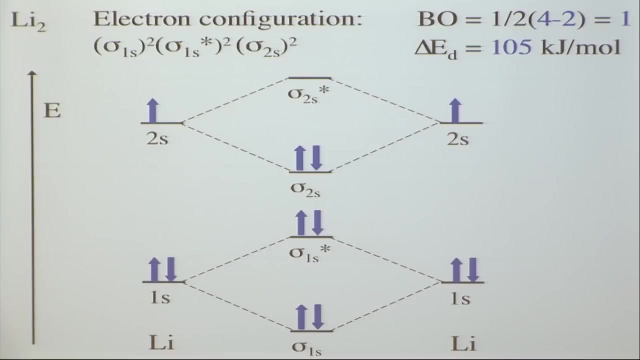 Am I right? Yeah, Yeah, You were out of time, OK, Good Thanks, Excellent 84%. So if we do out the math here, we always have our 1 half. We have four bonding electrons. We have two down here and two up here. 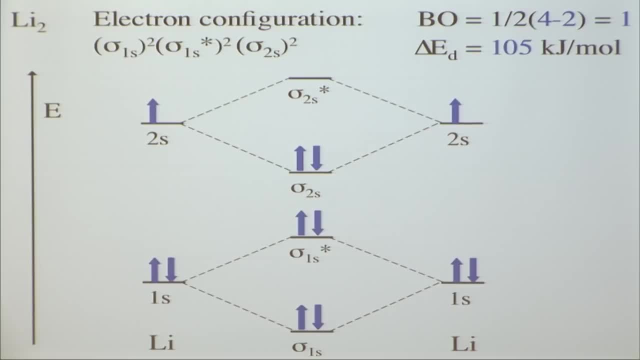 We have two antibonding electrons in our sigma 1s star, And so that gives us a bond order of 1. And in fact the dissociation energy does suggest there is a bond. It's not a great bond, It's 105 kilojoules per mole. 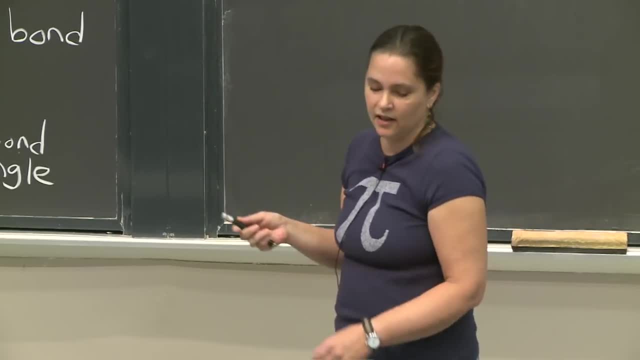 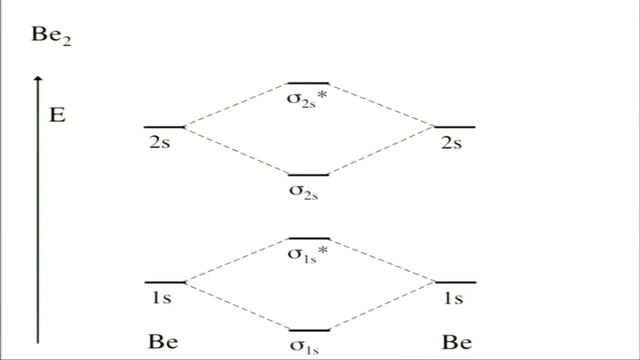 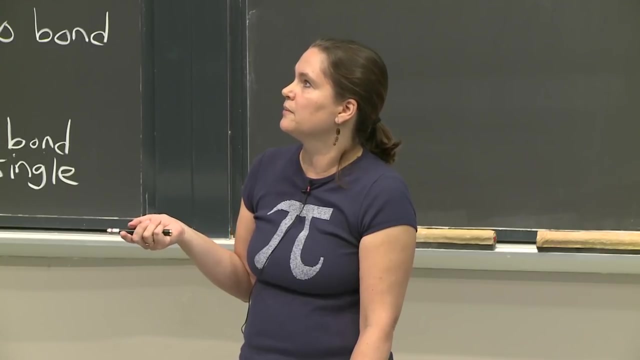 Not necessarily enough to power a starship, but still this molecule does exist. All right, So let's look at beryllium now do another example. So how many electrons is beryllium going to have? It'll have four, so we'll put those up. 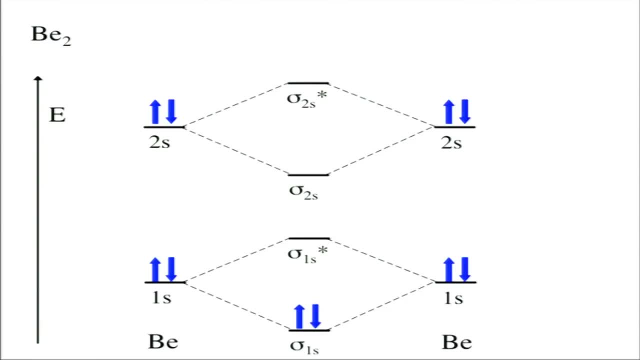 Now we're going to start with our lowest energy orbital And we're going to put some in the antibonding as well, And then we'll do this, and then we'll do that, And we filled up everything, And so we can write out our configuration. 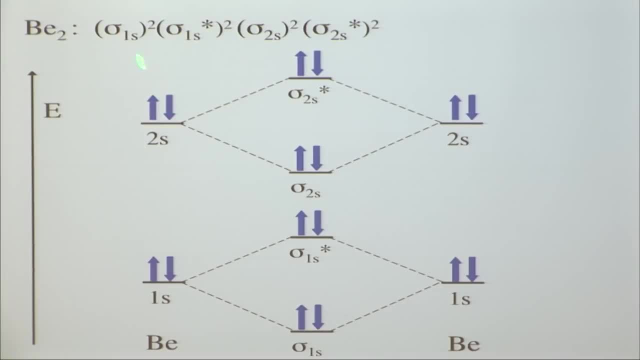 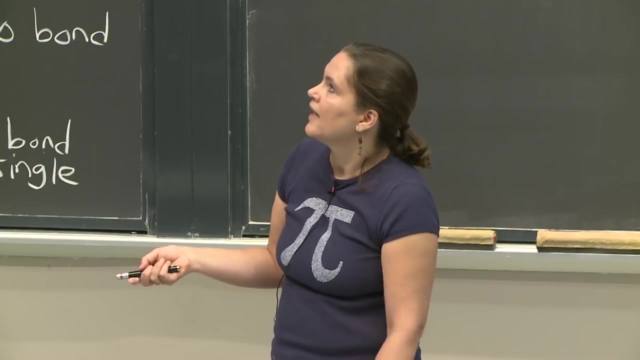 We have two in our sigma 1s orbital, We have two in our sigma 1s star, We have two in our sigma 2s and two in our sigma 2s star, Our antibonding orbital. there And now there are two different ways. 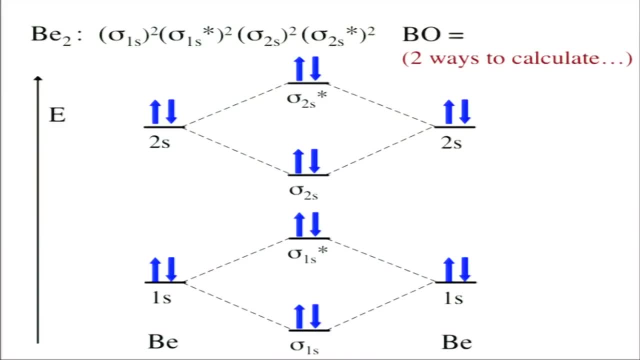 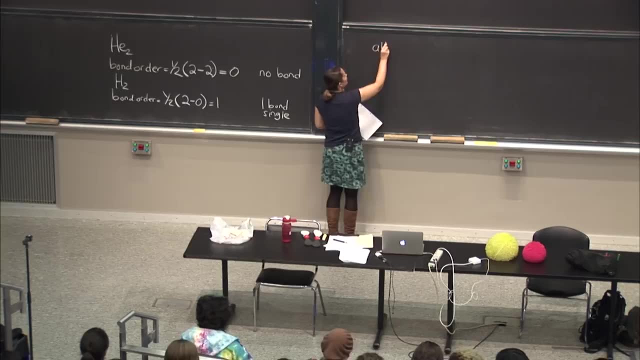 that I can calculate the bond order here, And we'll do both of them and show you that they come out the same way. One way that we can calculate this is to consider all electrons. So if we consider all electrons, our bond order 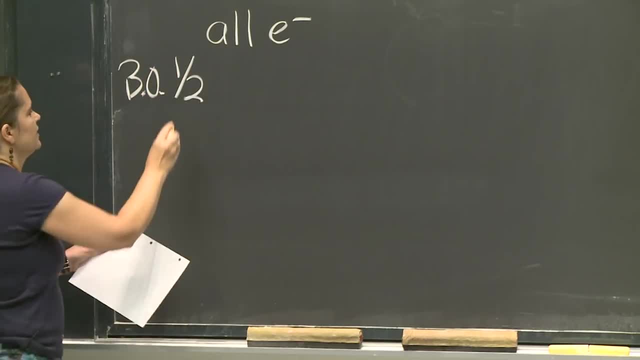 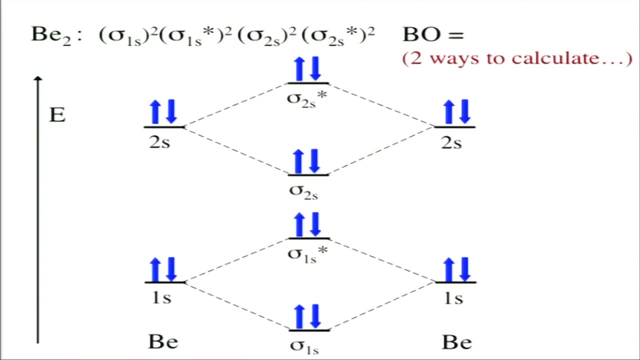 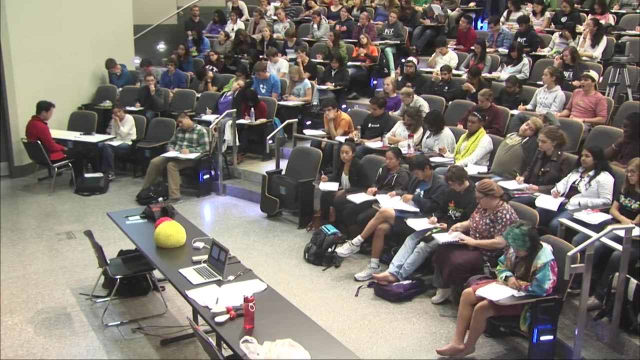 and that's often just said. B period O is 1 1⁄2 of our bonding, And now we can count up both the 1s and the 2s. So how many bonding electrons do we have? We should have four. 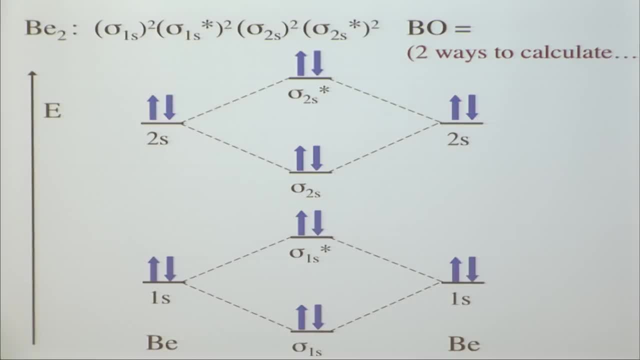 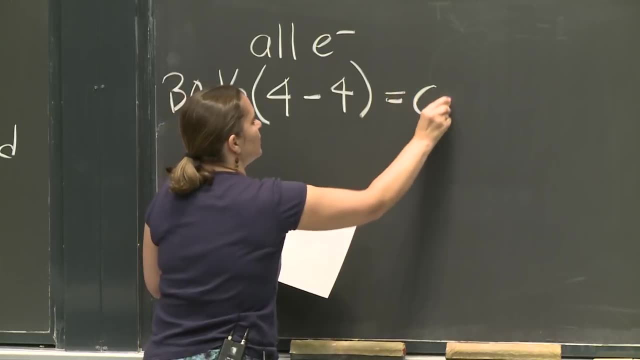 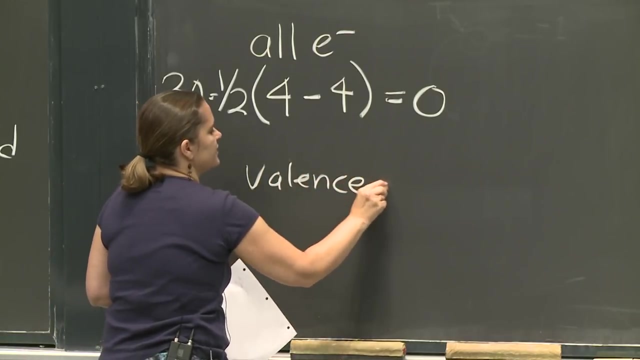 So we have two here, two here, So four. How many antibonding? Also four. So that suggests a bond order of zero. Or we could just: Let's consider our valence electrons, So that would be the electrons in 2s. 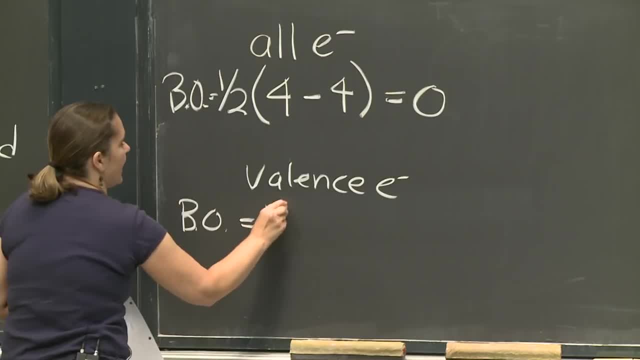 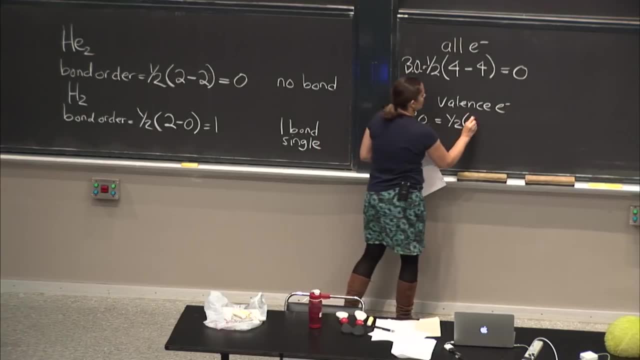 And if we do that, bond order equals 1⁄2.. It's always 1⁄2.. So how many valence electrons do we have in bonding orbitals Two? How many in antibonding orbitals Two? 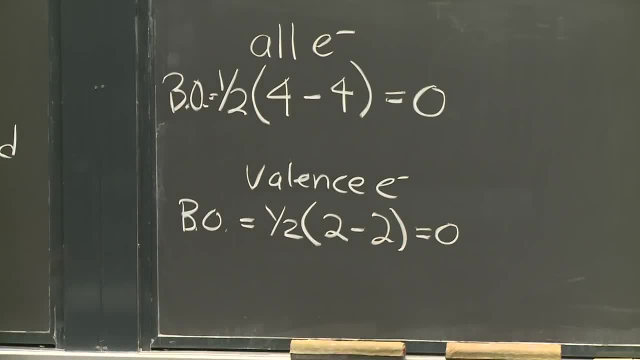 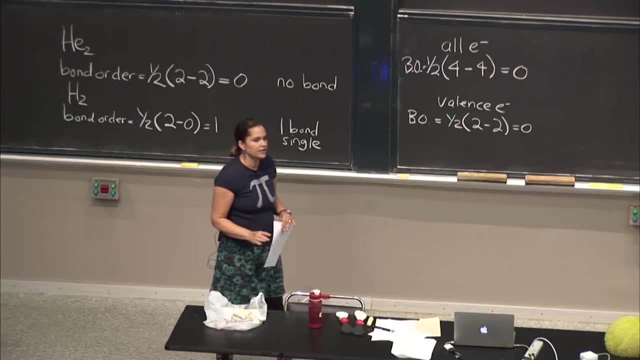 And that gives the answer of zero. So it should always work. unless you did something very strange, You should be able to do it both ways, OK, So that should work both ways and get the same answer. So if this is a complicated problem, 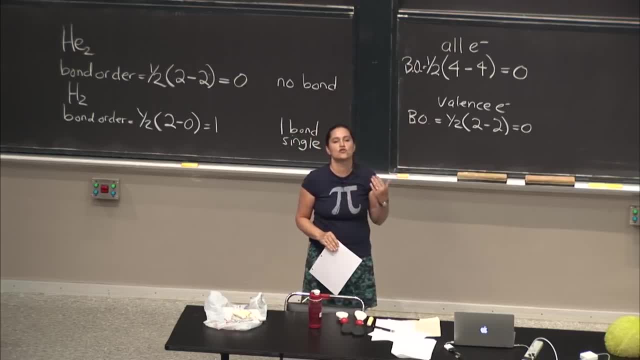 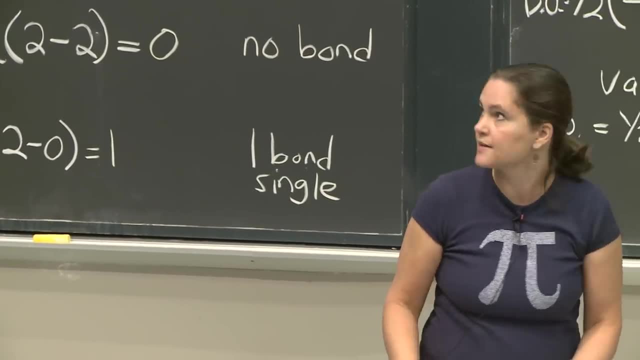 you might want to only consider the valence electrons. In fact, on a test you may only be asked to draw the molecular orbital diagrams for the valence electrons And you don't have to do the other ones. OK, So that should work both ways. 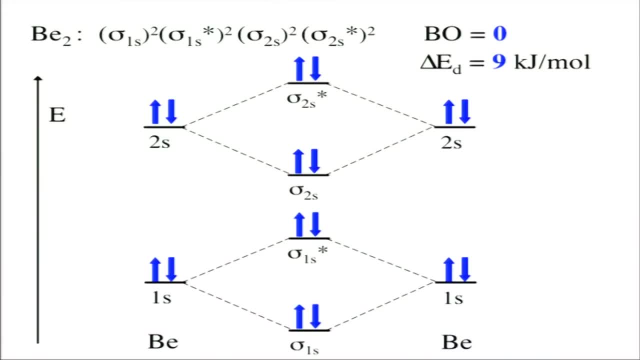 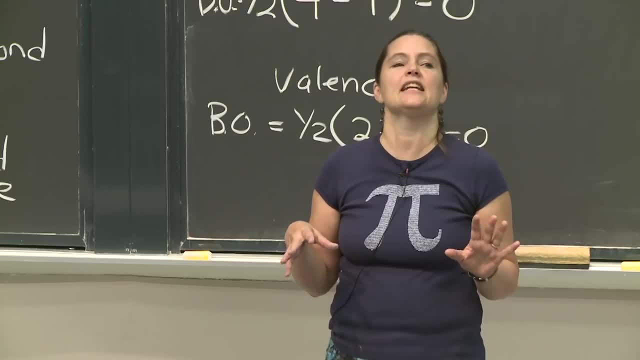 And we get a bond order of zero And in fact the dissociation energy is only 9 kilojoules per second. So it's a little stronger than dihelium, But this is an exceedingly weak molecule. So when you have the same number of electrons in bonding, 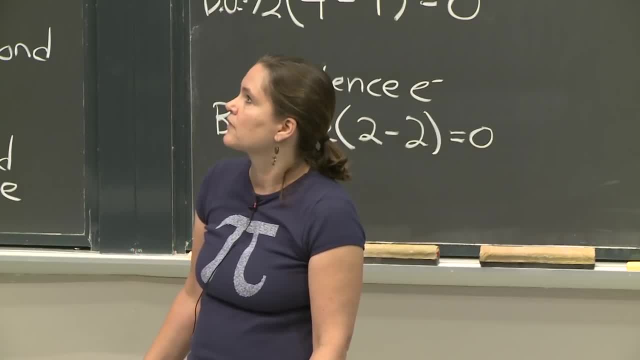 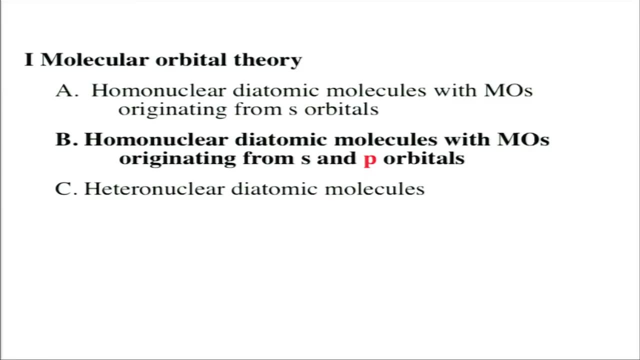 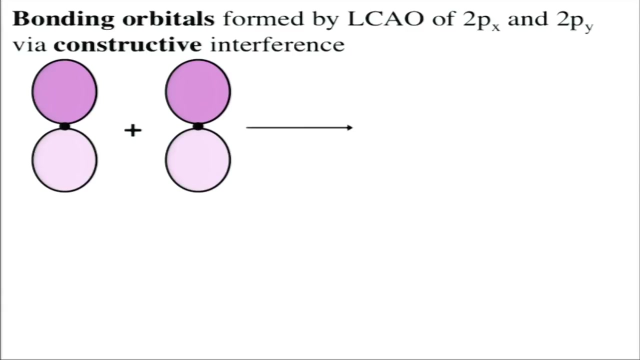 as antibonding, it doesn't lead to a very strong molecule. All right, That's the s orbitals. Now it's time for molecules that have p orbitals as well. So in this case, now I have my p orbital. 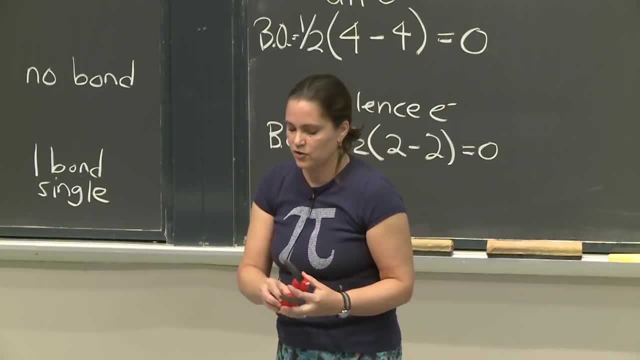 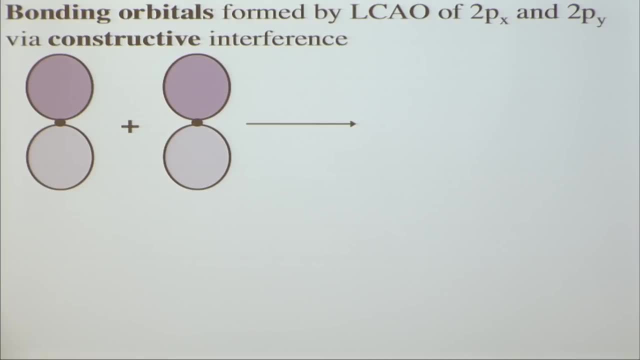 And another p orbital And we have our nuclei in the middle And we're going to bring these together And we will have constructive interference. And so here we're bringing together 2p x of a and 2p x b, or 2p y a and 2p y b. 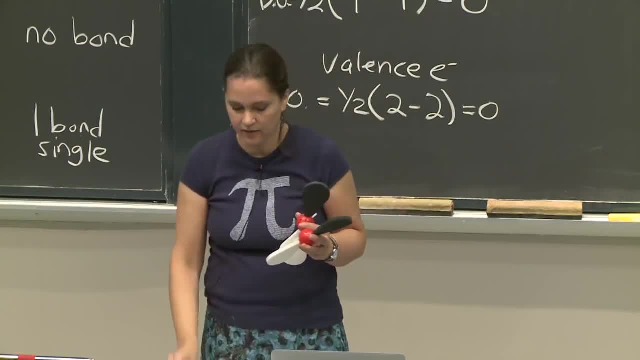 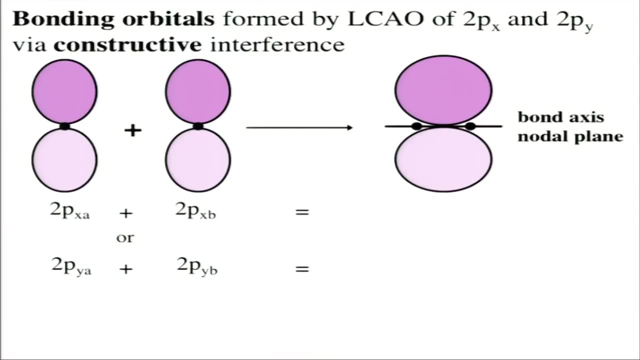 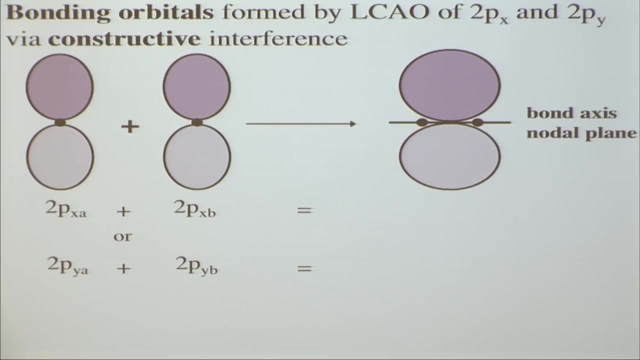 So just x and y we're considering right now. OK, OK, OK. And if we bring those together with constructive interference, then we're going to form a bonding orbital that has enhanced probability density in both cases and a nodal plane along the bond axis. 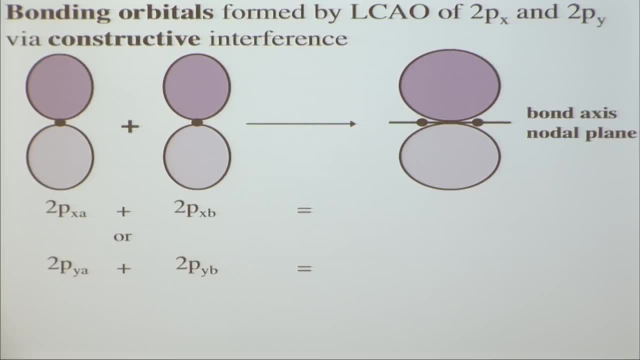 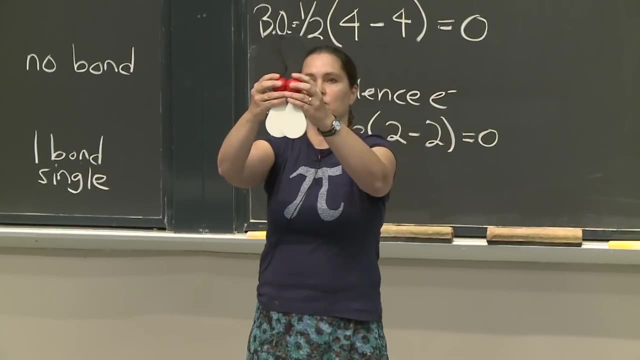 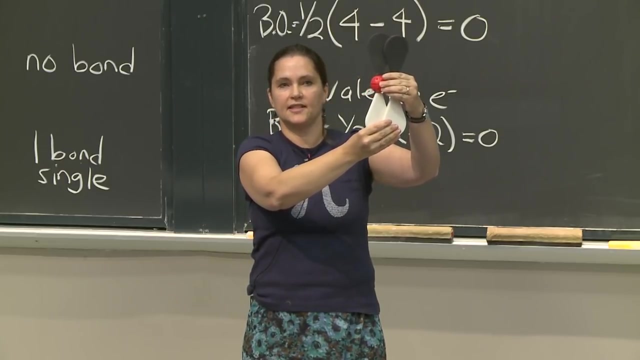 because we had nodal planes along there to begin with. So if we think about this and we have both of these, we're bringing them together and we're going to have, they're going to interfere constructively, enhance probability density here. enhance probability density. 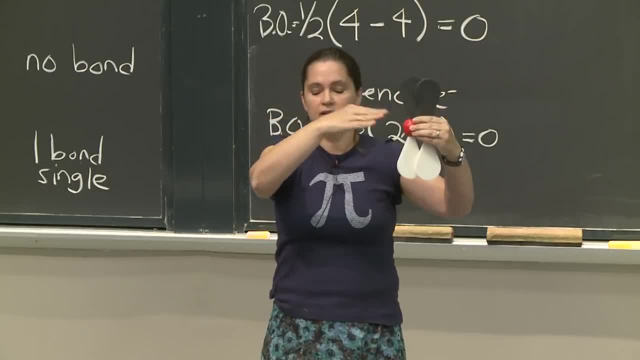 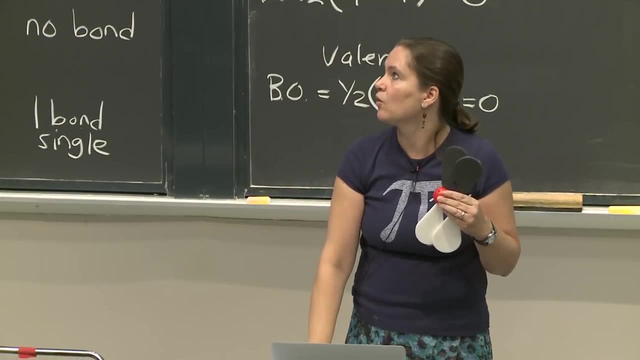 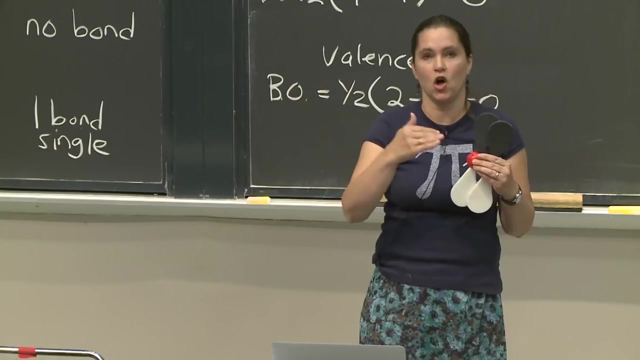 down here, but we still have our nodal plane because we started out with one, And so if we have a nodal plane, this cannot be a sigma orbital, It has to be a pi orbital, because sigma orbitals are not going to have a nodal plane along the bonding axis. 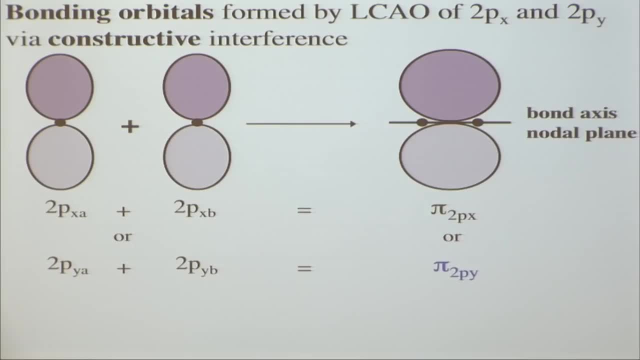 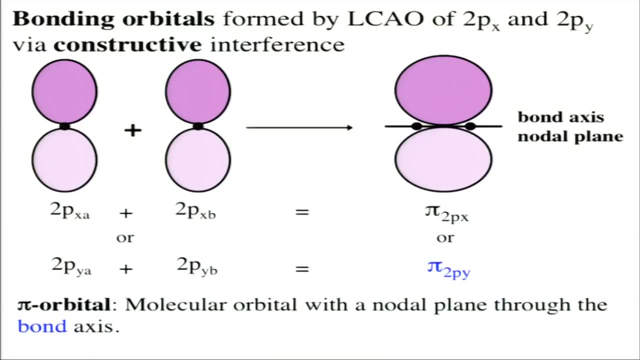 All right, So we could generate pi 2p x or pi 2p y this way. So a pi orbital is a molecular orbital that has a nodal plane through the bond axis, or maybe I should say along the bond axis. 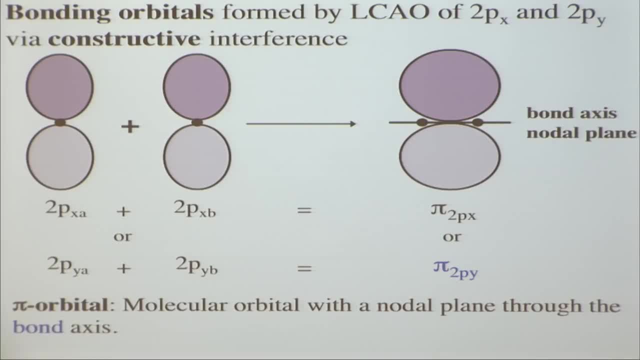 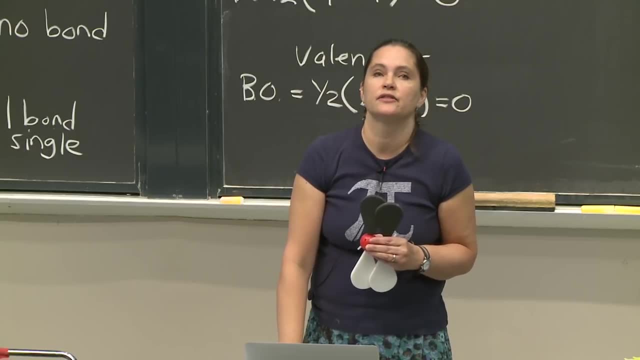 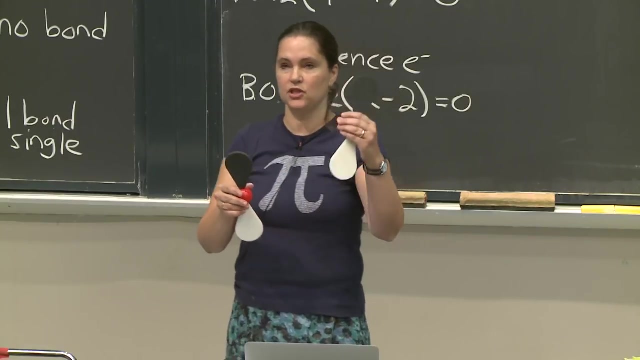 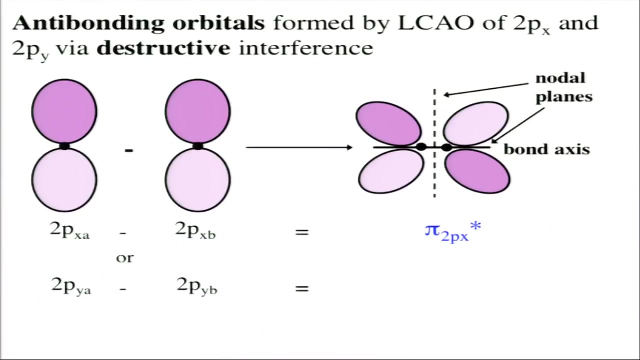 So here is our nodal plane. right through the bond axis, We can also have antibonding, which means destructive interference. So now I'm going to be subtracting one of these from one of these And I'm going to get something that looks like this: 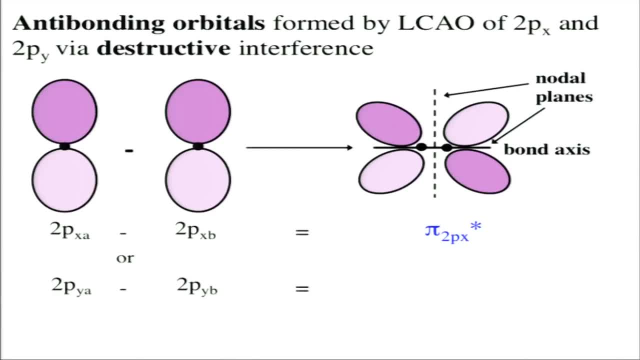 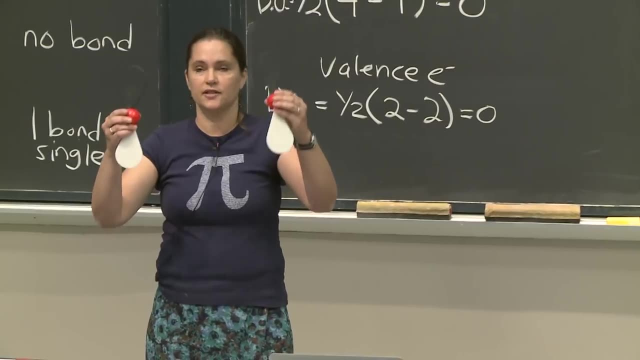 And it will be pi 2p x star or pi 2p y star And it will have two nodal planes. So let's look at this. So this is destructive interference. I'm subtracting one of these from one of these. 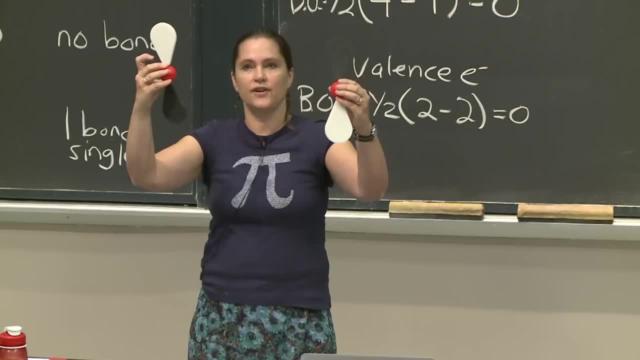 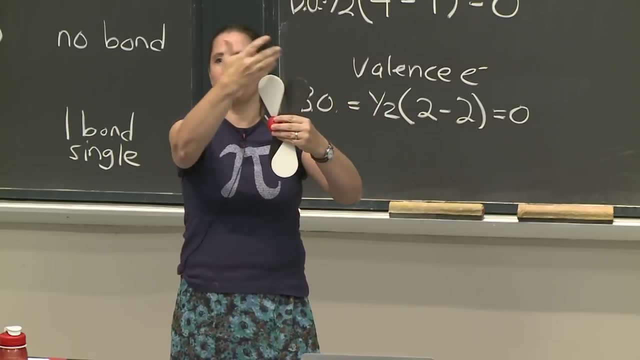 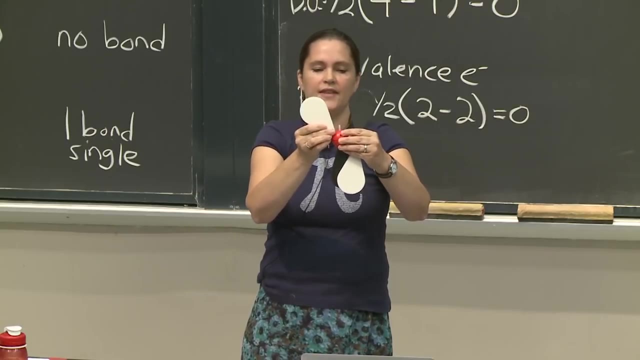 So the phase has to change. So I'm going to change the phase on one of them and then bring them together. Now we're not going to have that awesome constructive interference. increased probability density- These are negatively interacting with each other And this generates a nodal plane between the molecules. 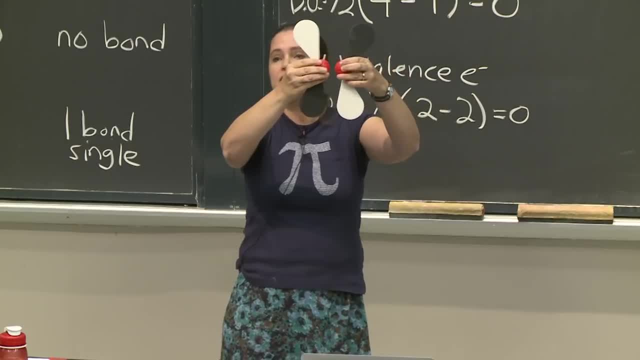 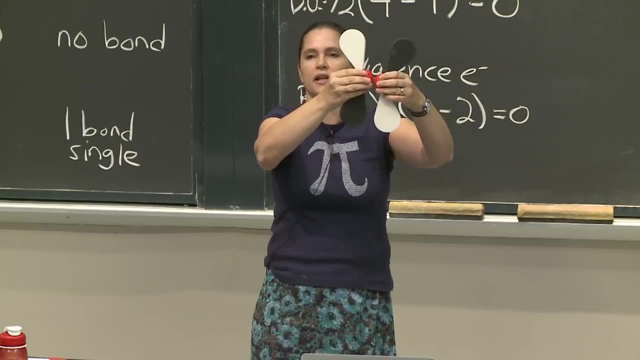 They really look much more like this now. So we have still our nodal plane through the bond. We had that before, We're always going to have that, But now we have an additional nodal plane. So we have an additional nodal plane between the nuclei. 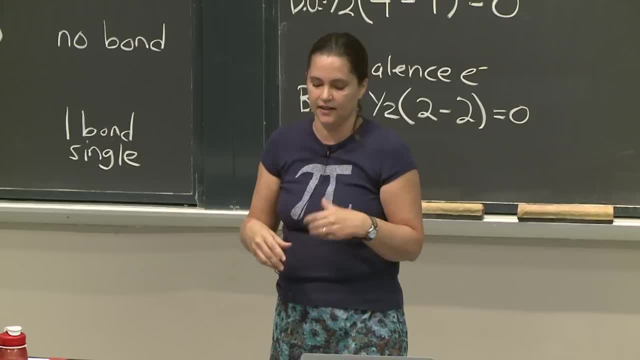 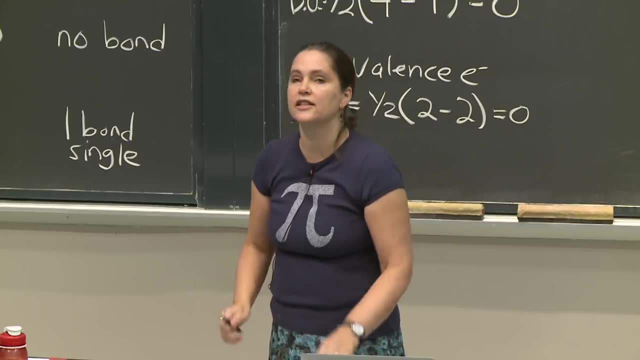 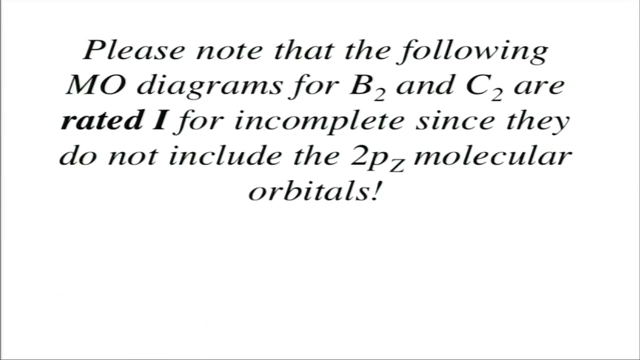 So in one case we have enhanced density, probability density again. In the other case, in antibonding, we have another nodal plane. All right, So now let's look at what happens to the energies of these pi orbitals. 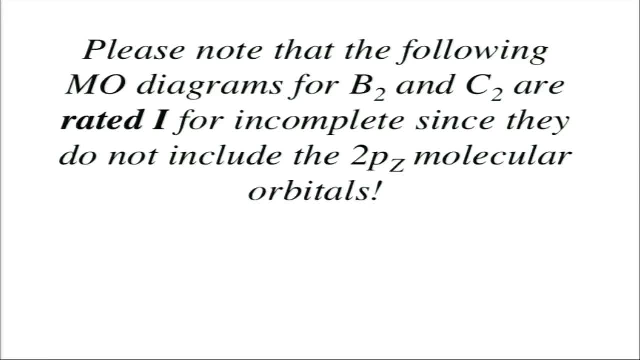 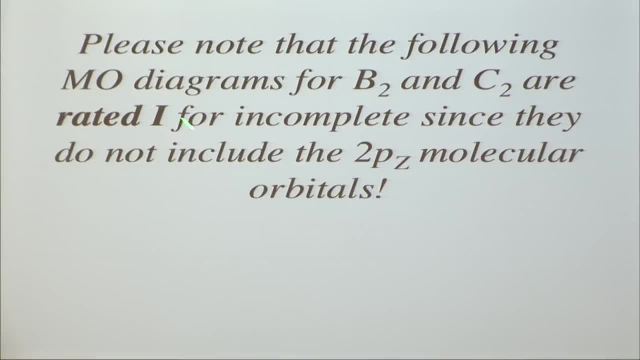 And the diagrams that I'm about to show you. we're only talking about p x and p y now. We have, for the moment, forgotten P x and P y. All right, 2pz. So these diagrams are rated. I for incomplete Warning to the viewer people. 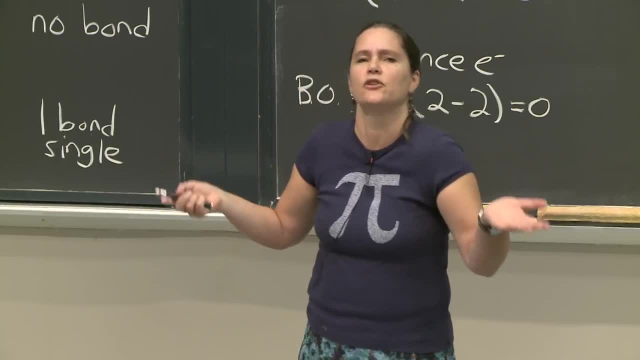 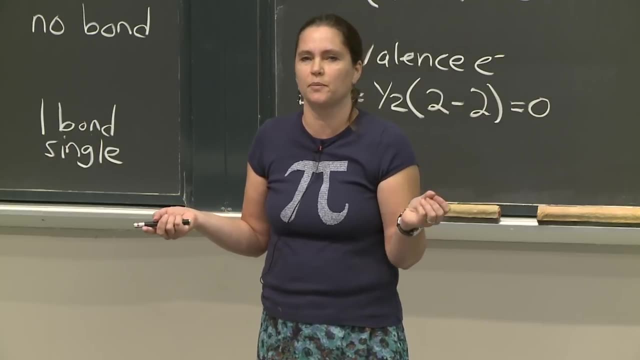 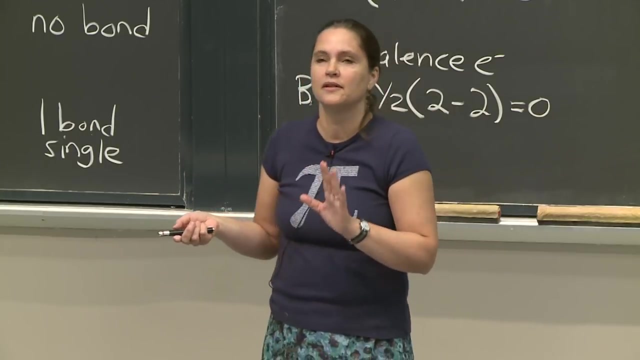 come to me and go where. where are the 2pz? Yes, they're not in these diagrams, but when you're asked for a complete diagram, you will always have to put those orbitals in and, in fact, completing these diagrams could be a question you get later. Okay, but for now we're gonna have 2pz here, but we don't have, it's not? 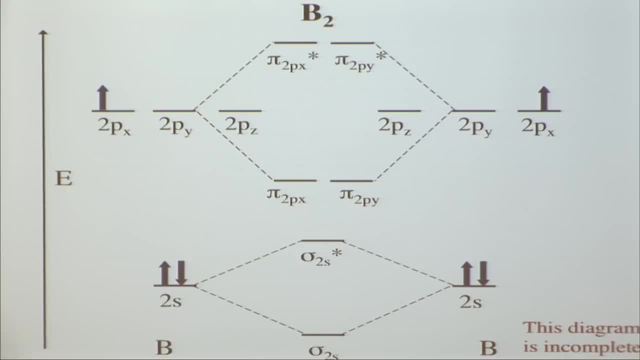 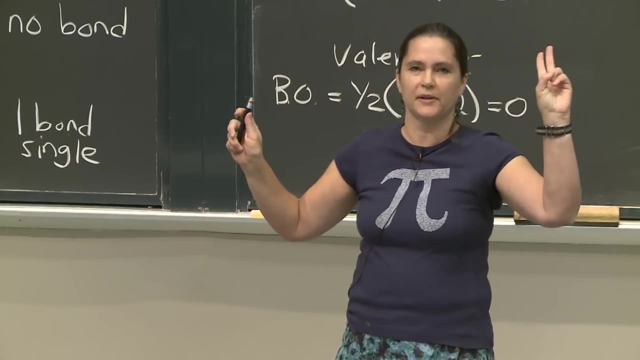 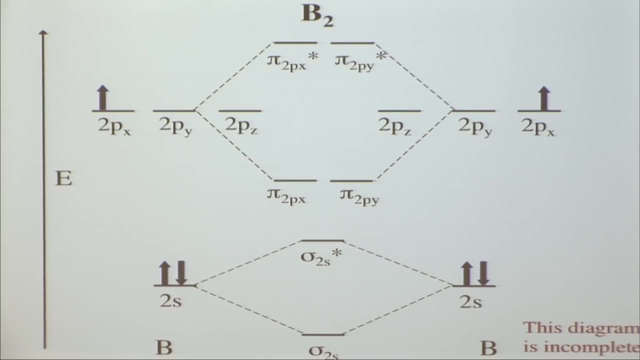 forming a molecular orbital in this diagram. This diagram is thus incomplete, but we're gonna start simple and build more complicated. So only only two p orbitals first, and then we'll add the third one, because this compound doesn't actually need that orbital. so we're good for now. All right, so we have moved on to. 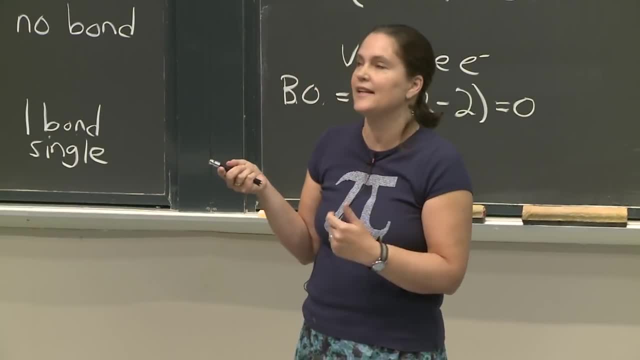 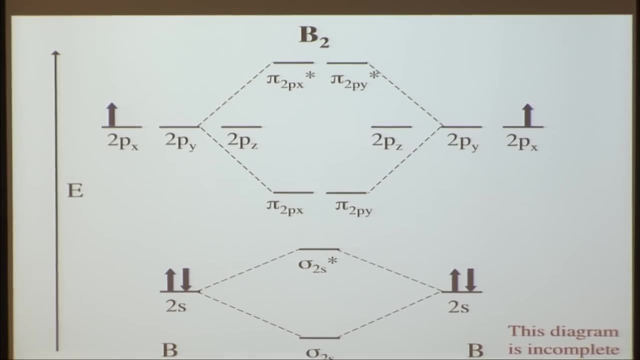 the first element that has a p electron in a p orbital. We have boron and we have two of them. So we have boron and we have two of them. So we have boron and we have two of them. So now I dropped off 1s to simplify this. So we're starting just with now. we just 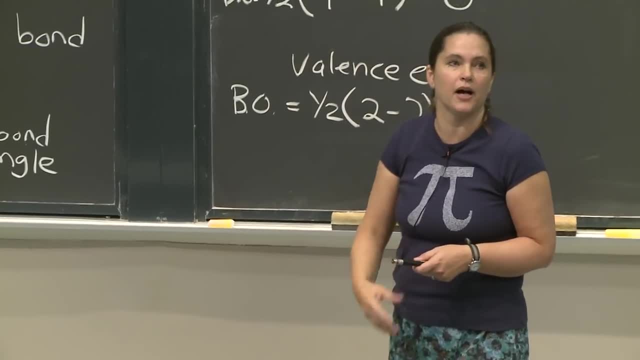 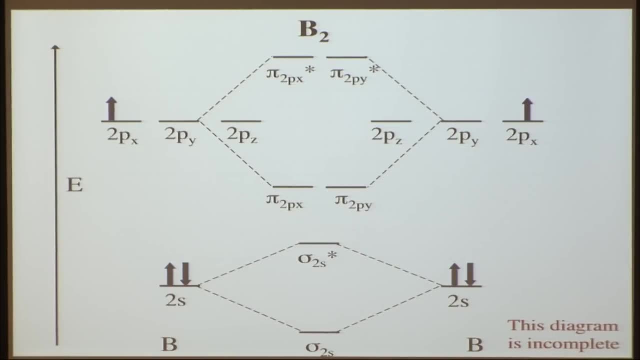 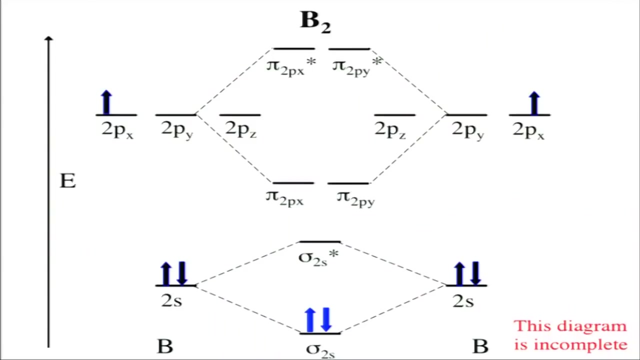 have our valence electrons, So it's a good thing we can calculate bond order just using our valence electrons. All right, so we have 2 in 2s and 1 in 2px or 2py- I could have put it either place. So let's put in where they would go. So we 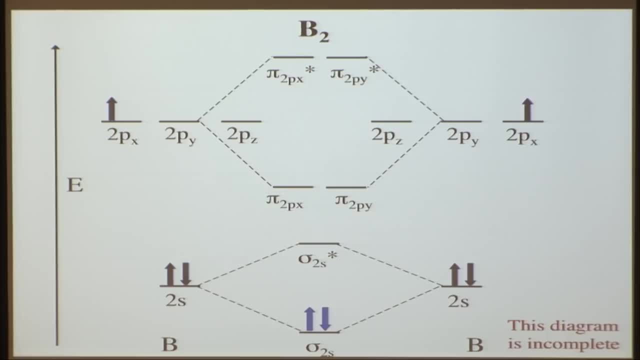 have 2s orbitals, they'll form, go into bonding. So we're putting sigma 2s first, Then into anti-bonding sigma 2s star, And now we have p electrons and we're going to put them into our pi orbitals, our molecular orbitals. I'll 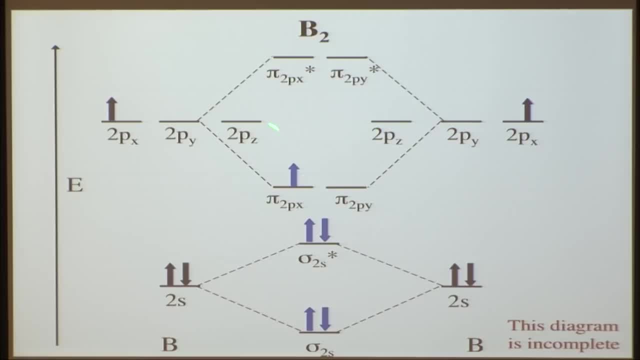 put one in, And where am I going to put the other one? Am I going to put it next to it or over here? What do I think? Yeah, so we're going to do that because, again, when you're going to sit on the bus, you're. 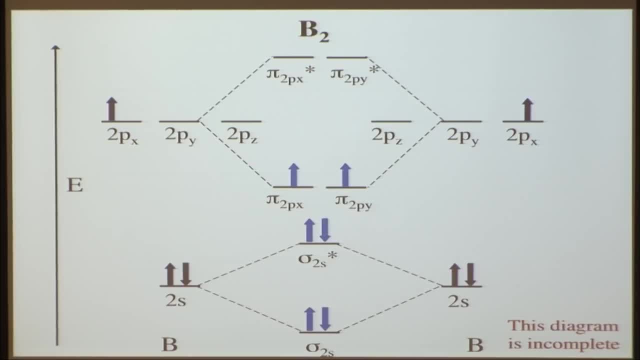 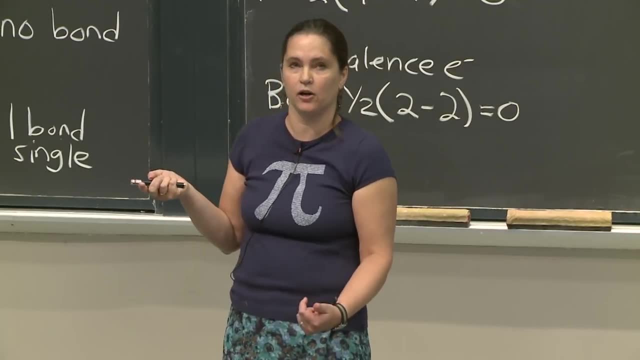 You want to have. if they're degenerate in energy levels as they are here, you're always going to put one electron in each orbital of the same energy first before you pair them up, And they'll have parallel spins. So we're reviewing things we learned before. 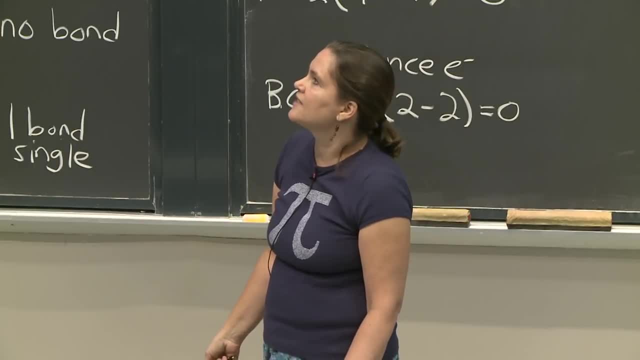 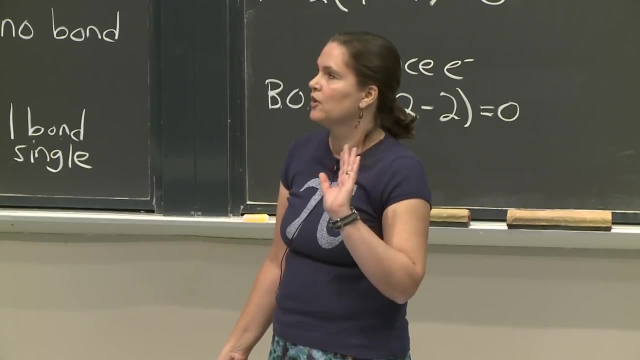 I love doing that. OK, so now let's see what our electron configuration is. And this is just the valence electron configuration. We're simplifying, We're not going to consider the 1s orbital, And we can write this down. 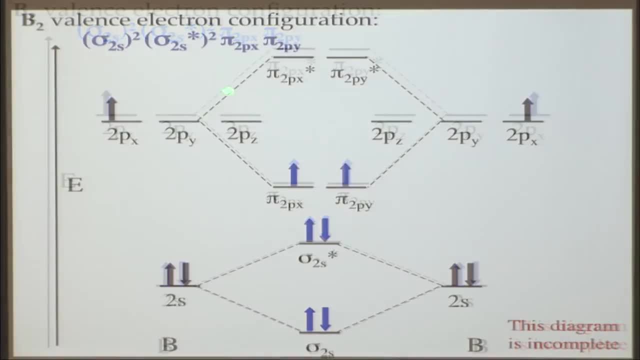 So we have two electrons in sigma 2s And we have two electrons in sigma 2s star, our antibonding orbital, And we have one in pi 2px and one in pi 2py And I can put a 1 or not put a 1.. 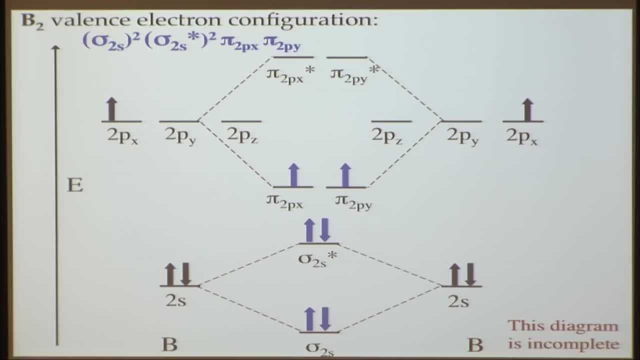 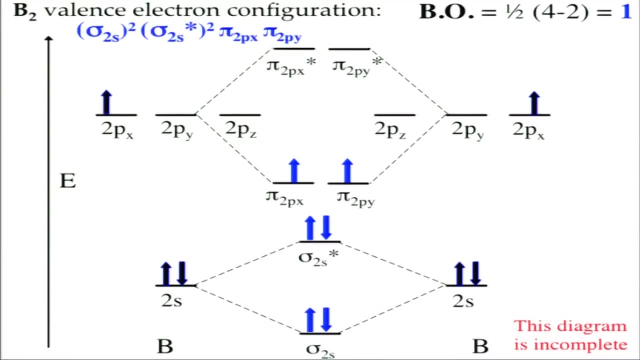 If I don't put anything for a 1,, 1 is assumed And we can calculate. We can calculate our bond order as well. So we have half, And again we're just using our valence electrons. but that's OK. 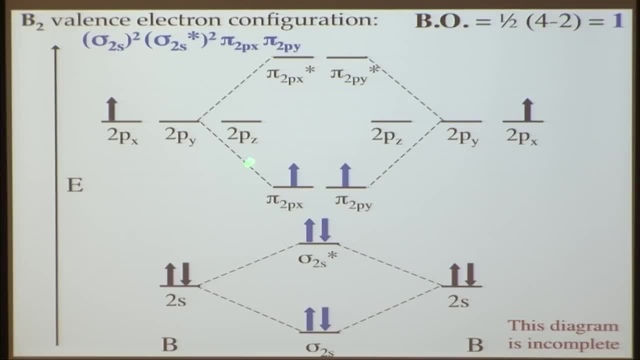 We have four now who are bonding: two down here, two up here. These are bonding orbitals And we have two that are antibonding And notice for our pi orbitals- this is what we saw before- bonding or lower in energy. 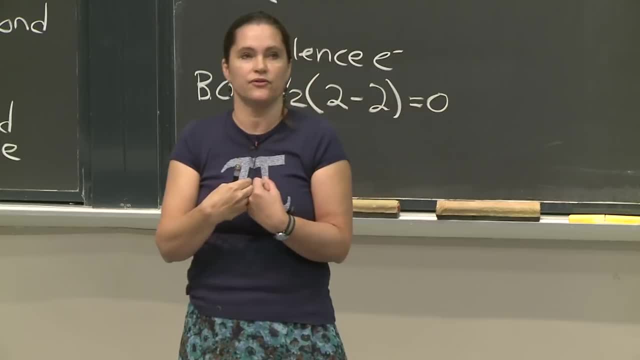 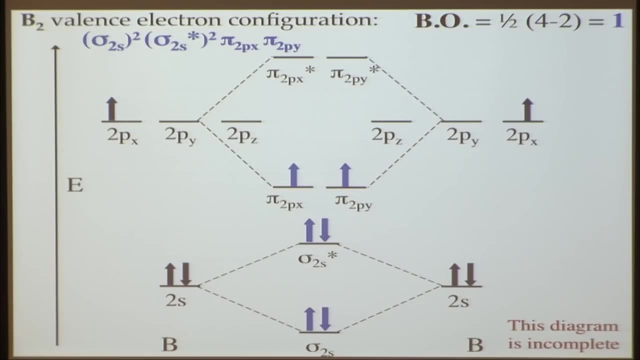 antibonding or higher in energy. With the bonding orbitals we had constructive interference probability of the electrons near the nuclei And so that's lower in energy. But in our antibonding ones we have a nodal plane in between our nuclei. 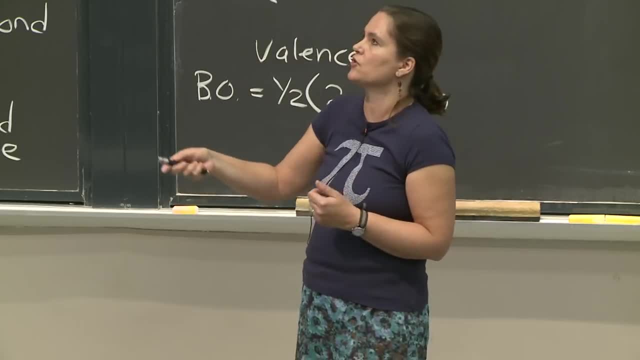 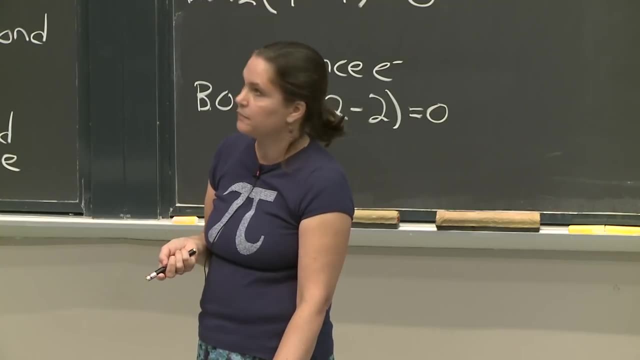 So we don't have any probability that electrons are right in between there, because there's a nodal plane, So those are higher in energy. OK, so here is our B2 diagram. So now let's try the same thing for carbon C2.. 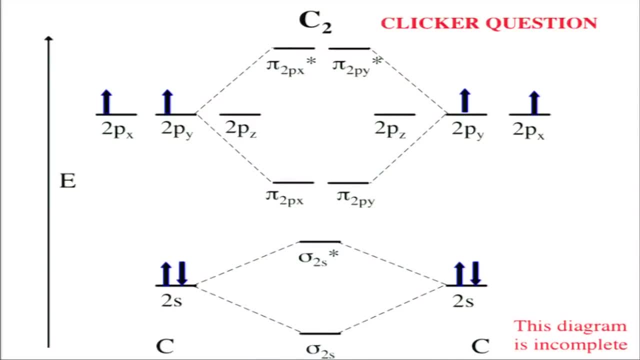 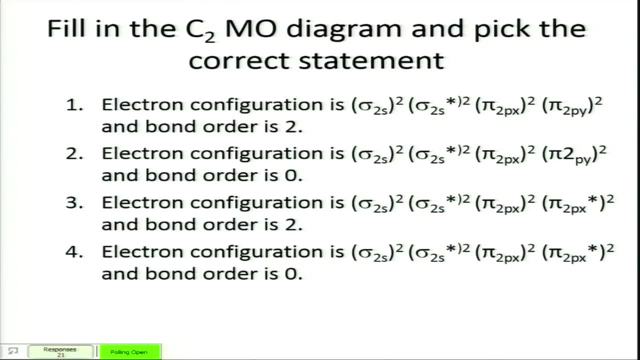 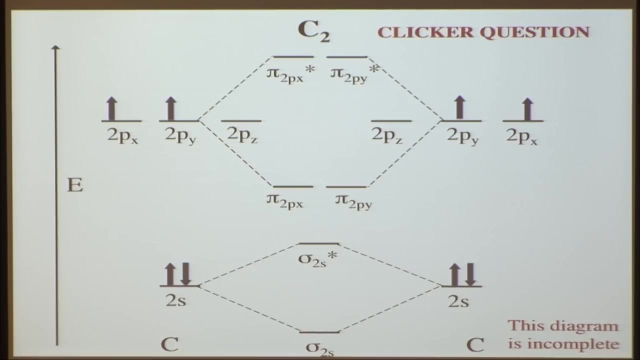 And that is a clicker question. OK, All right, let's just take 10 more seconds. OK, So let's take a look at that over here. The easiest thing to do to answer this question was to fill in the diagram in your handout. 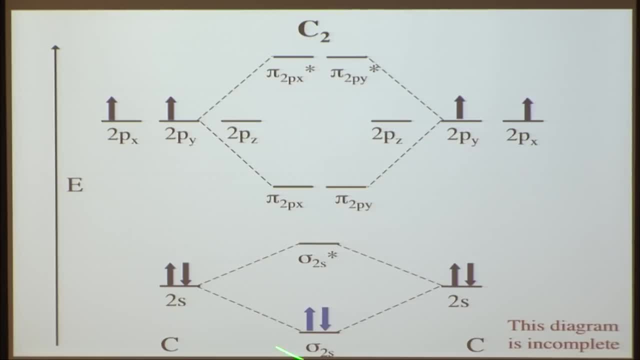 And so if you did that, you would have put 2 down here and you would have put 2 up here. Then you would have put one here, one there, another one there and another one there. OK, So now we have used these up. 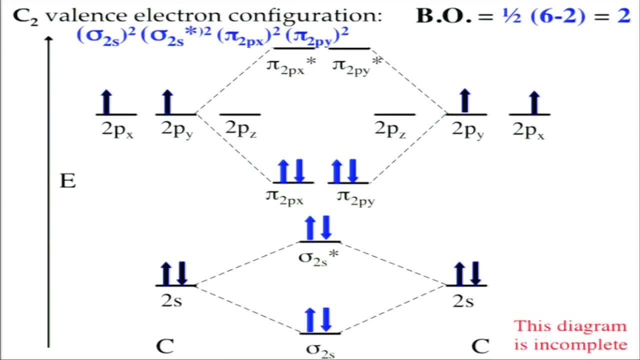 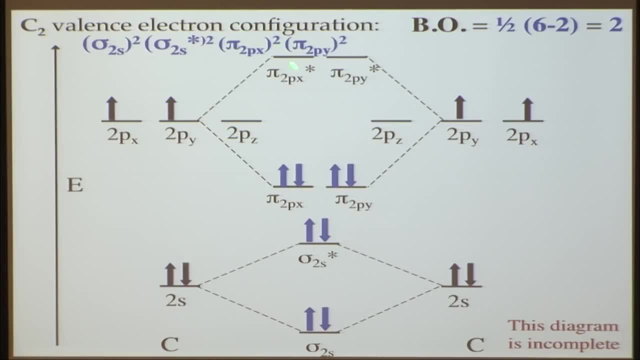 And so our configuration is sigma 2s2, sigma star 2, pi 2px2, pi 2py2.. And the bond order is 1 half. There are 6 bonding electrons: 1,, 2,, 3,, 4,, 5,, 6, and 2 antibonding electrons. 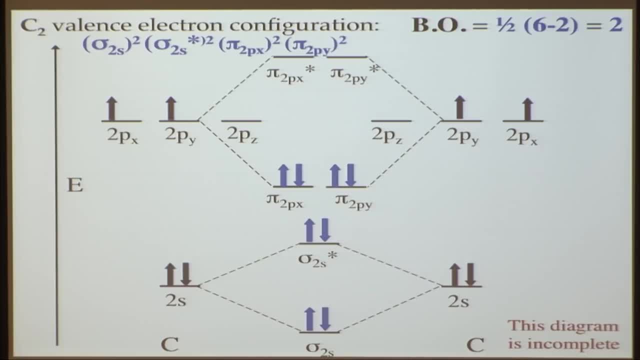 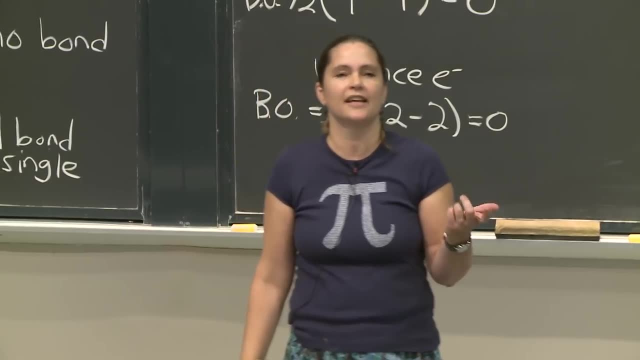 And so that adds up to a bond order of 2.. And so sometimes on a test there will be a simple question: what is the bond order? But to get there you have to draw your whole molecular orbital diagram and figure out how. 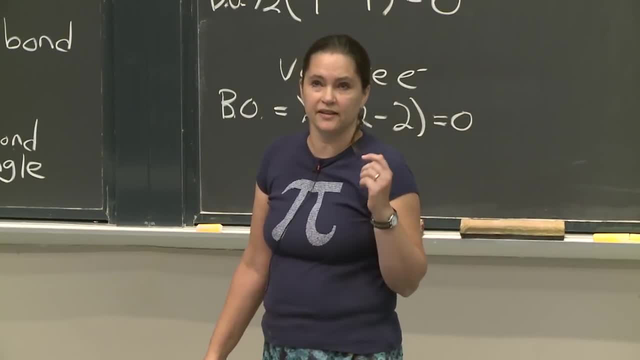 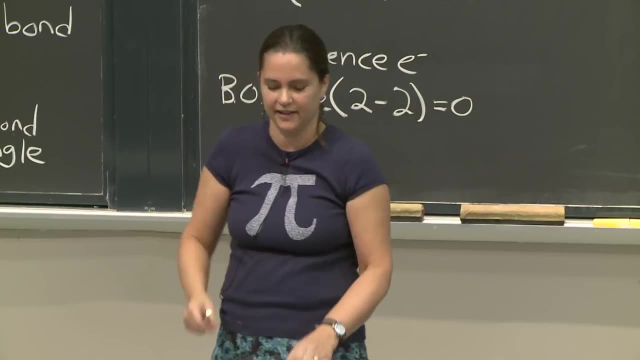 many bonding and how many antibonding? OK, These are not really that fast questions And it's nice Sometimes we give you a little space and you see this whole little molecular orbital diagram fit in there to answer the question, All right. 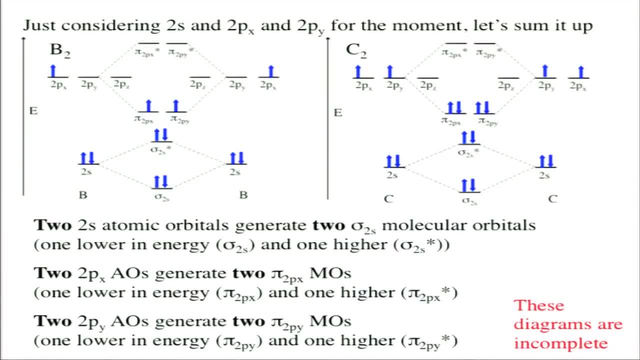 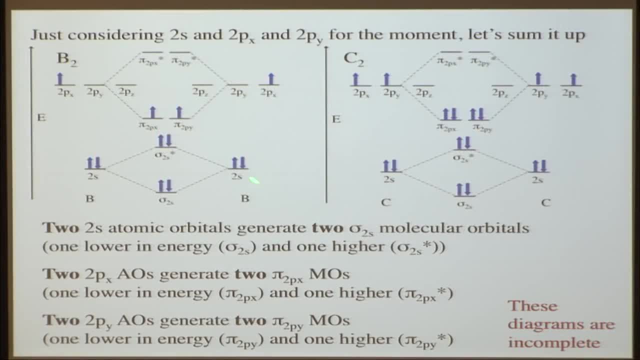 So let's just compare these two diagrams for a minute. So in both cases we had 2s orbitals, 2 atomic orbitals for 2s, And they both generated 2 molecular orbitals, a bonding and an antibonding. 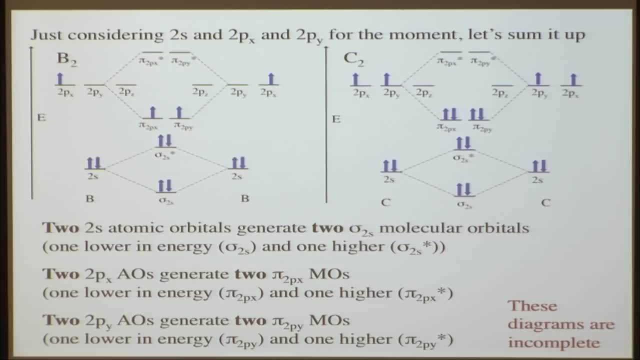 The bonding is lower And energy and the antibonding is higher in energy. We also had 2 2px atomic orbitals. They generated 2 pi 2px orbitals, 1 bonding, 1 antibonding, And the same for our 2 atomic orbitals for 2py. 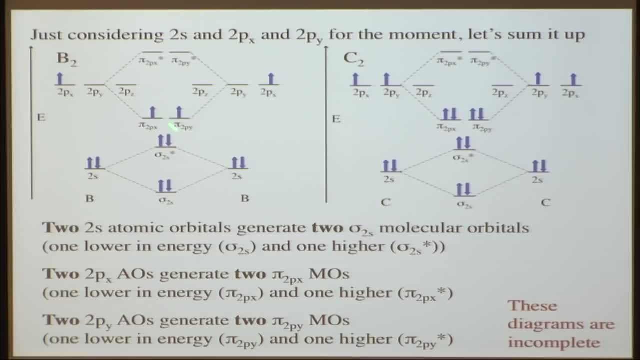 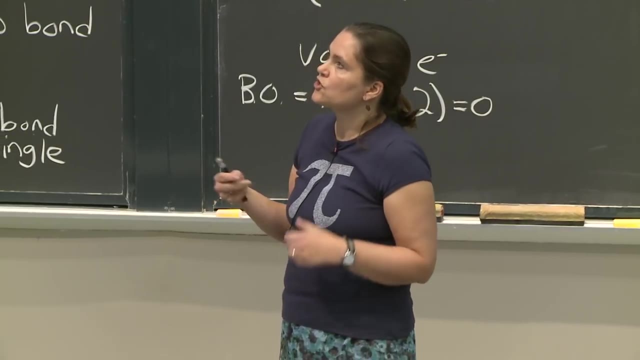 We had two of those And they generated 1 lower energy bonding pi bonding and 1 pi star Anti-bonding. So you always have n atomic orbitals generating n molecular orbitals. So the stability of the resulting molecules in these cases depend on how many of the electrons 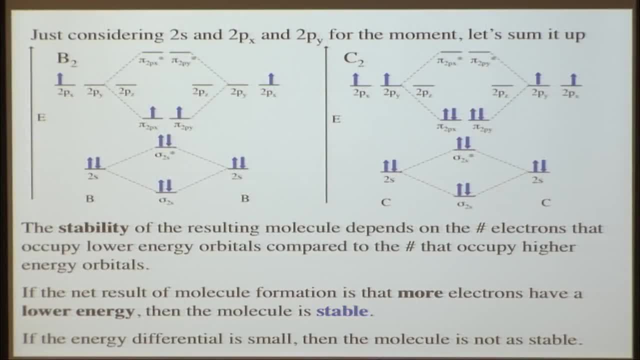 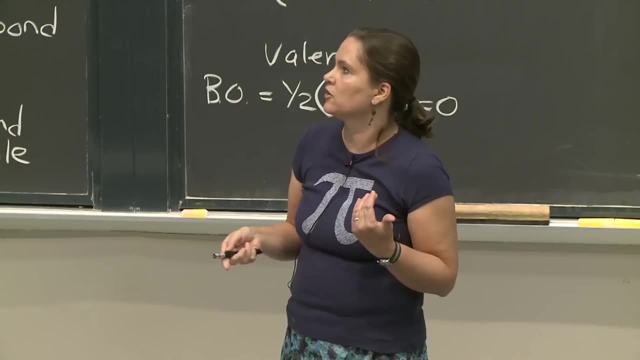 are bonding, how many are in lower energy as a result of formation of the molecule and how many are at higher energy as a result of formation of the molecule. And if the net result are more electrons than the molecules, then you're going to have a 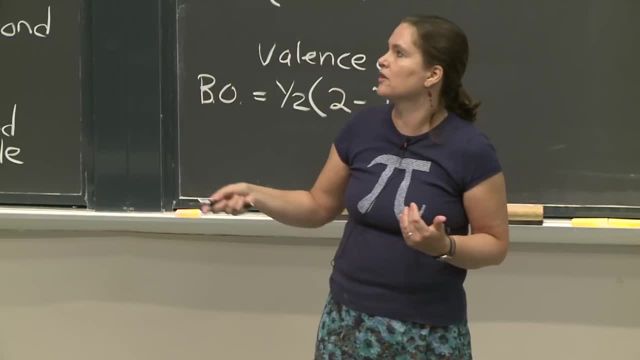 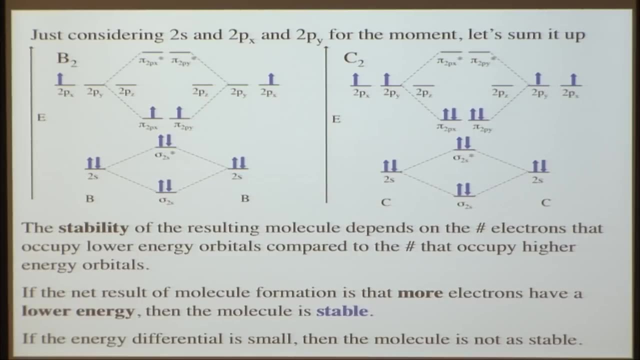 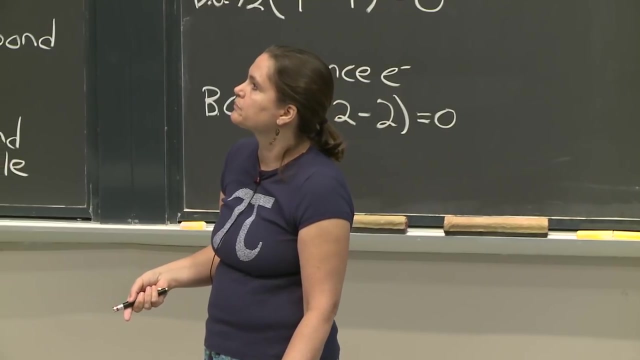 more stable molecule. If there are more electrons in lower energy, more electrons in bonding orbitals, then that molecule is more stable. If there's a very slight or kind of no difference, then that's not a very stable molecule. So now let's just compare these two and think about which of these is going to be more stable. 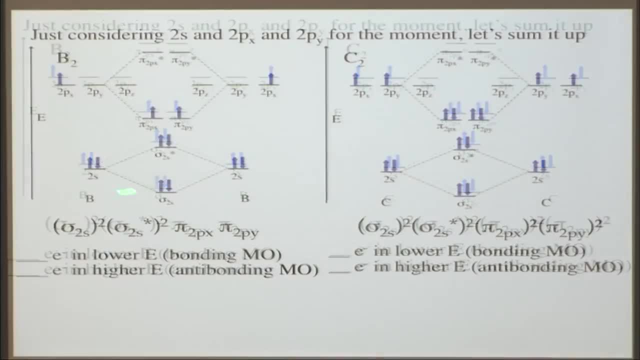 So we have our configurations again. So in the case of B2, how many electrons are in lower energy or bonding orbitals? 1. Yeah, We have 4.. 1,, 2,, 3,, 4.. How many in higher? 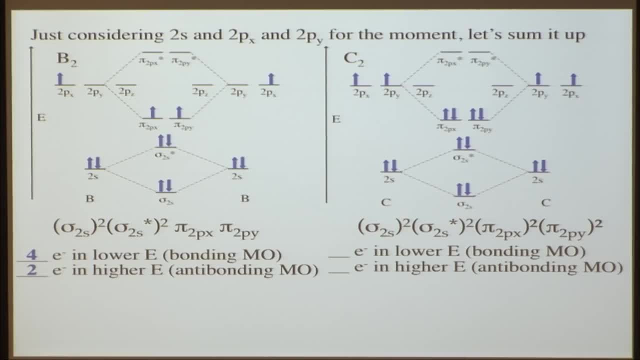 2. 2 up here 4 carbon, We had 6. 1,, 2,, 3,, 4,, 5,, 6. 2 in higher, And so the bond order here was 1.. The bond order here was 2.. 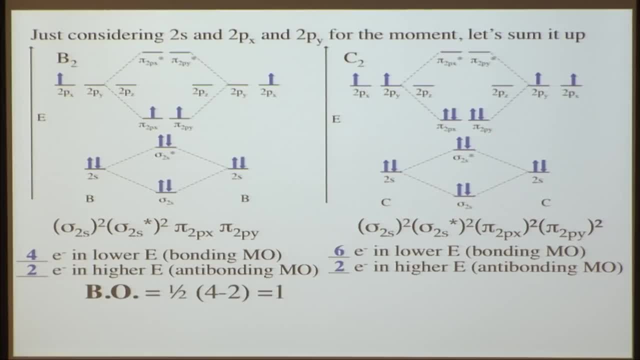 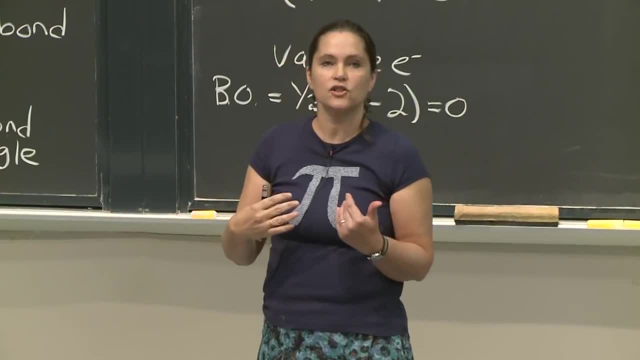 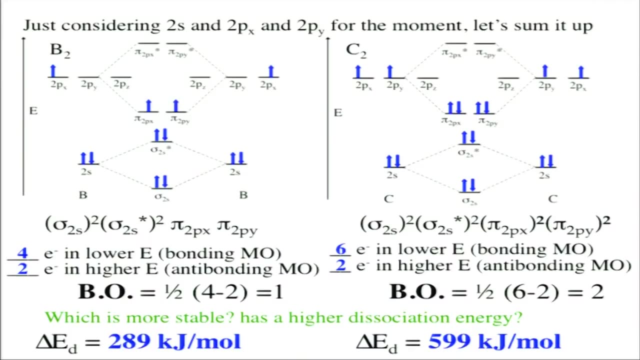 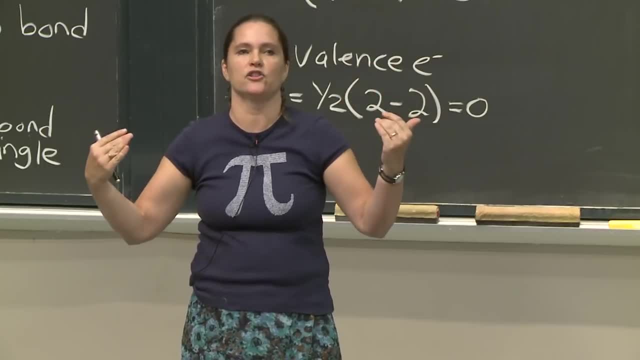 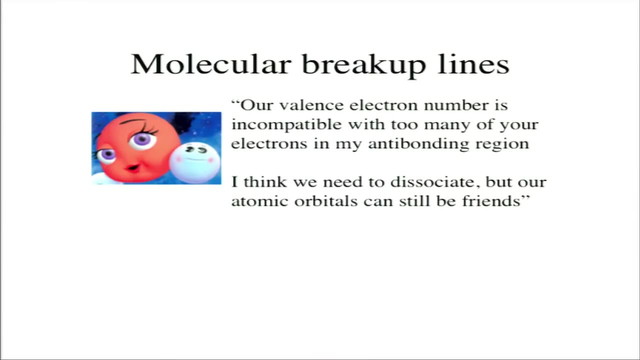 of their electrons are in antibonding or higher energy. that's not a happy molecule. So I'll just end with one way to think about this In this cartoon: molecular breakup lines. sometimes two atoms just have an incompatible number of valence electrons. 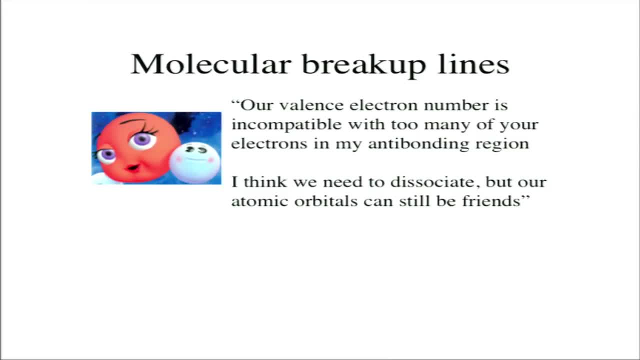 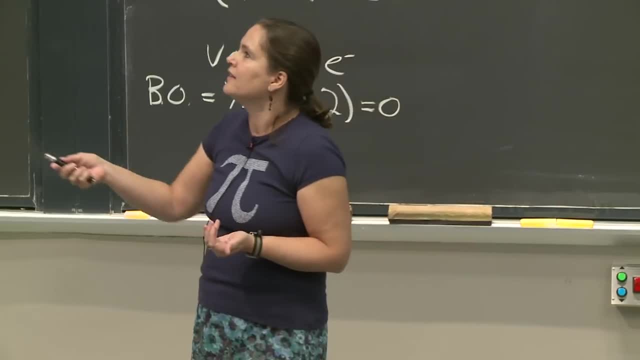 And there are just too many. You just hear this molecule saying: I'm sorry, too many of your electrons are in my antibonding regions. I don't know how many times we've all heard that, But it's time to dissociate. 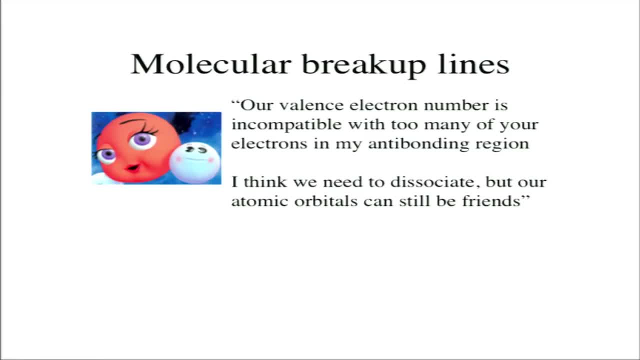 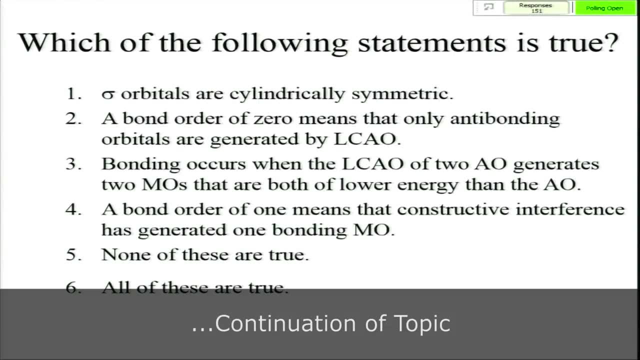 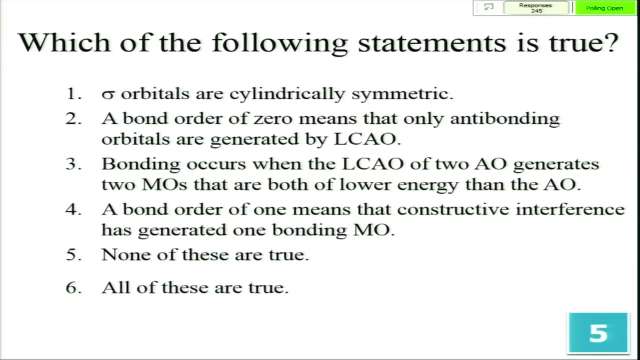 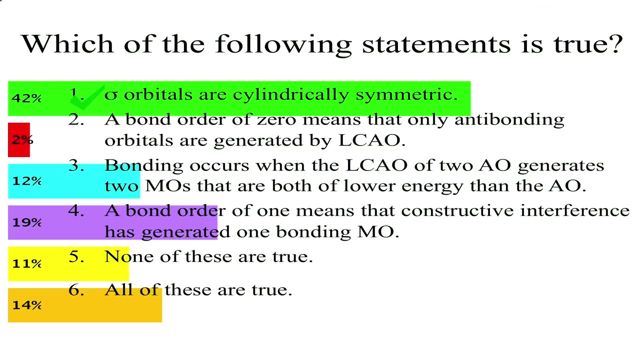 But our atomic orbitals well, they can still be friends. OK, see you on Wednesday. Take a look at the clicker question. All right, let's just take 10 more seconds. All right, let's just go through this. 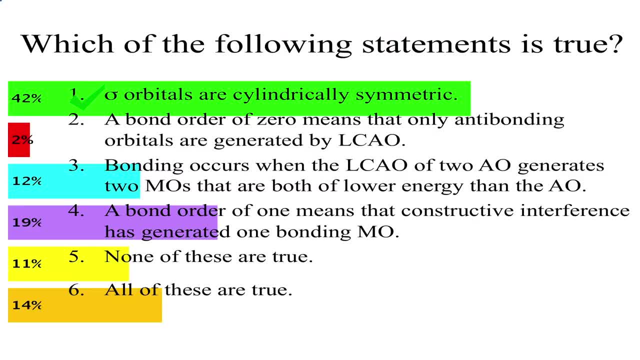 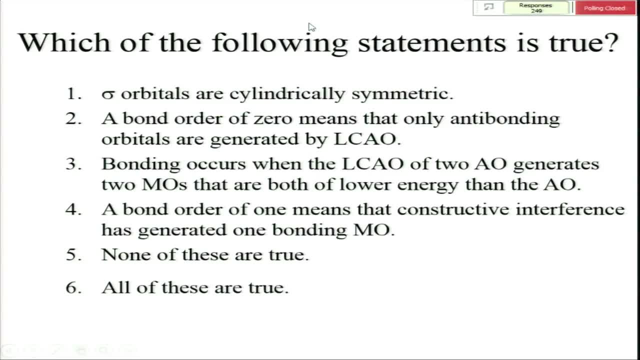 OK, Let's just go through this one. So this is a review of where we were last time, But so the correct answer is 1. So sigma orbitals are cylindrically symmetrical. Let's quiet down a minute, You can hear the answer. 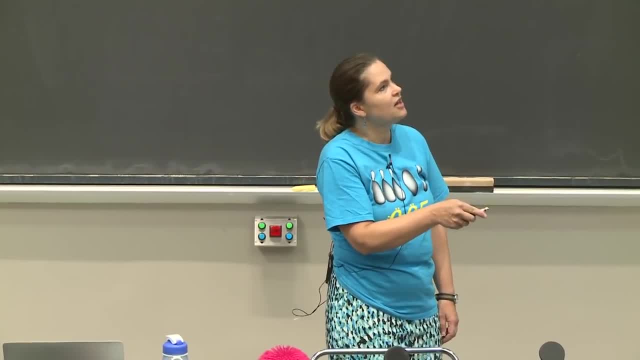 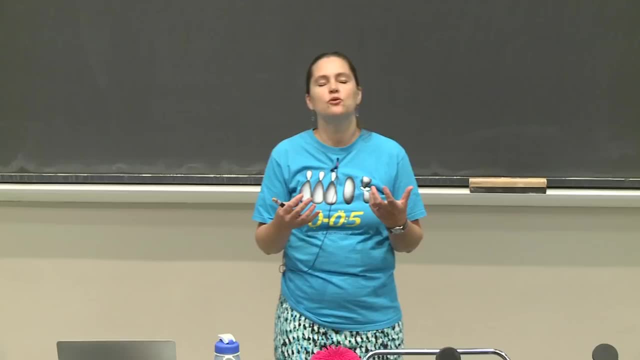 So this one is true. The second one is not true. A bond order of 0 doesn't mean 0. It doesn't mean that you just have antibonding orbitals. Whenever you bring together two atomic orbitals, you have to make two molecular orbitals. 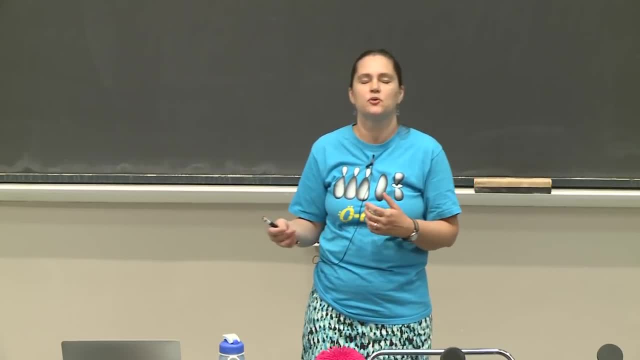 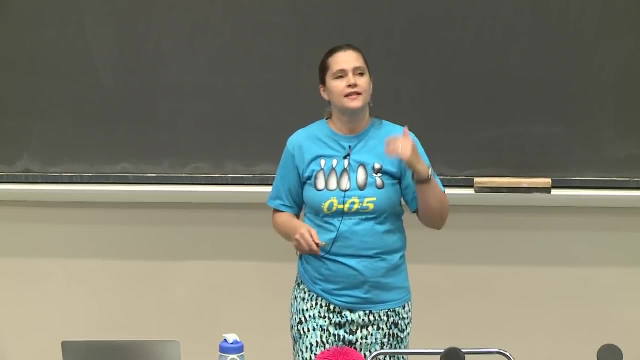 So it isn't that sometimes you make bonding orbitals and sometimes you make antibonding orbitals. Every time you bring together two atomic orbitals, you make two molecular orbitals, One that's lower in energy and that's the bonding orbital. 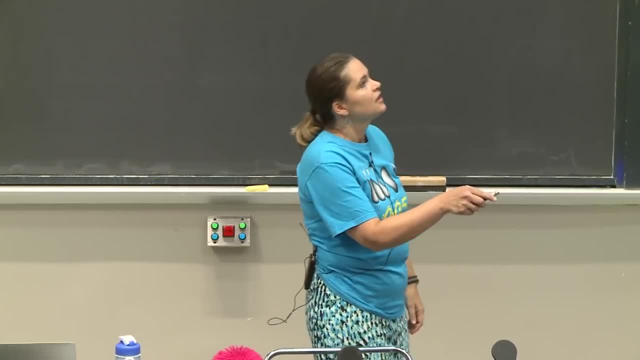 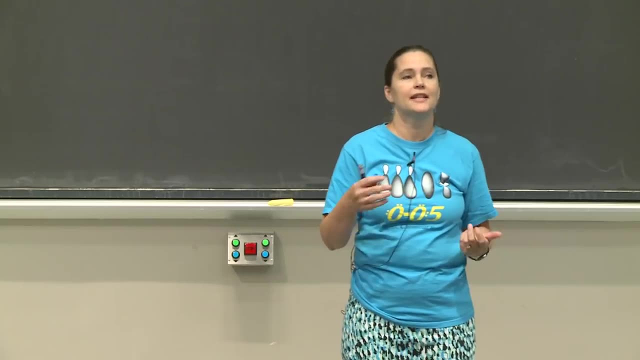 and one that's higher in energy, and that's the antibonding orbital. So that is not what that means. A bond order of 0 means that you have equal numbers of electrons in your bonding and antibonding orbitals, So there's no net stabilization due to the formation. of these bonds. So here, bonding occurs when you bring together two atomic orbitals to make two molecular orbitals that are both of lower energy. No, Every time you make the two orbitals, one is lower in energy and one is higher than energy. 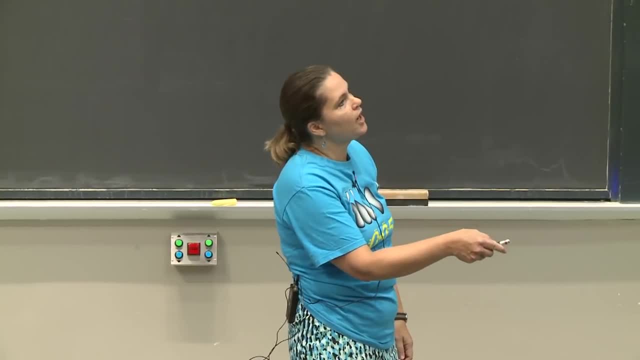 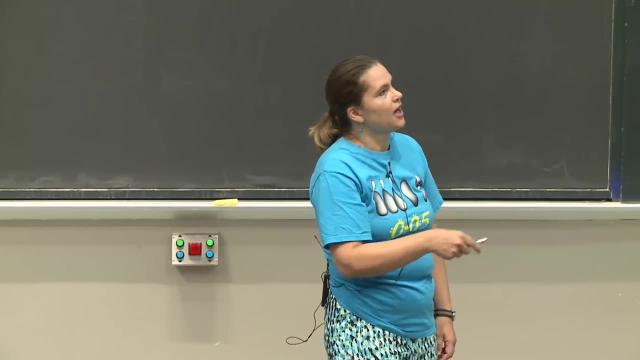 You can't make two that are both lower in energy, And a bond order of 1 means constructive interference, So you can think about this as one binding orbital or one binding orbital, where the interference is generated at one bonding orbital. That's not what a bond order of 1 is. And again. every time you generate a bonding orbital, you generate an antibonding orbital, And 1 means that you have twice as many electrons in your bonding orbitals as antibonding orbitals, because the formula is half the number of bonding. 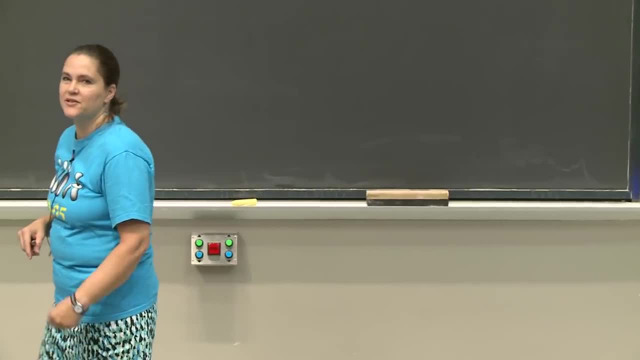 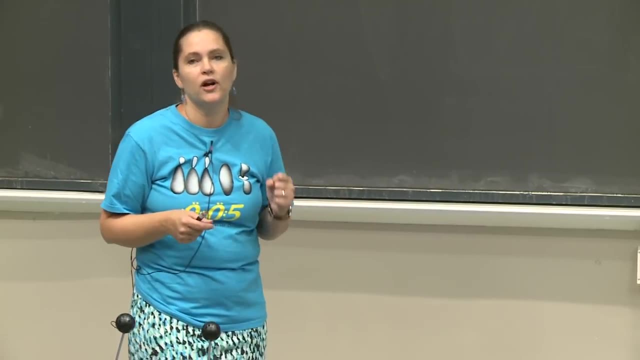 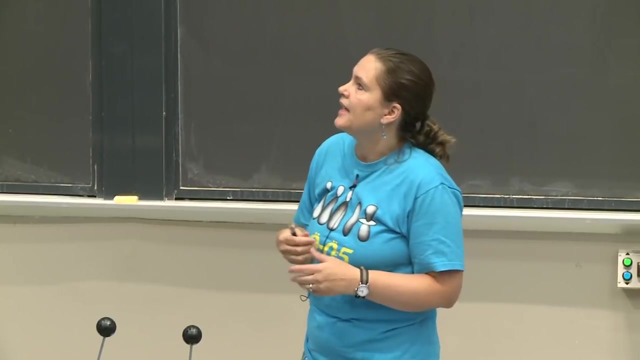 minus antibonding, But that's good, And it's important to remember that sigma orbitals are bond axis. All right, so we had these diagrams for boron and carbon just talking about the interactions of the px and py, And so we had forgotten about our pz. 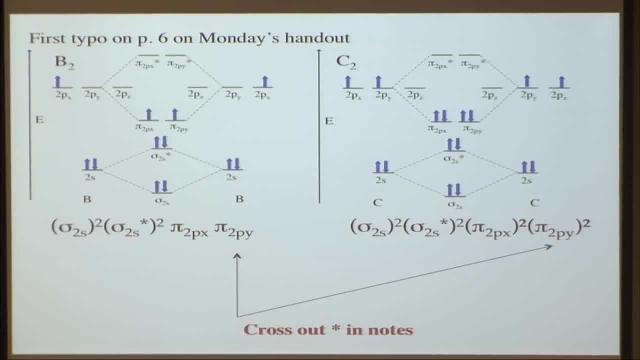 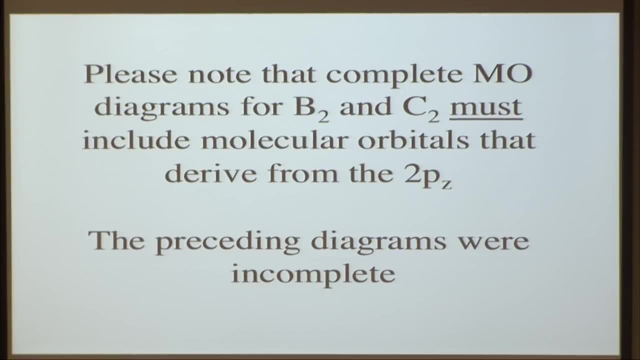 And you can't do that on a test to get into trouble. So I'm always telling people, for these two handouts you must include the molecular orbitals that were derived from p to z. So on a test you need to put them, even if they're empty. 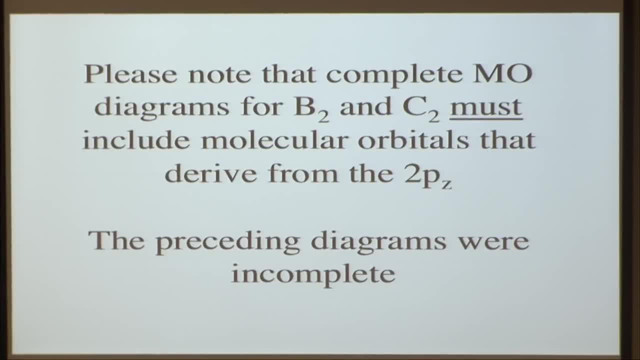 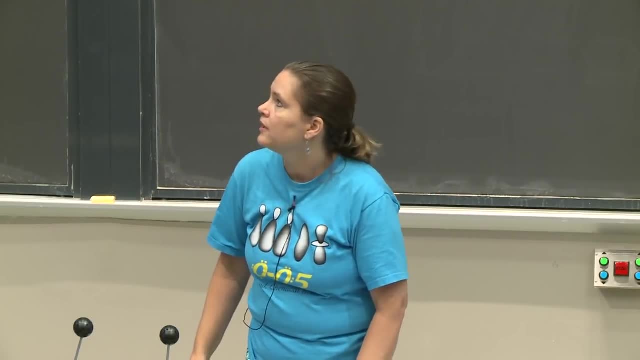 even if they don't have anything in them, they need to be part of your molecular orbital diagram. We didn't have them in the diagram because we hadn't talked about them yet, So now we're going to talk about them. So two pz orbitals. 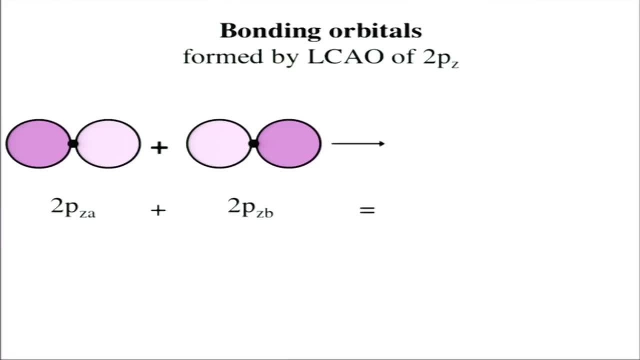 Again, this is on Monday's handout. You have this linear combination of atomic orbitals, So now, and all our p orbitals. they all look the same as each other, They're just different in orientation. You have one along x, one along y. 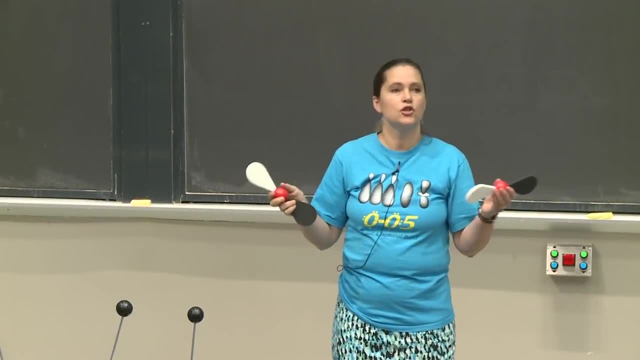 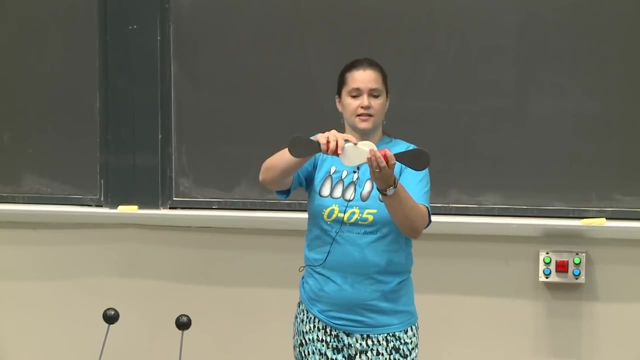 one along z, But they're the same. So now we're going to bring our two pz orbitals together And we're going to do it along the bonding axis. So we've defined this as the bonding axis in the class. So we'll bring them together. 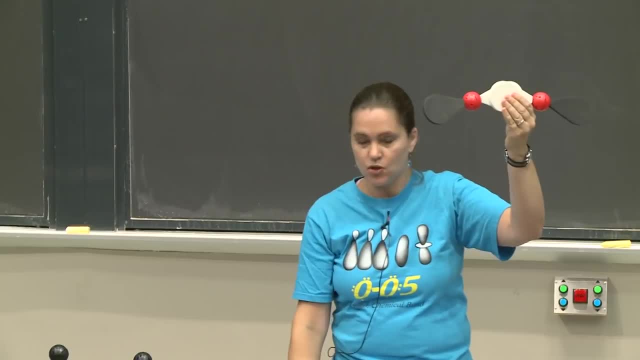 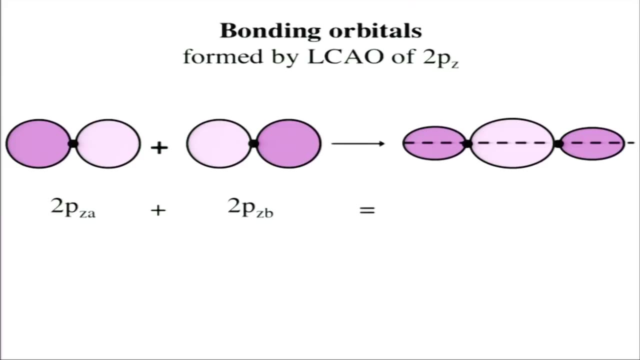 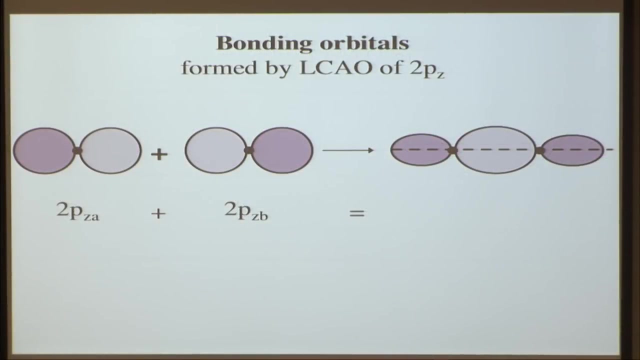 And there'll be constructive interference with our bonding orbitals. There's always constructive interference that generates bonding orbitals, And so we're going to create an enhanced amplitude as the wave functions come together, And it's going to be cylindrically symmetric. 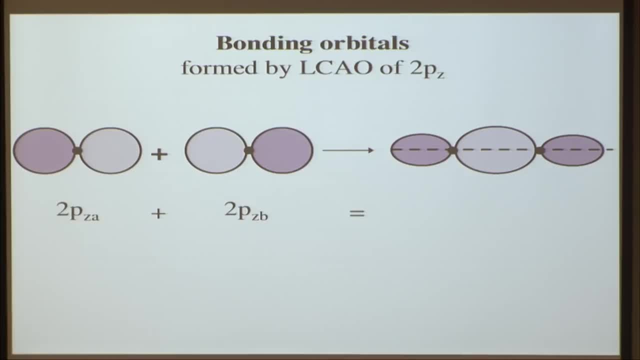 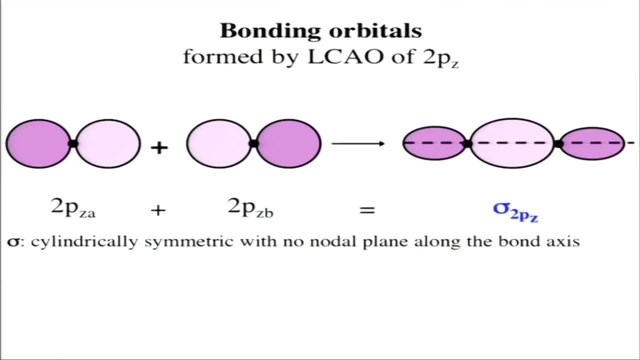 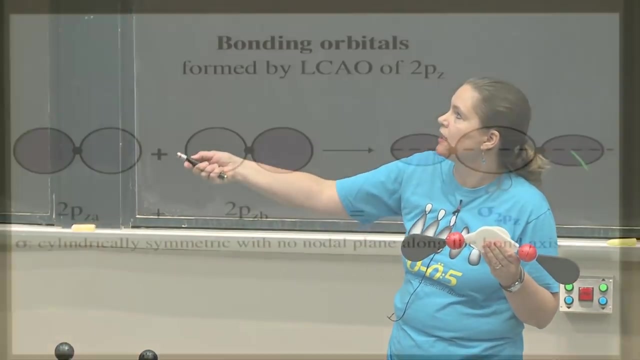 So what type of orbital do you think this is going to be Sigma or pi? It'll be sigma because it's cylindrically symmetric, So we do not have any bonding plane along the bond axis And it's symmetric around And we have enhanced probability density. 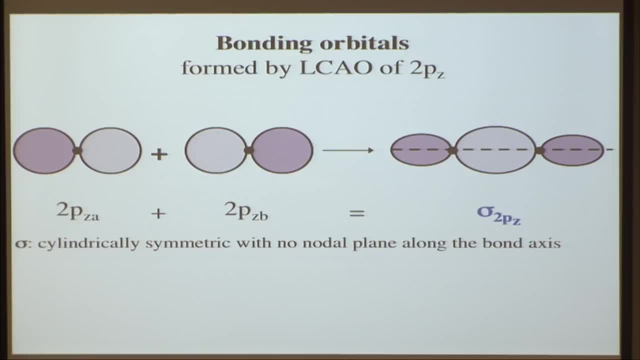 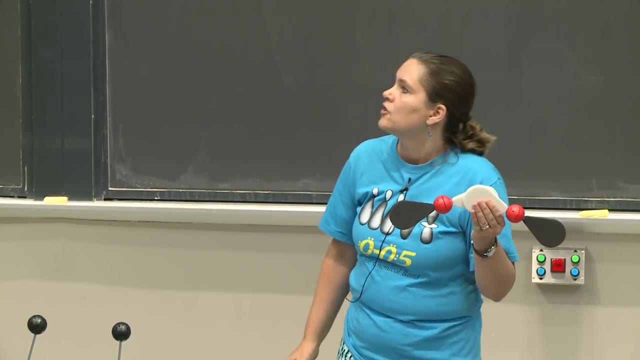 And we have enhanced probability density. And we have enhanced probability density And we have the wave function squared, enhanced probability of having an electron between the two nuclei, And so this is a sigma 2pz, So p orbitals can form sigma molecular orbitals. 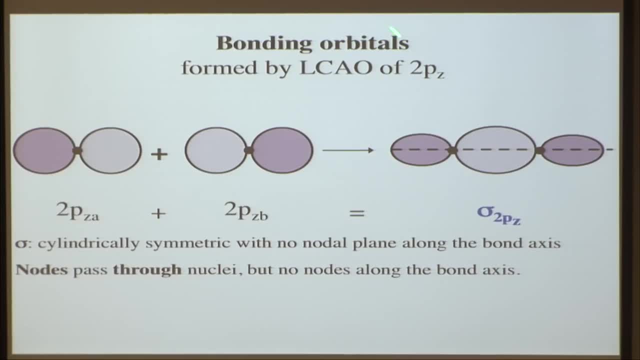 So we do have nodes passing through our nuclei. Here are our nuclei again. We do have them. They were here before in our p orbitals. There's a nodal plane in our p orbitals But we do not have them. We do not have, in this case, a node along the bond axis. 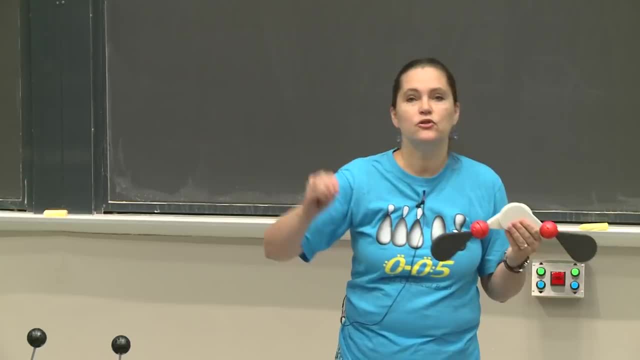 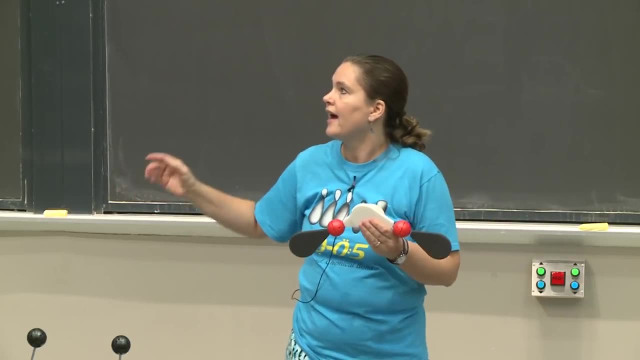 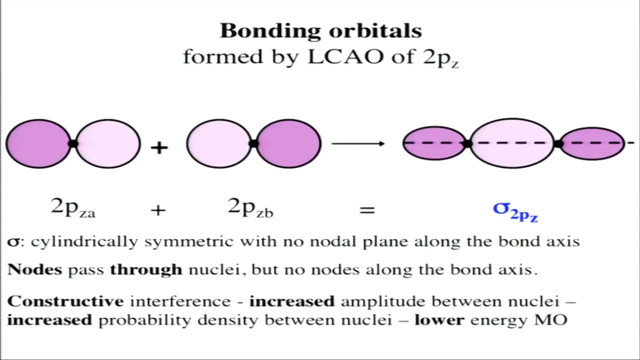 So that is our bonding. So whenever you generate a bonding orbital which is going to be lower in energy, we're going to have our increased amplitude between the nuclei again our increased probability density and therefore lower energy. So whenever you have constructive interference, 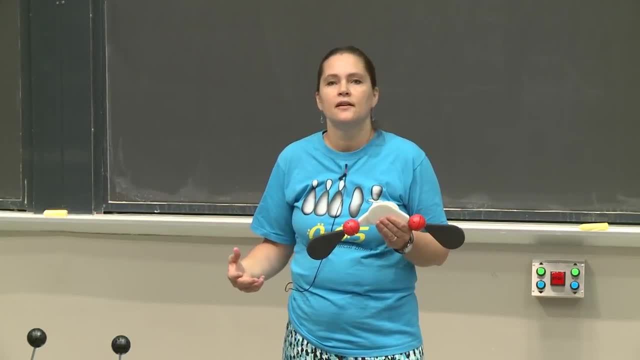 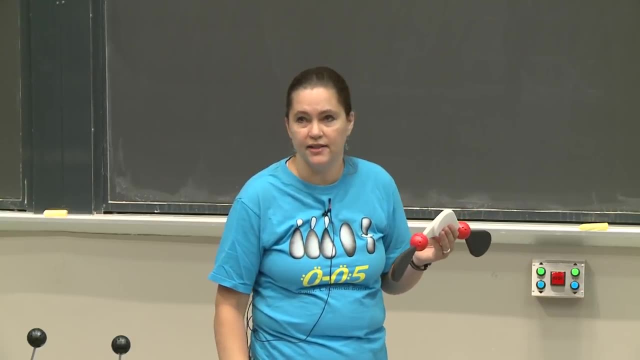 generating a molecular orbital of lower energy. you've got to create something of higher energy. That's just how life works. So we also are going to have antibonding orbitals, which are generated by destructive interference, And again these orbitals can be thought about as wave functions. 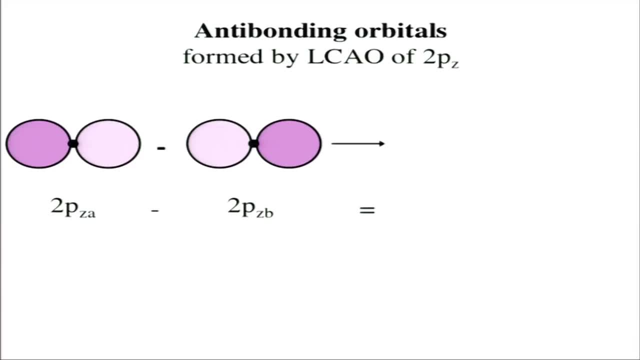 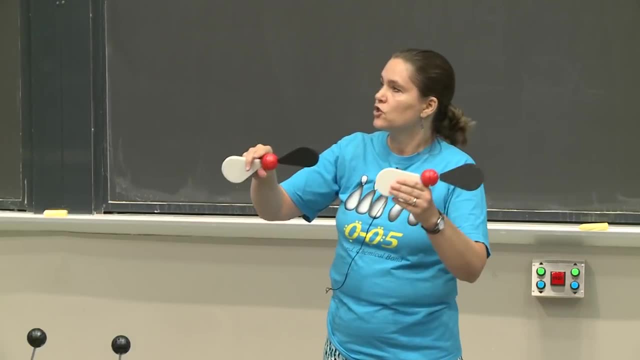 And a property of waves is that they constructively interfere and destructively interfere. So now we can subtract our two orbitals, which you're going to switch the sign and have. they're going to be out of phase. So they're going to be out of phase. 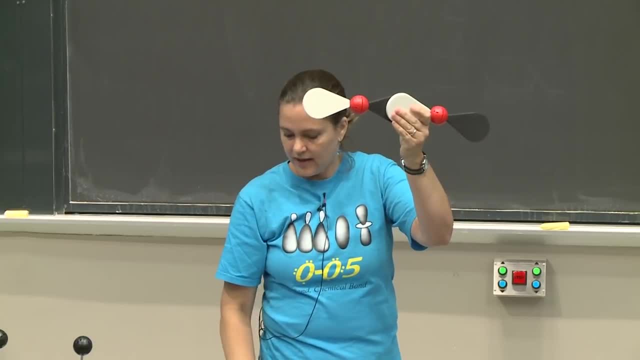 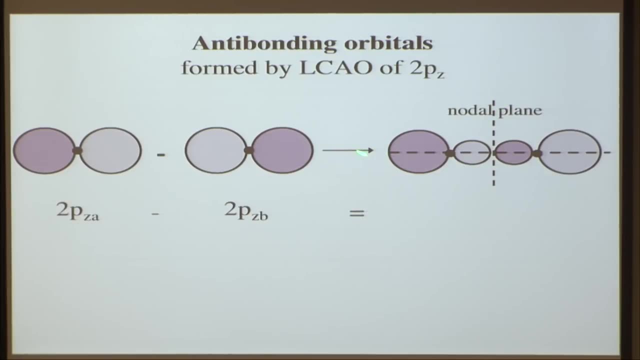 So they'll destructively interfere And that's going to look like this. So now you're going to generate a nodal plane between the two nuclei, but it's still symmetric around the bond axis. So this is a sigma 2pz star. 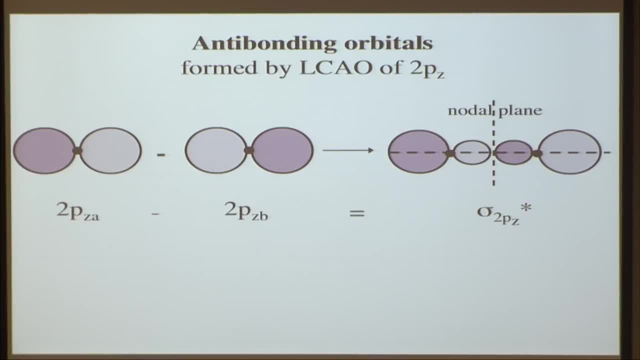 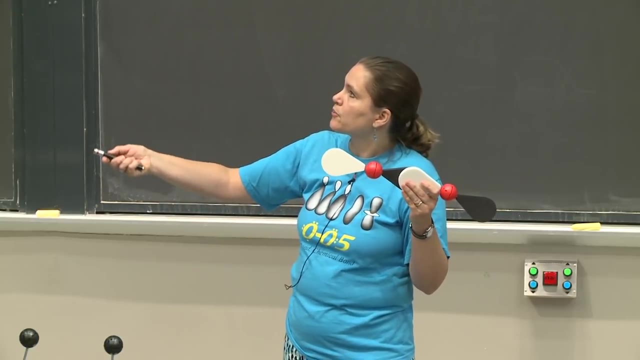 So it's an antibonding orbital. So again it's sigma. So it's still cylindrically symmetrical with no nodal plane along that bond axis. But you do have a new nodal plane that's generated, So nodes pass again through the nuclei. 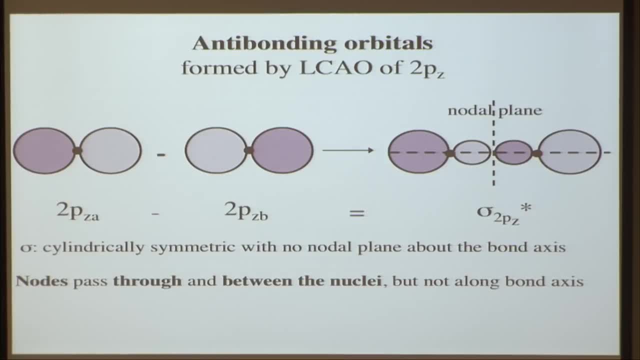 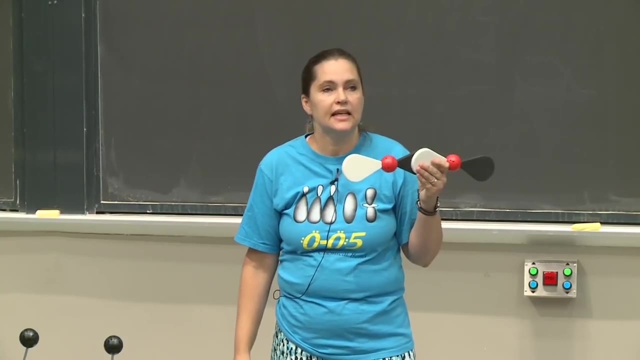 but also now between these two orbitals. So we have a new nodal plane that's generated, that's between these nuclei And that's a result of destructive interference, Generates that nodal plane. You have decreased probability density for an electron being found there. 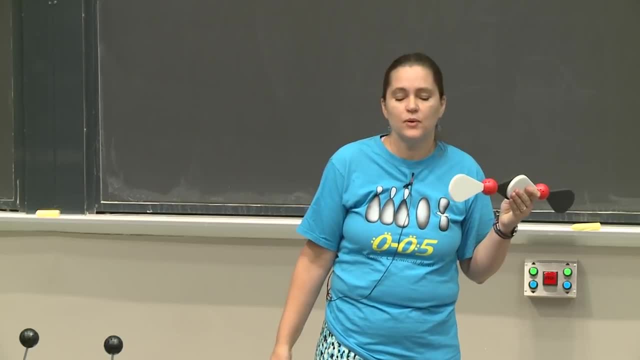 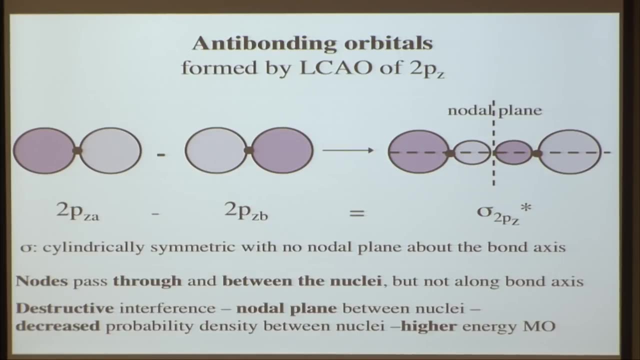 And so So that poor electron's kind of shut out of that sweet spot. The electrons like to be between those two nuclei, where they have the two positive charges of the nuclei And then their little negative charge, And they can sit right there and be very happy in a low energy. 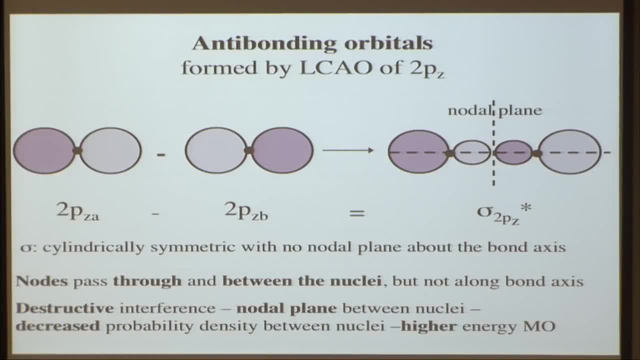 state. But here there's really lower probability density, lower likelihood. the electron will be found here And that generates a molecular orbital that's antibonding or higher in energy. All right, so now we have to go back to our M1.. 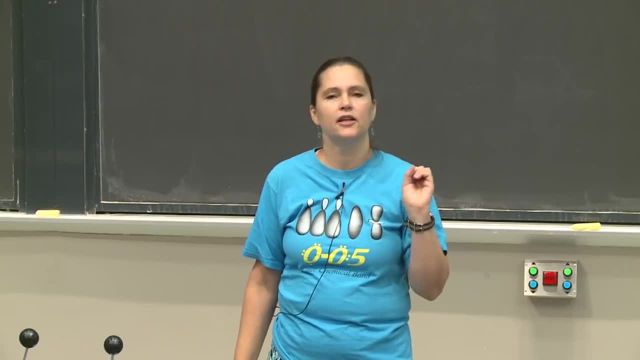 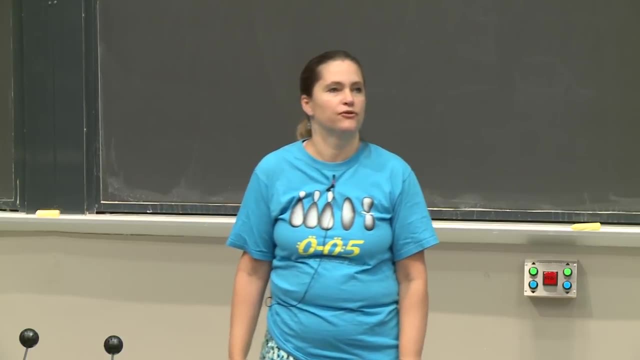 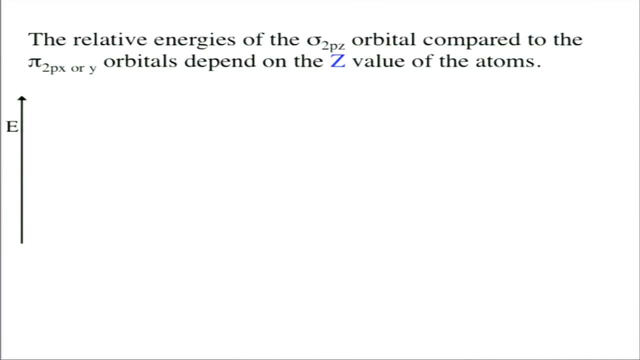 M0 diagrams and figure out where to put these new molecular orbitals onto our nice diagrams. And it's not as simple as it was before, Because where we put these new sigma 2pz molecular orbitals depends on what z is, So it depends on the value of z. So if z is less than the magic number of 8, then We have our pi, 2px and 2py orbitals are lower in energy than our sigma 2pz molecular orbital, But if we are equal to or greater than 8,. 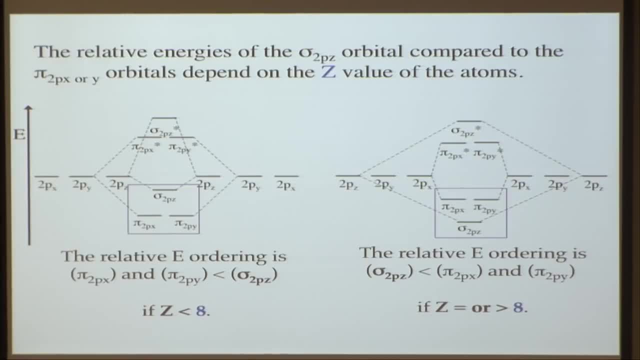 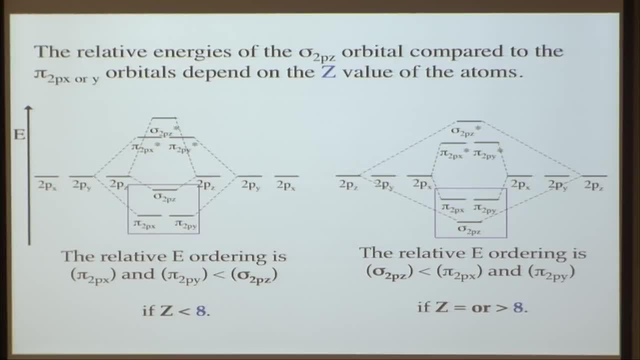 And 2py And 2py. Now, if z is greater than 8, pi is first, its lower in energy as you go up your energy scale. And if z is equal to or greater than 8, pi is second. 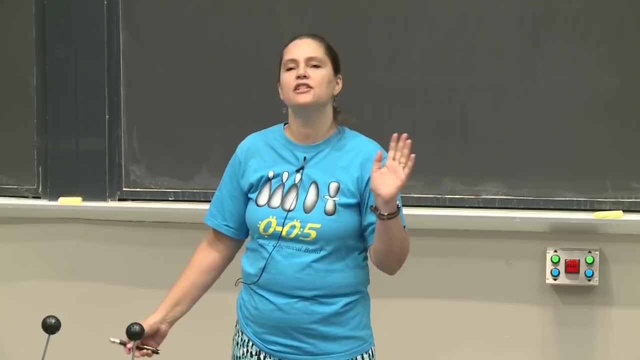 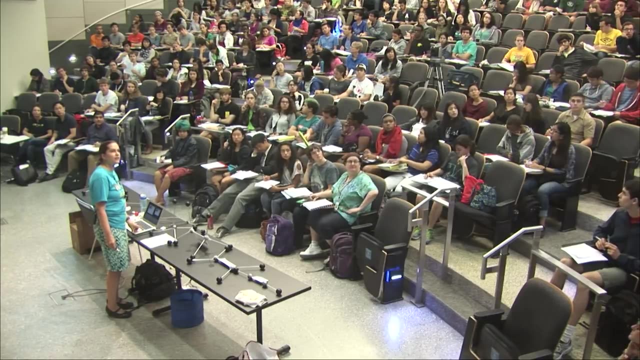 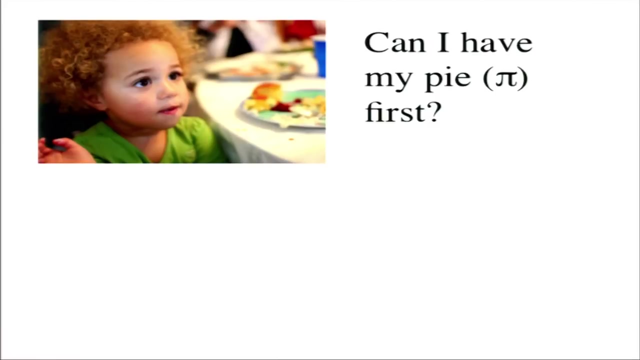 And sigma is first. So how are you going to remember this? There could be many different ways one could remember it, But I'll tell you how I remember it. And I sort of my life revolves around my daughter and my dog have the question: can I eat pi first? 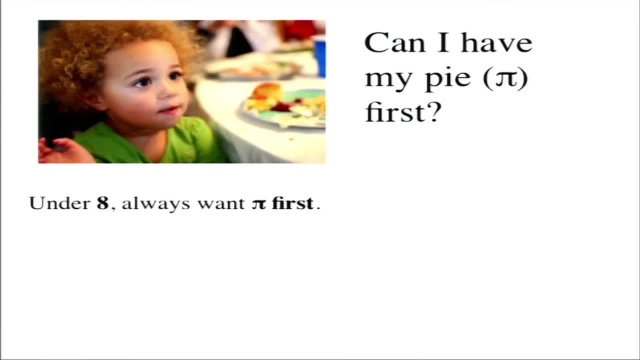 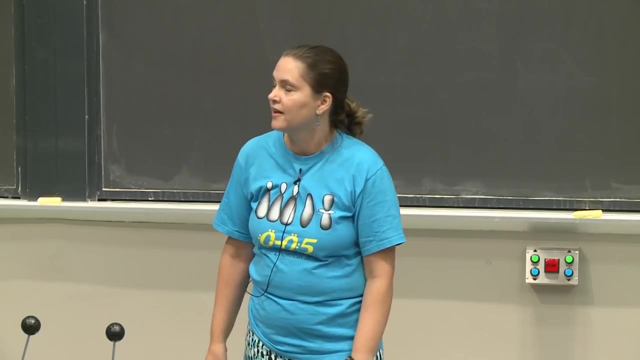 So if you are under the age of 8, you always want your pi first. So if z is less than 8, pi comes first. Pi is lower in energy and sigma is higher. However, when you mature to the grand age of 9,, say, or 10,, 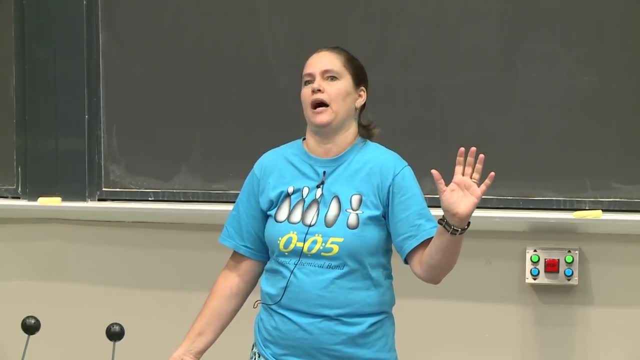 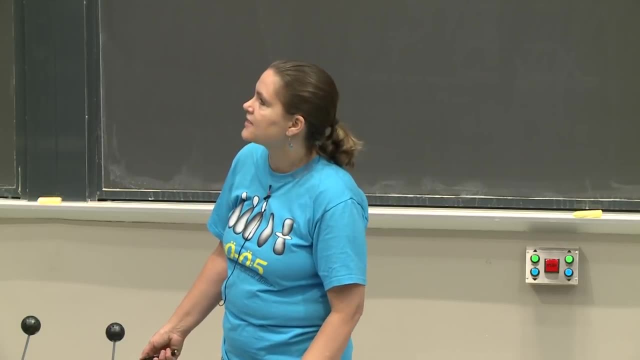 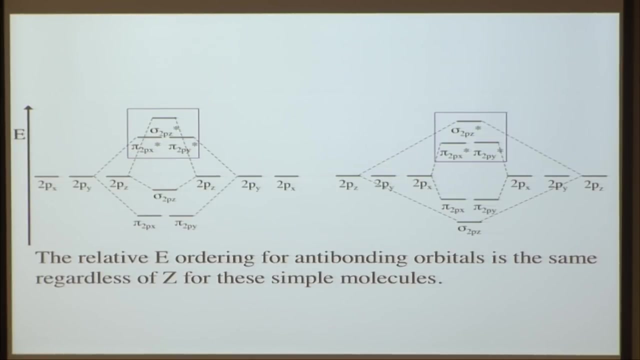 if you were a kid, 10 is like the oldest you can possibly imagine- being very mature And you can eat your Thanksgiving dinner and wait for pi. So that is how I would remember it. Under 8, pi is first Equal to 8 or greater, you can wait till after dinner. 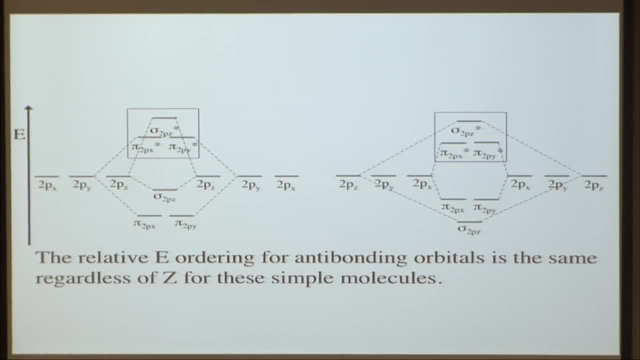 to have your pi. Pi comes second. Note that the ordering of the antibonding orbitals is the same. So all you have to remember is down here It depends on z: Is pi first or is pi second. So let's take a look at an example. 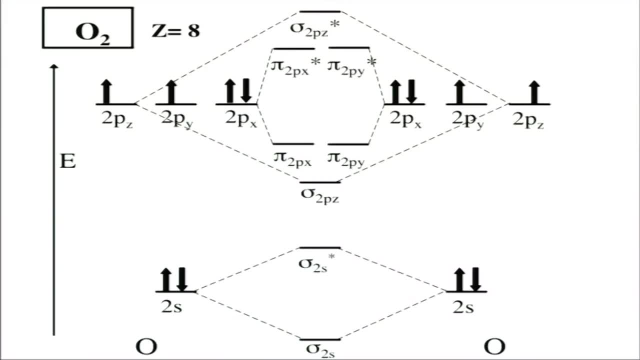 Let's look at our friend molecular oxygen that has a z equal to 8.. So oxygen is at the old mature age of 8. And so it's going to have its sigma 2pz first. It can wait for its pi orbitals until later. 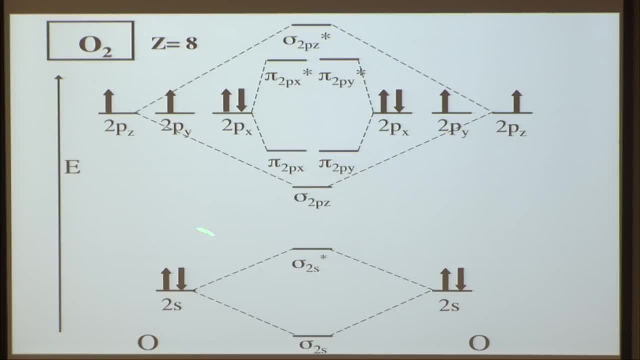 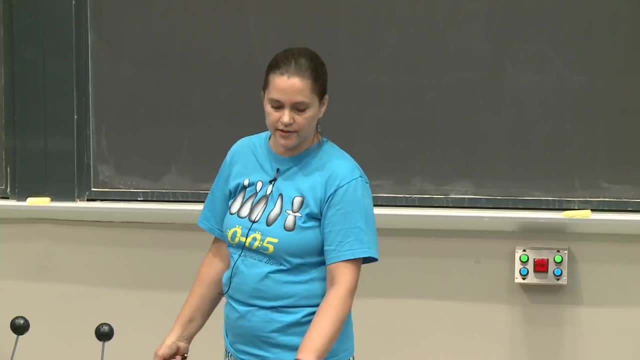 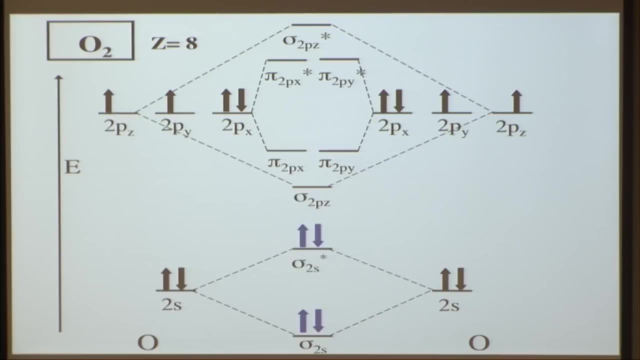 So let's start putting in our electrons So we have each oxygen And each oxygen making up molecular oxygen or O2, brings two 2s orbitals to the Thanksgiving dinner table And two of them go down in energy into the bonding sigma. 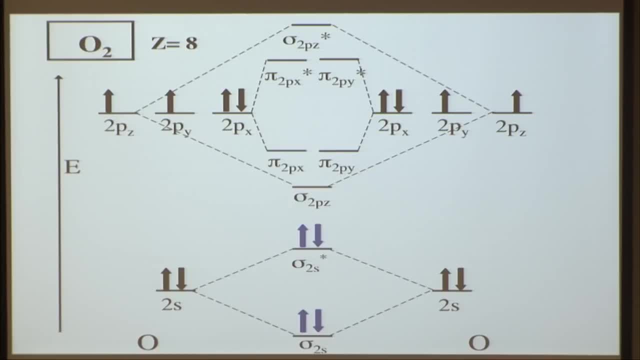 2s orbital And two go into our antibonding sigma star 2s orbital. Now we have four electrons in our pz orbitals, in our atomic pz orbitals, So we need to put all of those in, So we always start with the lowest energy orbital. 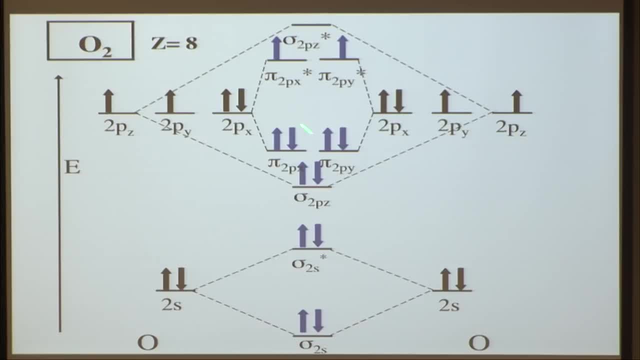 So we'll put two in there, Then we'll go up. We have two more here. two more here. We'll put them in singly, with their spins parallel, And then we'll pair them up in the lowest energy orbitals, And then we have two more left. 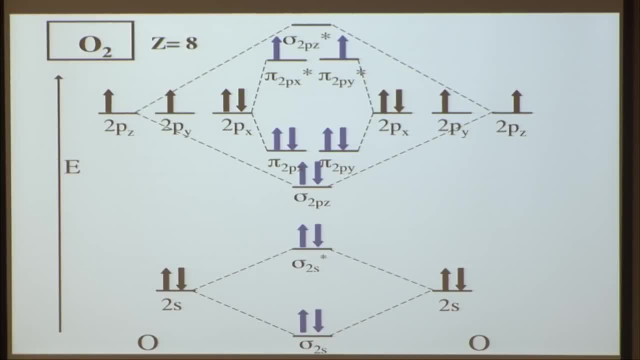 So we're going to have to put those up in our antibonding orbitals So they go into pi 2px and pi 2py star, And then we're going to put those orbitals up here. All right, So now we can calculate the bond order for oxygen. 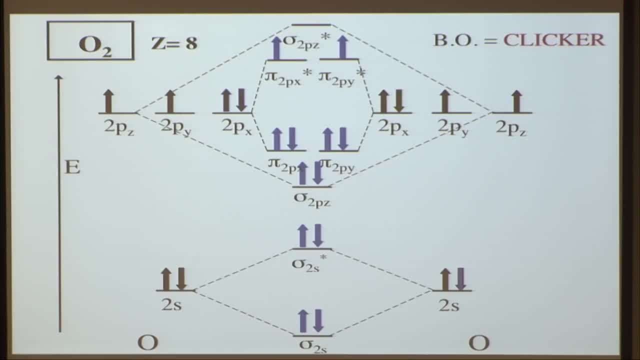 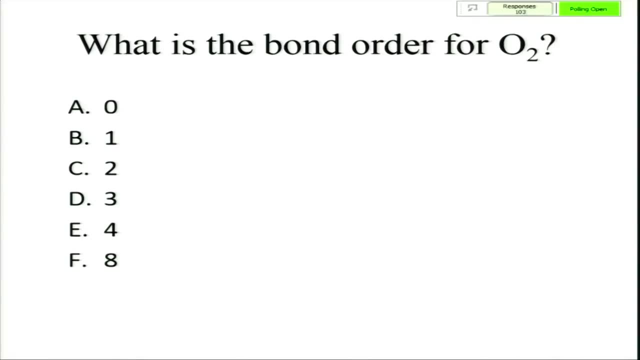 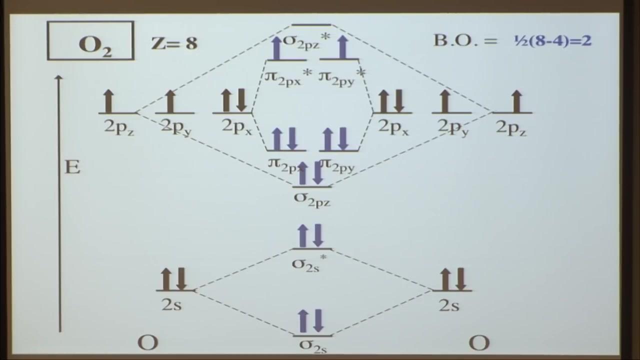 And that's a clicker question. All right, Let's just take 10 more seconds, All right. So let's take a look over here. So bond order Again is half the number of bonding electrons minus the number of antibonding electrons. 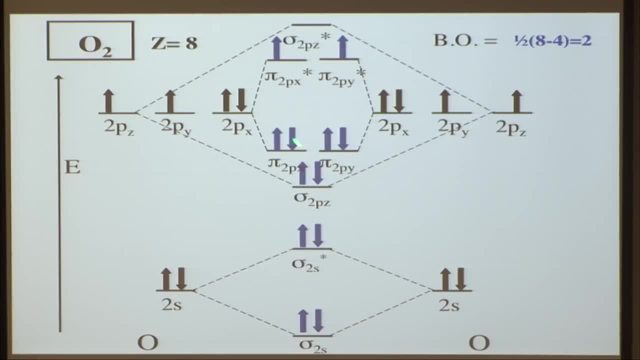 And we have eight bonding: 1,, 2,, 3,, 4,, 5,, 6,, 7,, 8.. And we have four antibonding: 1,, 2,, 3,, 4.. So that gives us a bond order of 2.. 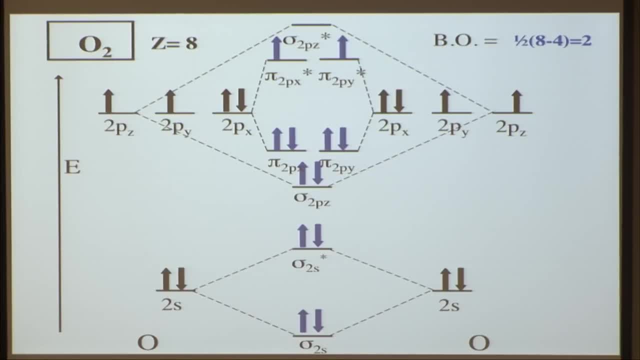 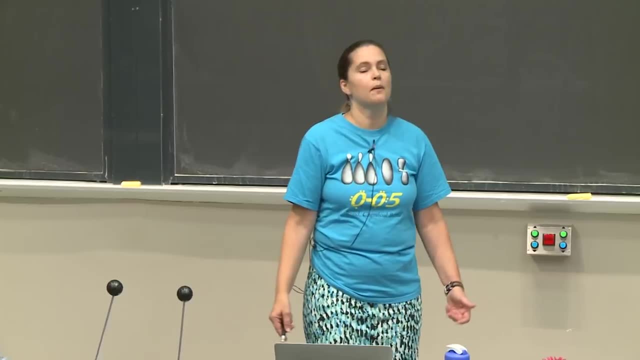 And the bond order equation is one that you do have to memorize, That will not be given to you on an exam. And with a bond order of 2, we have again a pretty big number for dissociation energy. Again, that's the energy you have to put into a bond. 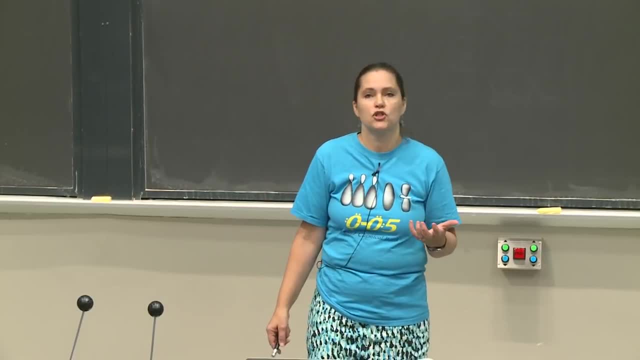 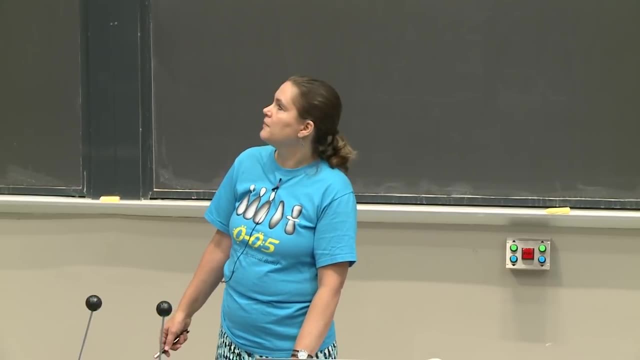 to break it, to dissociate it, And that means it's a pretty strong bond. if it's a big number, If you need a lot of energy, that's a strong bond. Another thing that you can see from this diagram is that O2 is a biradical. 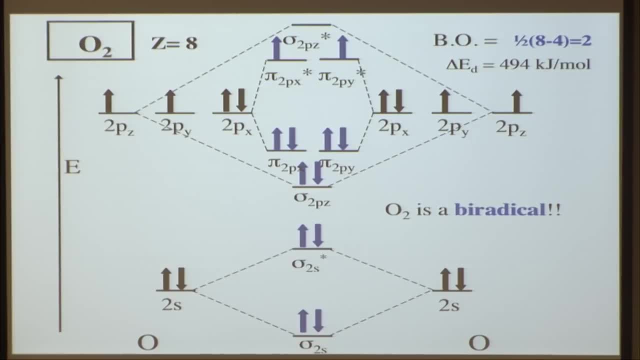 It has two lone pair electrons, so two unpaired electrons, which also makes it paramagnetic or attracted to a magnetic field. So whenever you have unpaired electrons you will have a paramagnetic species And diamagnetic means they're all paired. 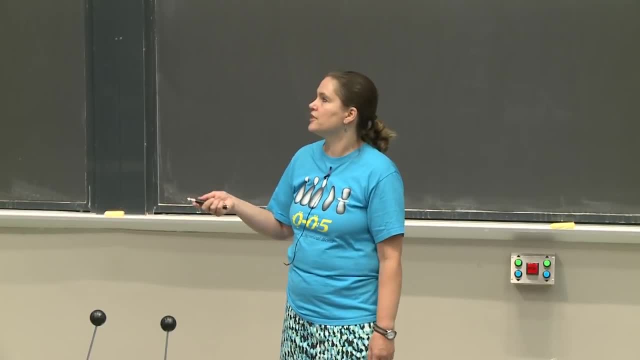 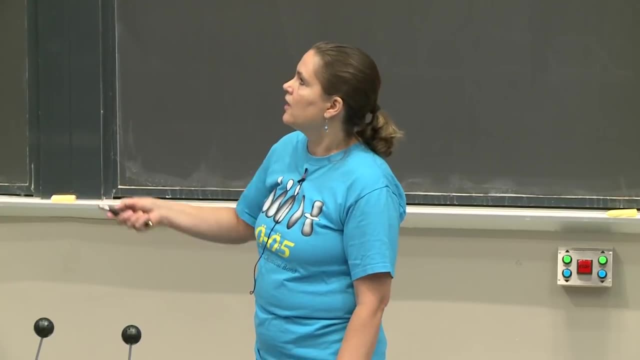 And so there's some questions on problem sets and on exams, so you need to know the definitions of those. All right, so we talked about this when we were doing Lewis structures, if you recall, And we drew a beautiful Lewis structure of molecular oxygen. 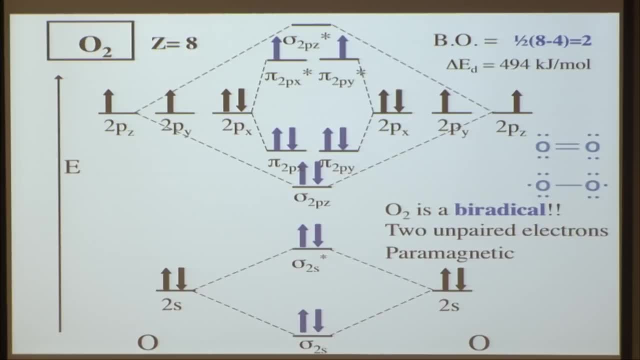 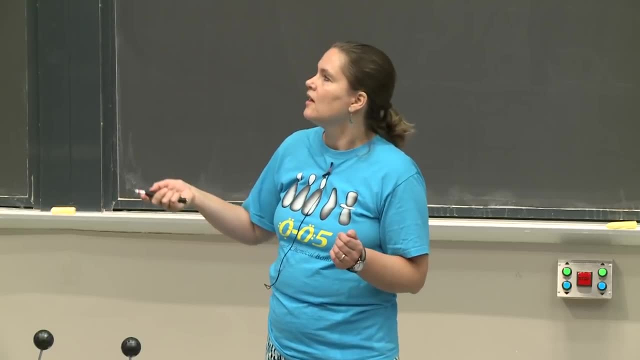 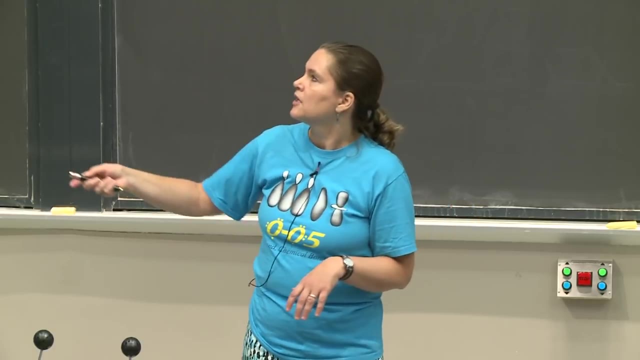 that had two lone pairs on each oxygen and a double bond. But I told you that that was not really a complete description of molecular oxygen. that molecular oxygen was actually a biradical. But you would not get a hint of that from the Lewis structure. 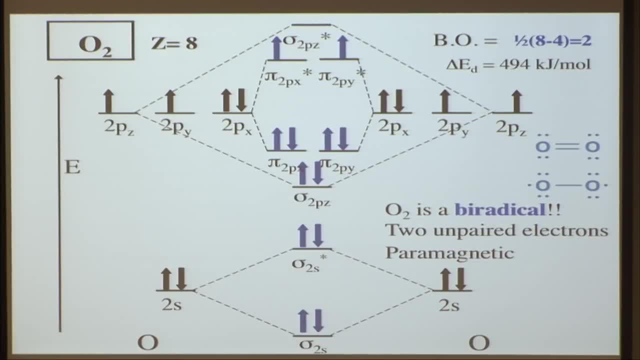 So if you draw the Lewis structure as a biradical, then you have a single electron here and a single electron there and a single bond. But we also see the bond order is two. So this one does describe It's- the biradical nature, but doesn't really. 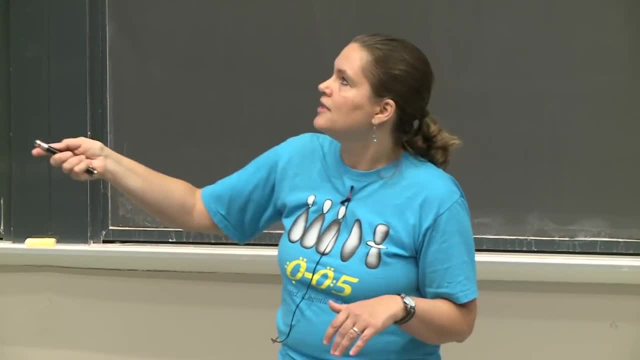 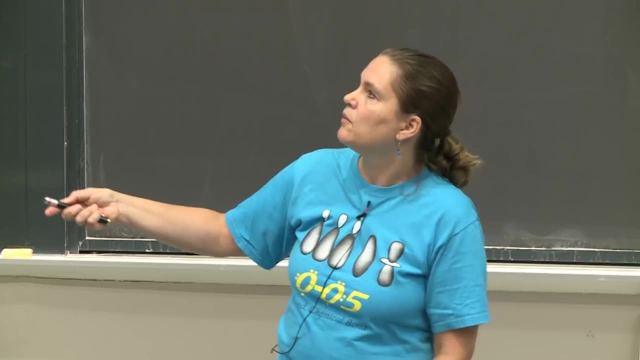 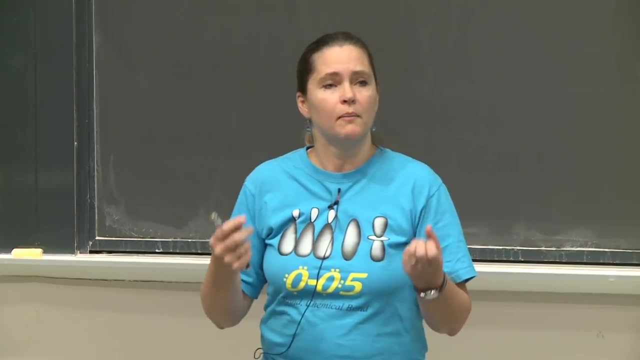 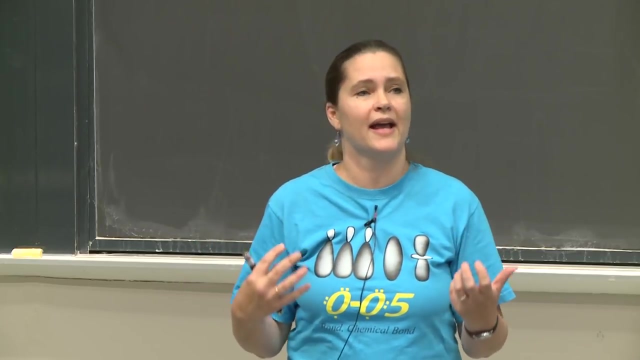 describe that double bond character that it has. So neither of these Lewis structures really completely describe molecular oxygen And we need a molecular orbital diagram to really help us understand the properties of molecular oxygen. that it's pretty strong bond between it. It has double bond character but it also is very reactive. 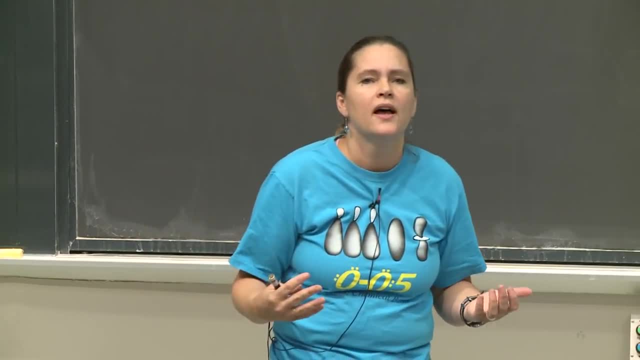 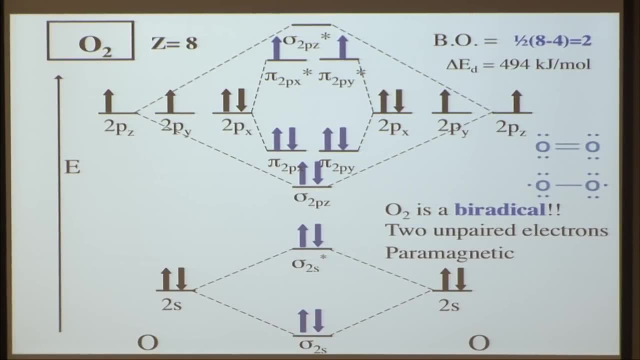 It's a biradical, So this is just a. It's a bizarre molecule And really that is why this diagram right here really tells us why our life, our planet, is what it is right here That describes it. It's because of oxygen that we have the life forms that we did. 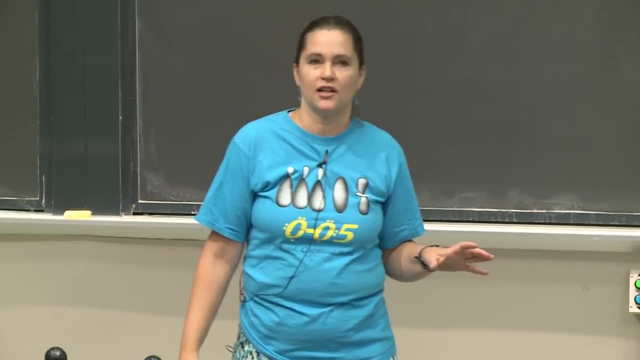 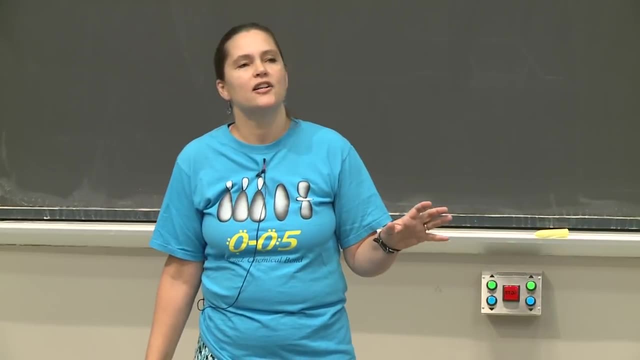 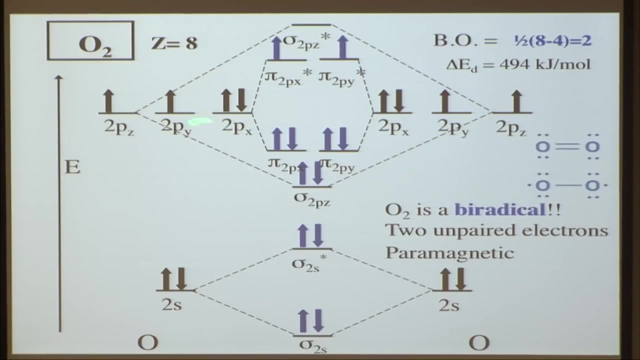 Life was very different on this planet before molecular oxygen came about. You did have microbes that lived anaerobically without oxygen, But when oxygen came, everything changed. And so here this. if you say, can you explain life to me? 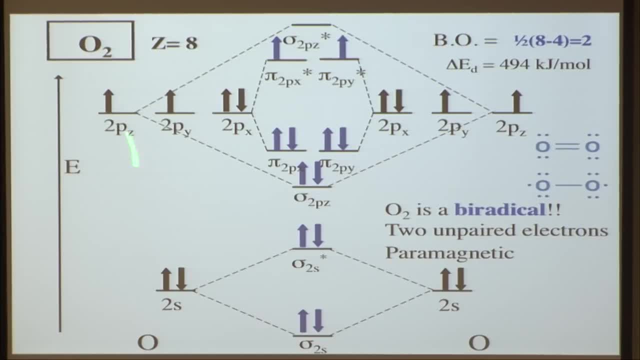 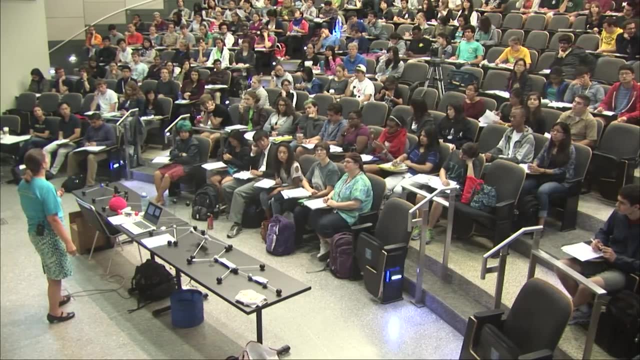 You can draw this And there it is. This explains life as we know it, because life as we know it exists because of this crazy molecule that is O2.. Nothing else really like it. It is an amazing molecule that allows us to live. 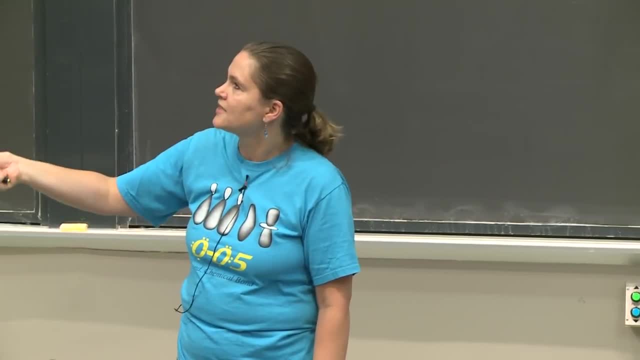 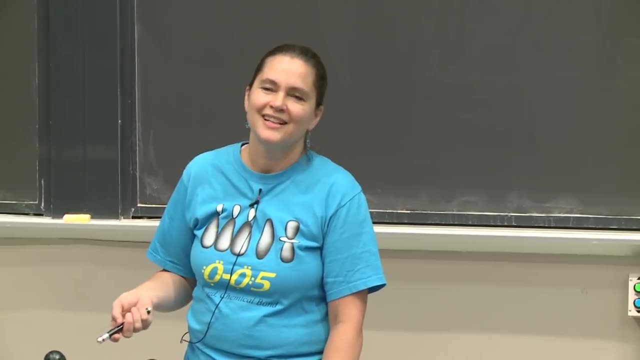 So there you go, So you don't learn anything in chemistry. This diagram: I just explained life as we know it to you right there. All right, We also. it's not just, there's a few other elements that, yeah, are pretty important. 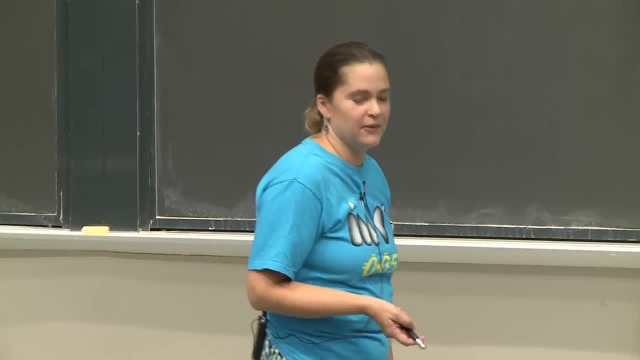 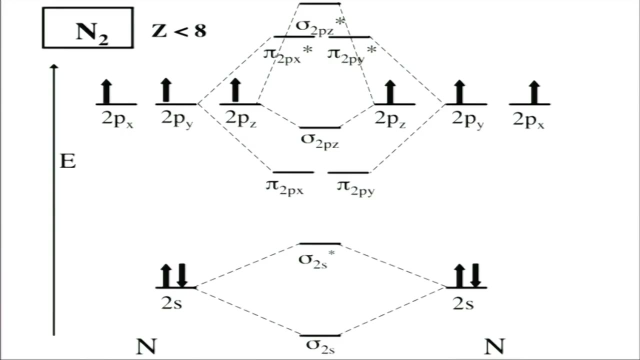 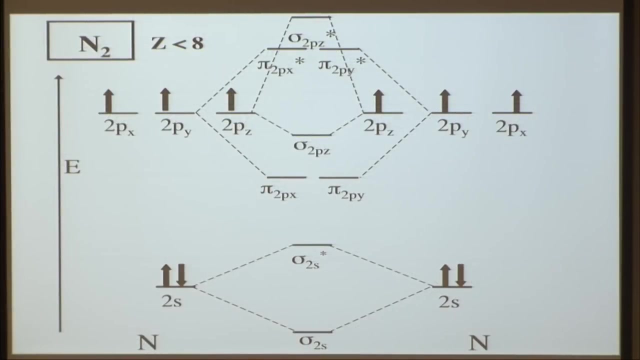 And one of them is nitrogen. We wouldn't really be much anywhere without nitrogen either. Oxygen is no. nitrogen is pretty special too. OK, This also helps. Maybe these two molecular orbital diagrams really sum up life as we know it. All right, so let's look at molecular nitrogen N2.. 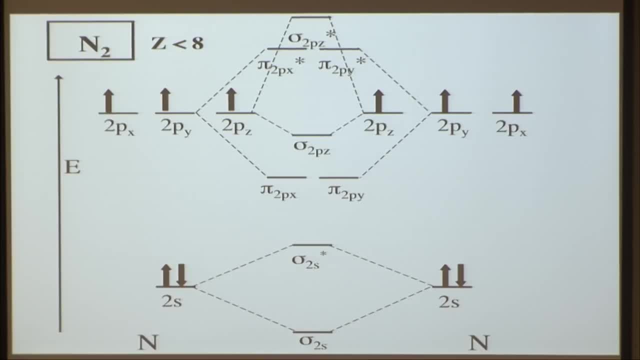 So we have two electrons in our 2s orbitals, So we're going to bring them together. We're going to put two in the lower energy orbital, our sigma 2s, and two in our antibonding orbital, And then we have three in our p orbitals from this nitrogen. 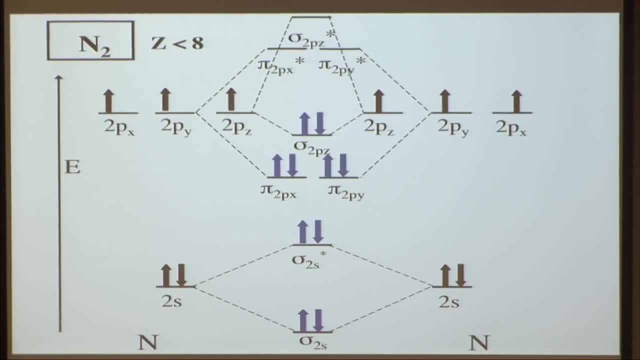 three electrons from this nitrogen, And so we'll put them down here. We'll put in two, three, four, five, six, So we didn't need to use any of these antibonding orbitals. And this is a z less than 8 case. 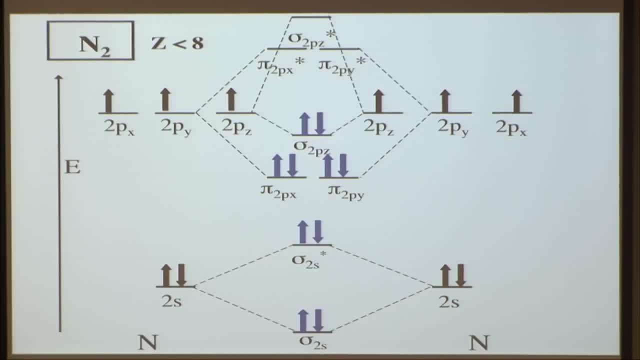 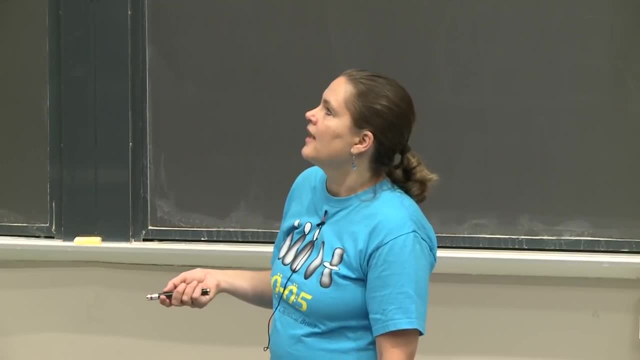 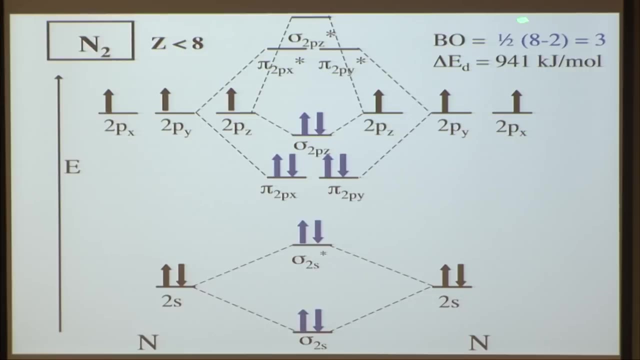 So here we have our positive. We'll put our p orbitals first, because it is z less than 8.. So let's look at the bond order here, And the bond order is half of 8,, 1,, 2,, 3,, 4,, 5,, 6,, 7,, 8,. 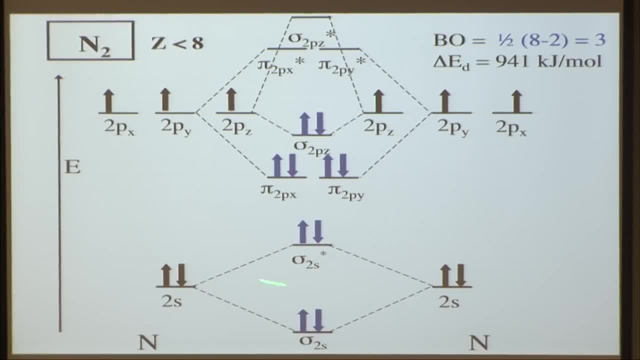 8 bonding electrons and just these two antibonding electrons. So a half of 8 minus 2 is 3. And you have a really big number for your dissociation energy: 945.. 41. This is a very stable molecule. 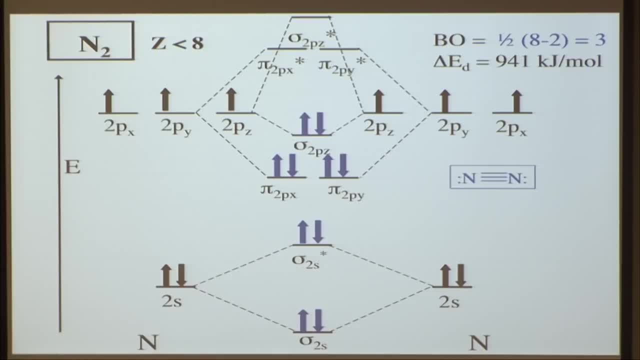 And you can draw the Lewis structure of this without much difficulty. This one works quite well And you get a triple bond and two lone pairs. So this would be a diamagnetic molecule: no unpaired electrons, no radicals here, But this is a crazy strong bond. 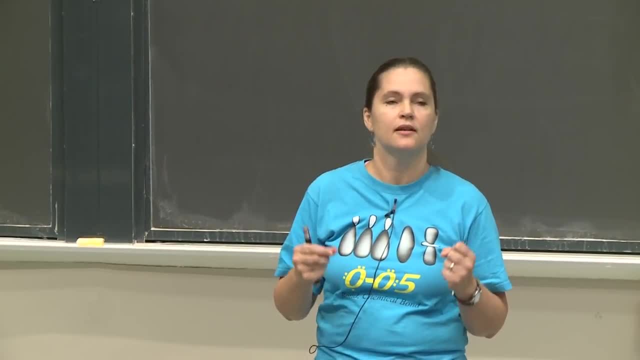 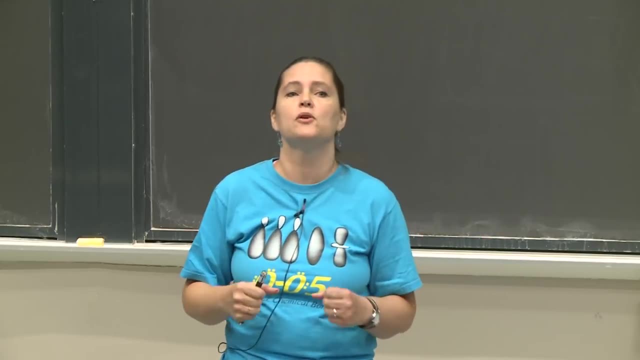 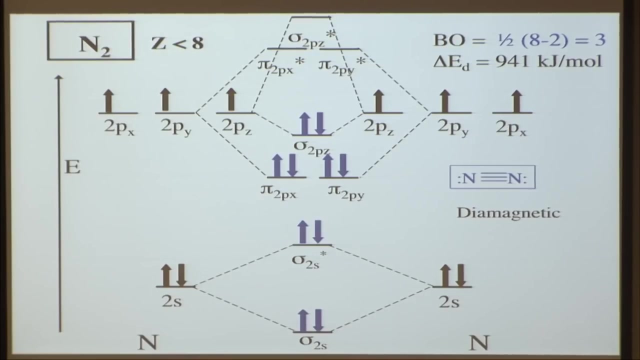 It's really hard to split nitrogen because of this triple bond, And molecular orbital theory tells you it should be a triple bond. It should be really, really strong interactions between these nitrogens, And so this is a very hard thing. We want to do this industrially and we'll. 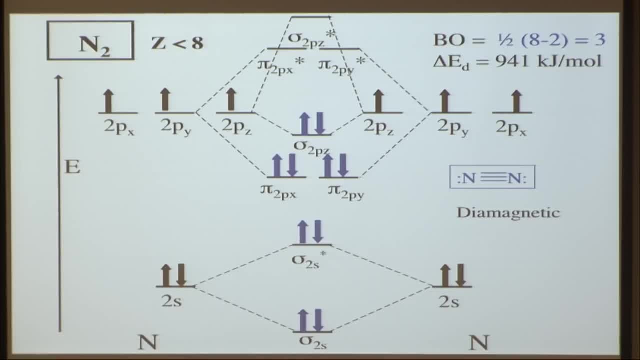 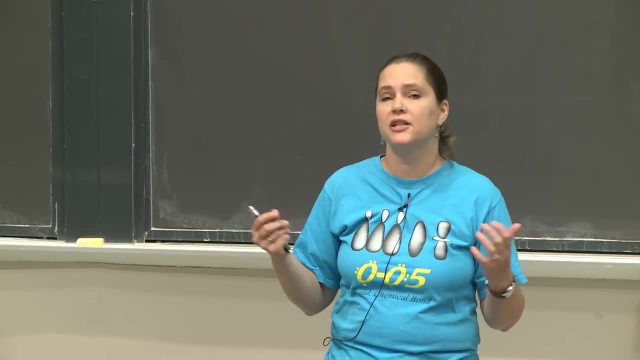 talk more about this. when we get to chemical equilibrium, How do you split the nitrogen bond? This is actually currently a big area of research: how you break that bond, because we need nitrogen for life, And so how do you split it? There's lots of nitrogen and two in the atmosphere, but we need